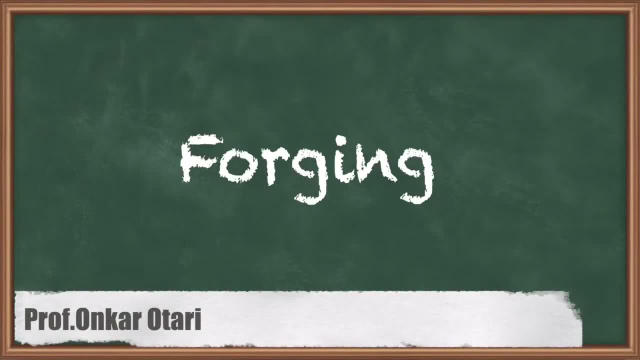 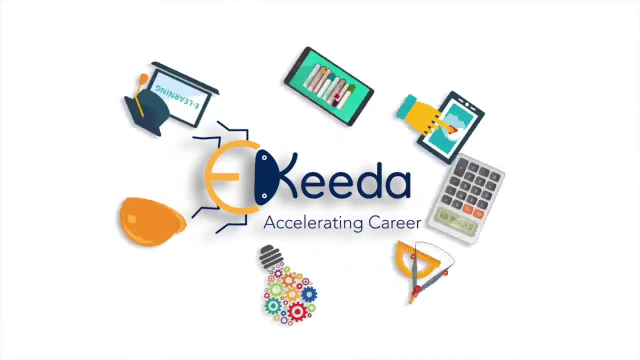 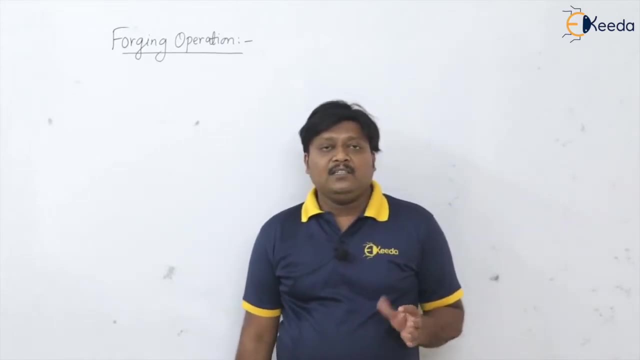 welcome students. now in this video we are going to see the next metal forming process, that is, the forging operation. so what is forging operation? so it is a process in which the material- material or metal- is heated and then the force is applied to manipulate the size and shape of the component. 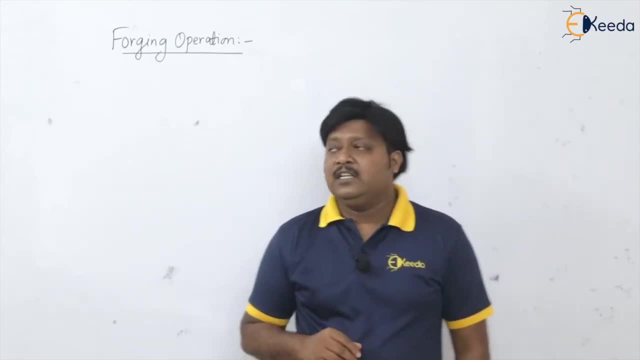 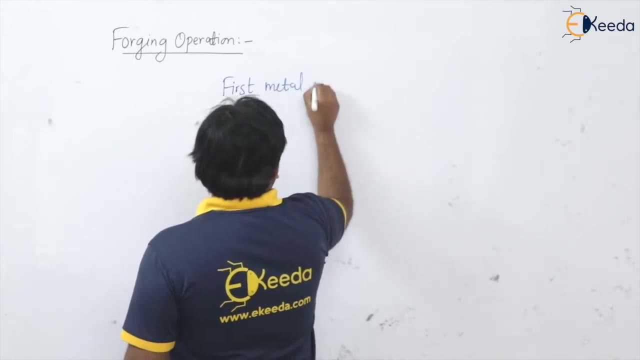 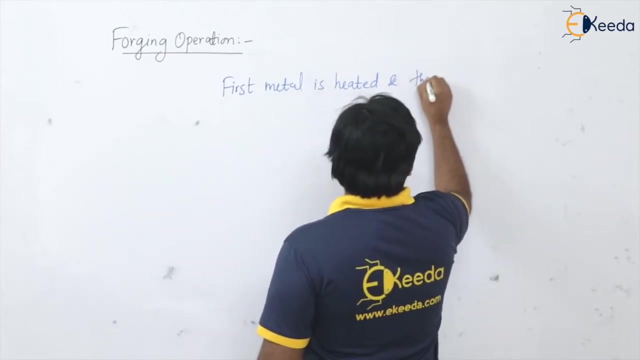 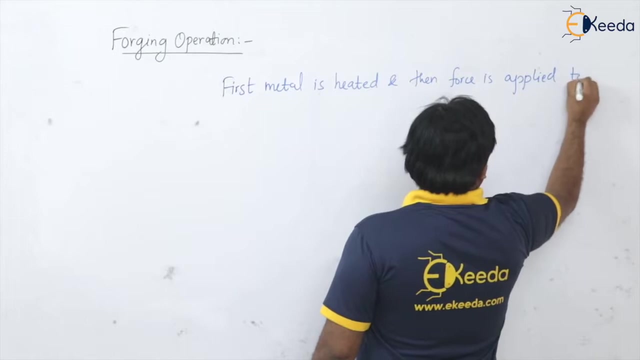 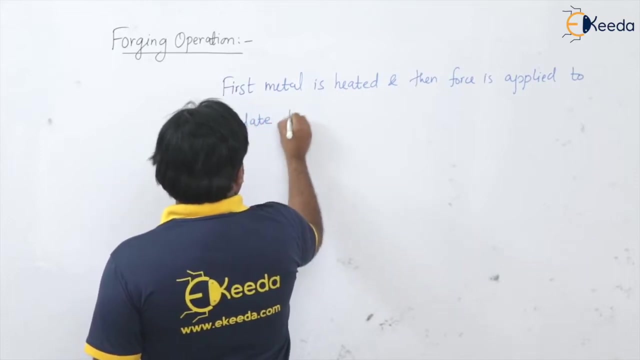 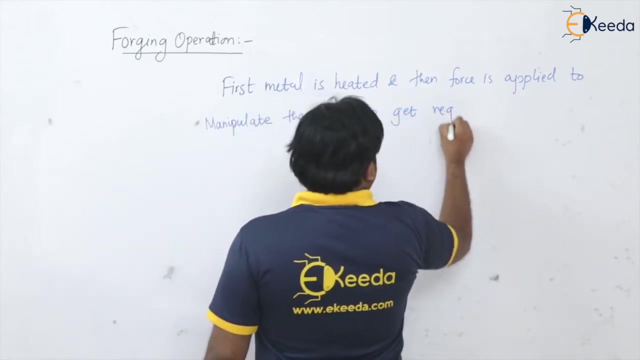 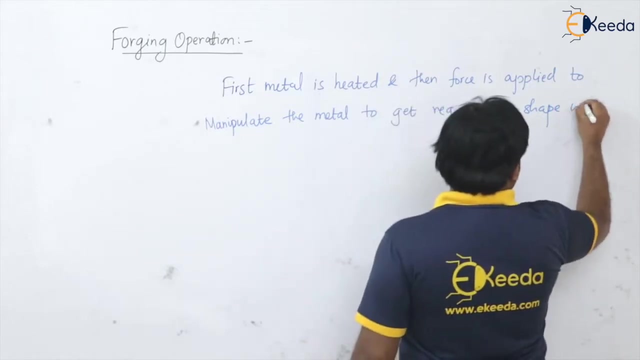 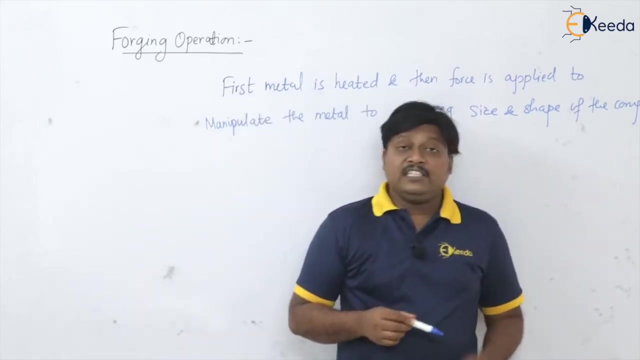 or that metal. this is the forging operation. so here, first we heat the metal, first metal is heated, and then force is applied to manipulate the metal to get required size and shape, or shape and size of the component. this is the forging operation. so, and the stresses induced here are of course the pure compressive. 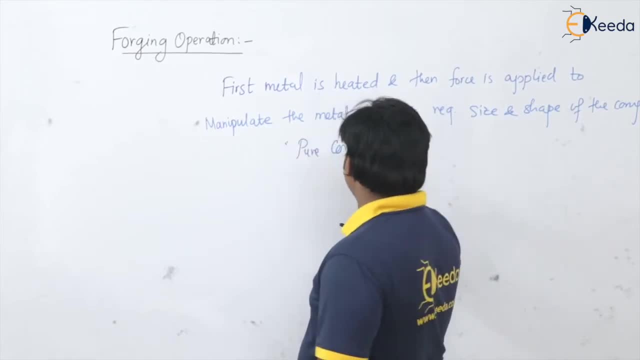 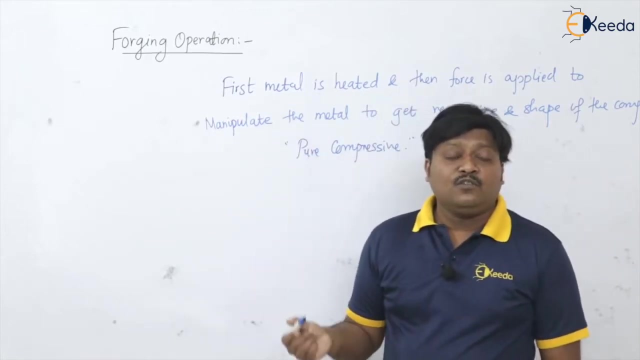 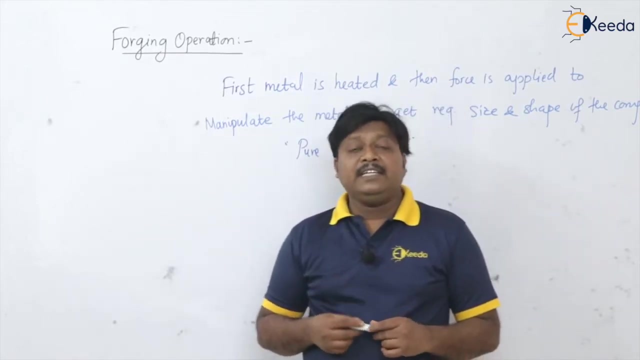 pure compressive stresses are going to induce into the material. see, the forging operation is one of the oldest metal forming process which is known to the mankind since the copper age. and this forging operation can we have the hot forging operation or sometimes we can use the cold forging operation also now very important characteristic. 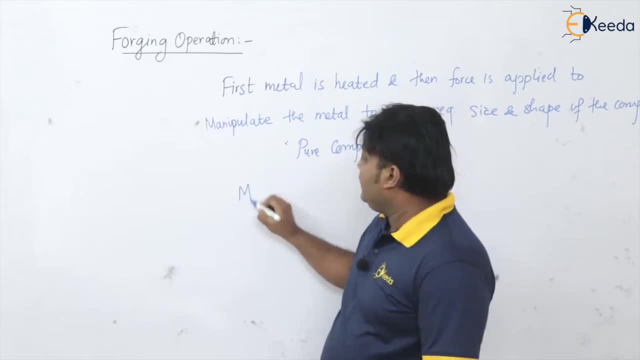 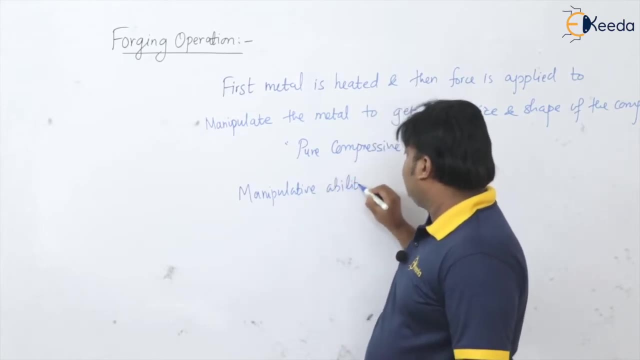 softening of thefry. reason also now very important characteristic or property of the forging operation, that the manipulative ability isn't IT. the manipulative ability also to control the grain flow and serait an important language. so ht at" At40 from이야 Grain Flow. 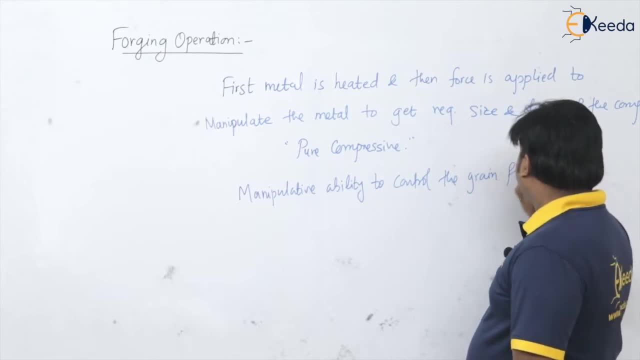 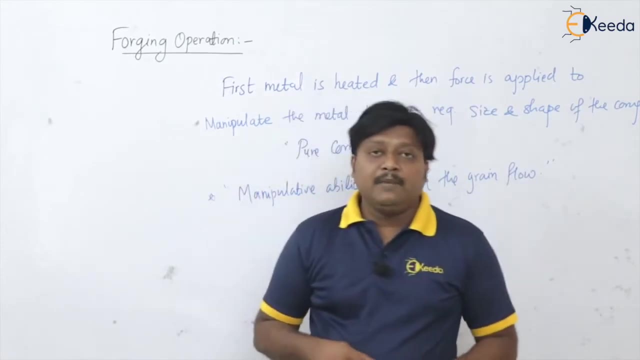 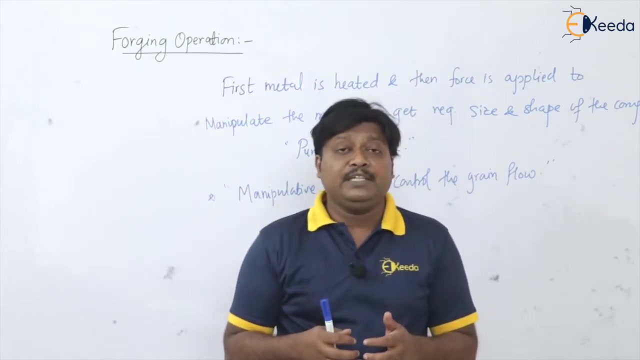 tofu To control, to control the grain flow, so thatconhungerI Know Alit important thing for the forging operation. please remember, because of this maneuverability, ability to control the grain flow, we can get the best mechanical property in the specified direction. that is very important. characteristic characteristics of the forging operation. 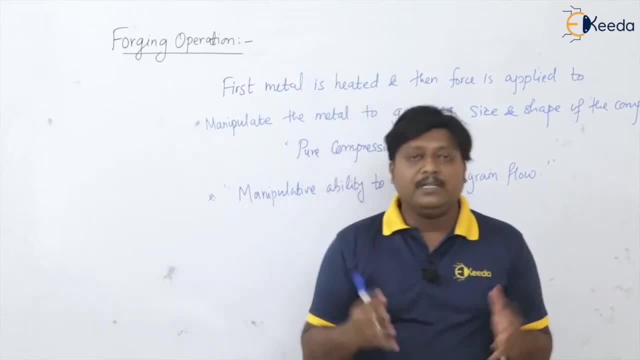 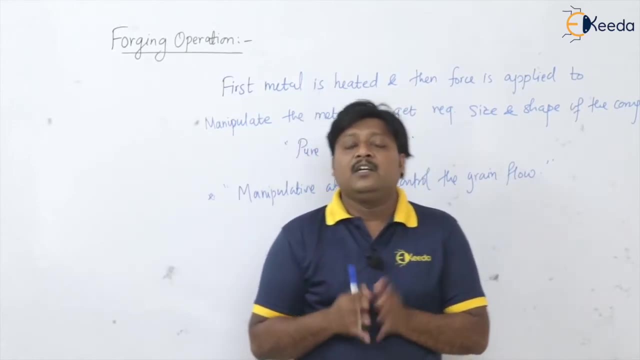 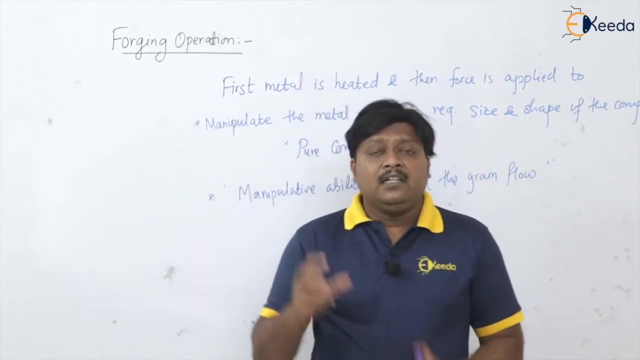 so required orientation of the grains can be possible. because of that, wherever and whatever good mechanical properties we want to impart in the product, we can easily get. now, as already we discussed in the beginning of this topic, that in all the metal forming processes- the say limitation of the all metal forming processes- that we can go for the uniform kind of shapes in all these. 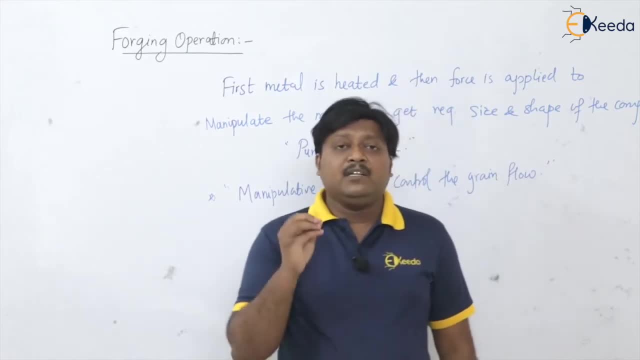 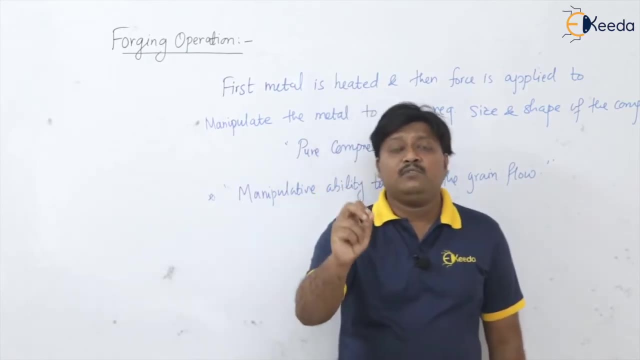 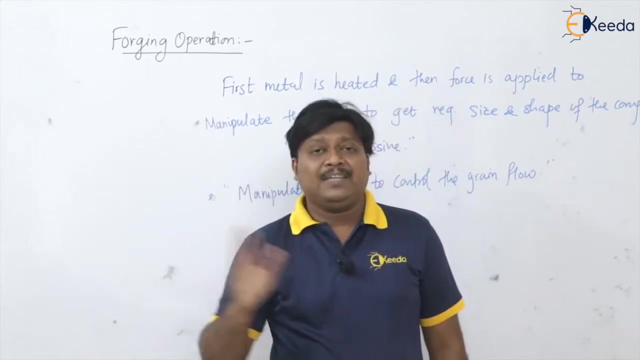 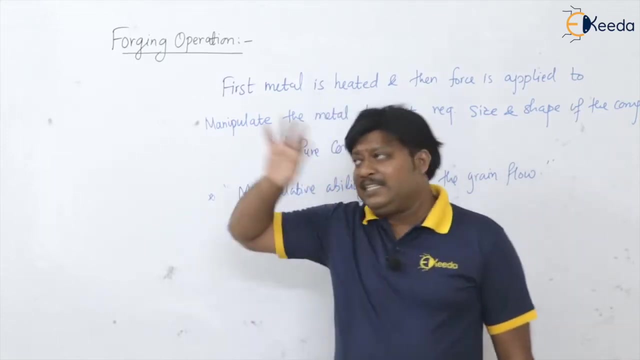 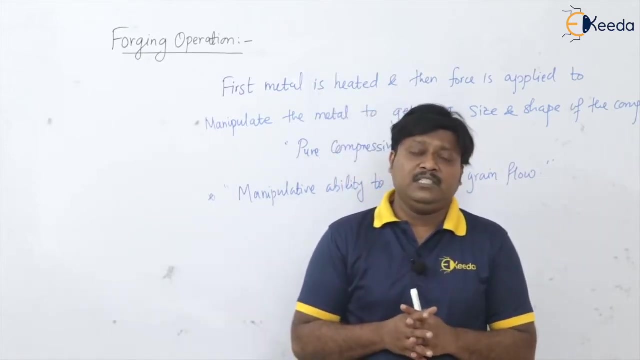 processes. but see, forging is only the metal forming process, where approximately 每種 phenomena of an all jo-no shapes of the product. but the limitation of the forging itself is that we require the huge amount of forces and the power consumption. remember, if you require, the higher. 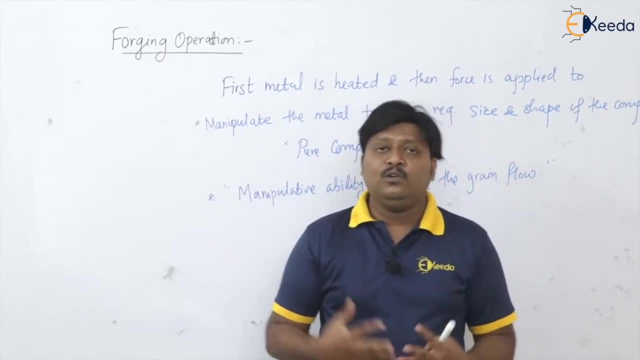 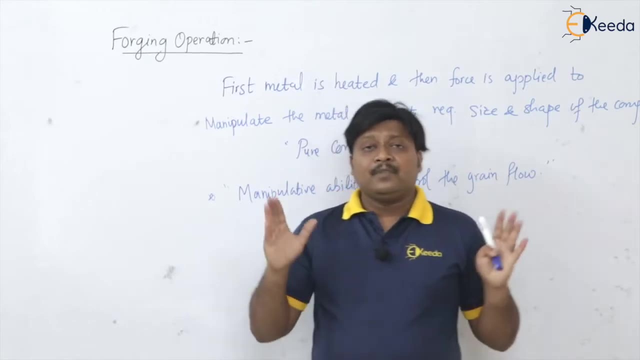 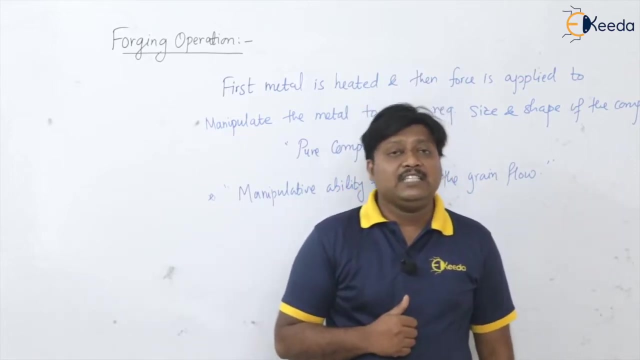 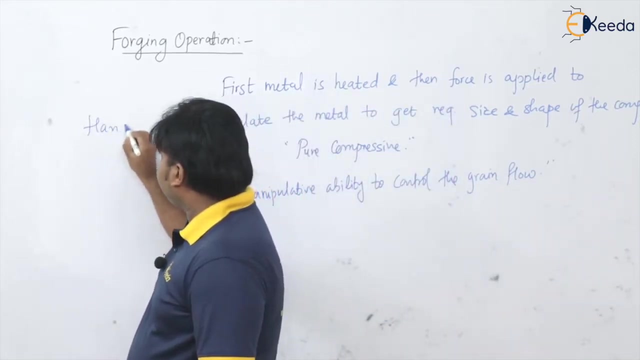 amount of forces. to produce that higher amount of strength of forces or load, we need to have the that much amount of power consumption. so the force and power consumption is quite high in the forging operation. okay, so let us see what are the classification of forging. so forging is basically classified into, say, the hand forging. there are two types we can. 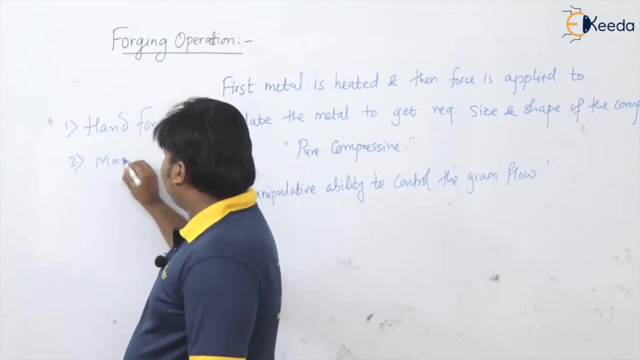 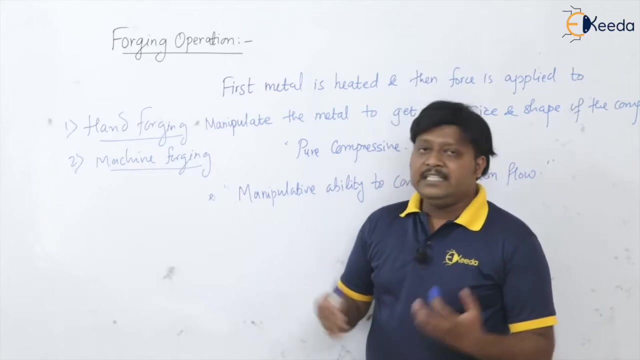 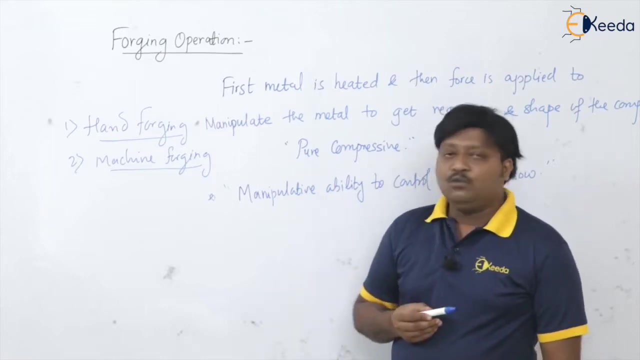 have and the another is machine forging. okay, so hand forging, whatever the force for the deformation of the part is given with the human hands. okay, so generally the drop hammers we can use here for the for the force. so that's why these are the hand forging operations. but when we look at the, this 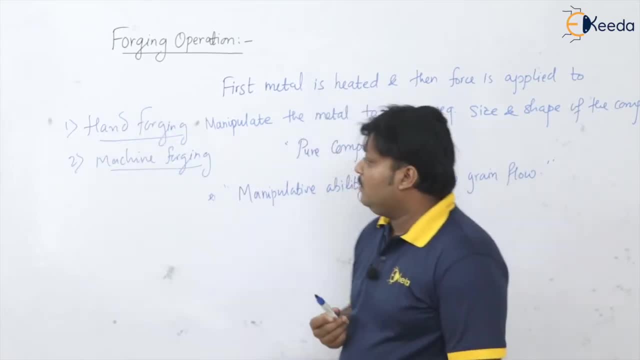 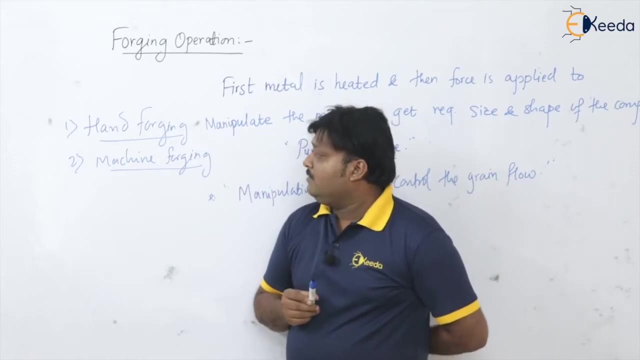 example of this hand forging, that is the blacksmith forging operation. so that's why these are the hand forging operations. but when we look at the operation, we have seen: okay, now, if you look at the machine forging, so in machine forging we are having the press forging, isn't it the press forging? 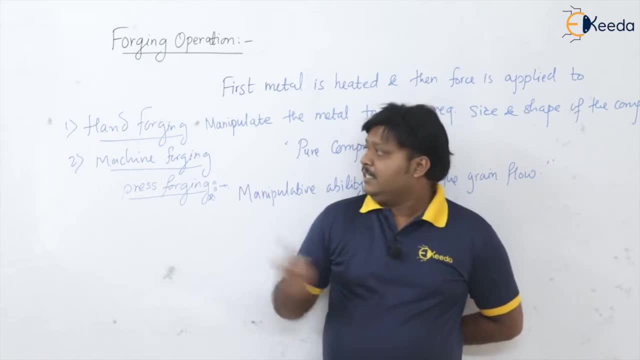 so see, in press forging, here the forces are applied by the drop hammers. okay, so the impact forces are are going to form, so, but these forces are the sudden and the kind of forces. impact force is going to apply on the product, but in press forging, whether, whatever the force is, 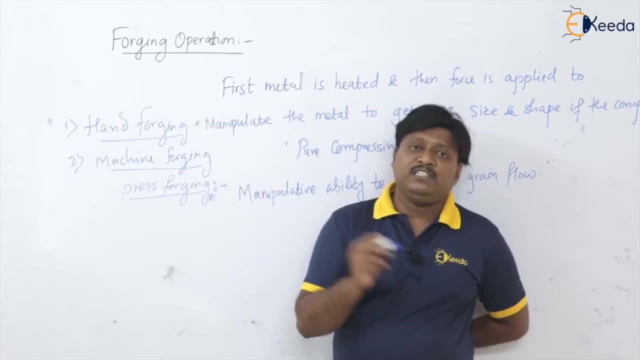 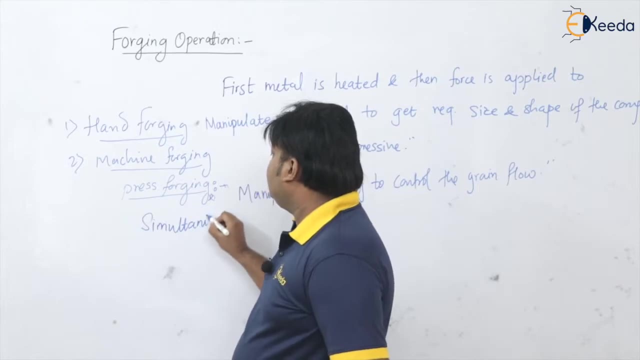 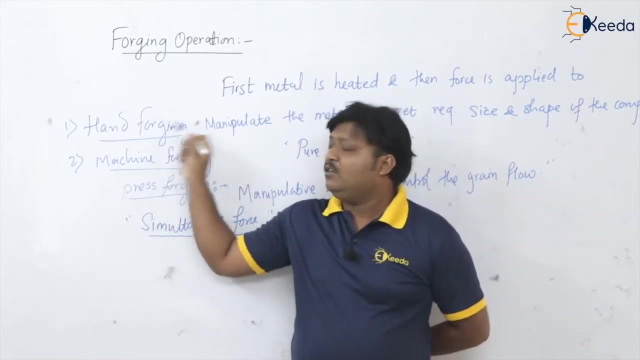 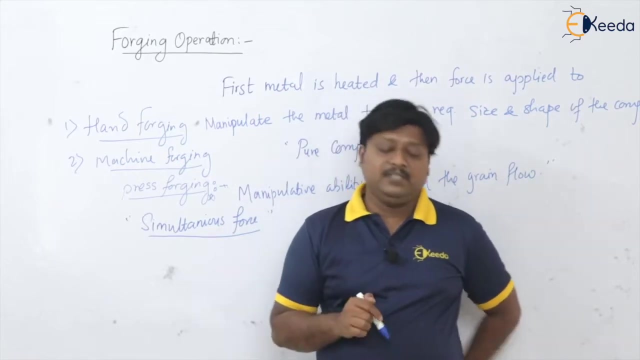 applied on the component is not the impact force, it is not a certain force, but it is the simultaneous force. it is simultaneous force, please remember. okay, so this is actually the press forging and we can now directly have the drop forging. please remember draw forging and press forging. these are the main classification that we have and these are 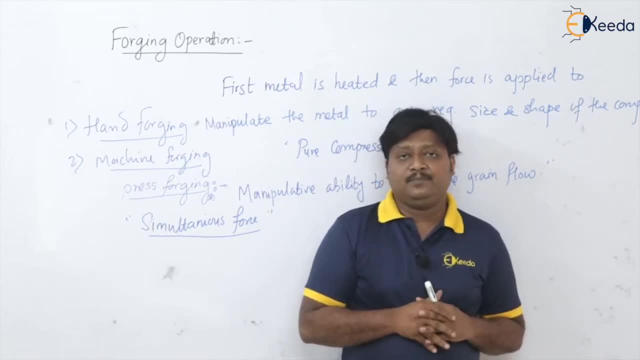 actually the closed, a forcing operation. in both operations the closed die is going to use wearing case of die forging the material is kept with donted sandpaper or the Take the case by some kind of a strong material in which the pressureHello again this is- survive that force and alluvium of different kind of material. if we take that now, if we put this, Suffloud has core código gemacht, so to that we have to use these two things, these measures, and they were used that way- is important what the work follows, because waxing it is a pure body. skating actually can not perform in real life but in fact every performance is moved continuously. R EMO Be a 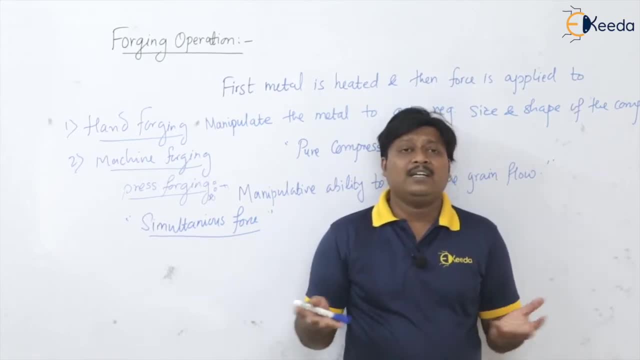 on the or the billet. material, that is, raw material, is kept on the lower die, whereas the press forging we are keeping the material into the die. okay, so that that is the basic difference. and the force applied in the drop forging is sudden force, the impact force, whereas the press. 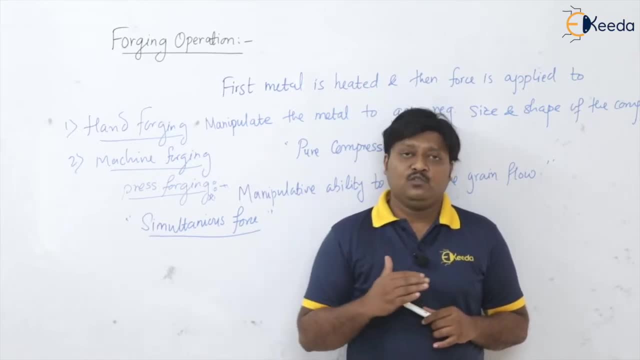 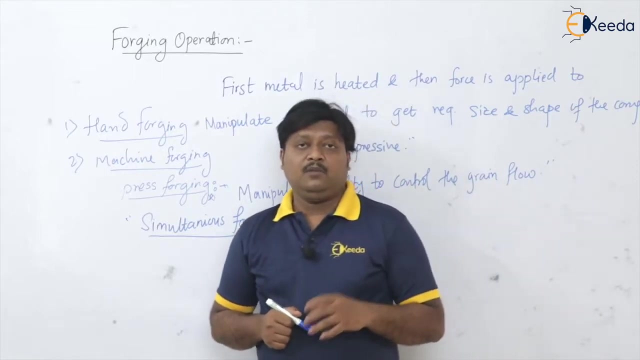 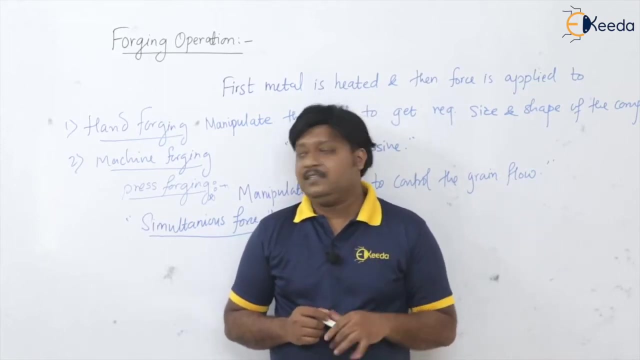 forging, we are having the simultaneous force, so simultaneously we are applying the force for the deformation of the material, not instantaneous or impact loads. please remember this. now, based upon the shape of the product obtained into the die, we are having the classification for forging operation. is that for the press forging? i am saying so in that we are having based upon 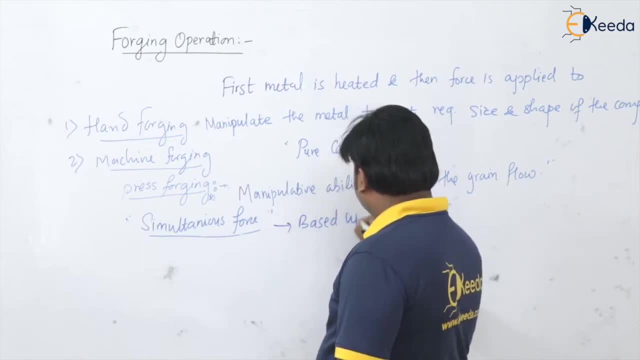 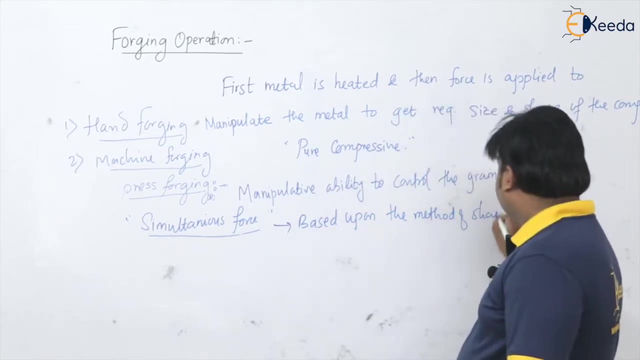 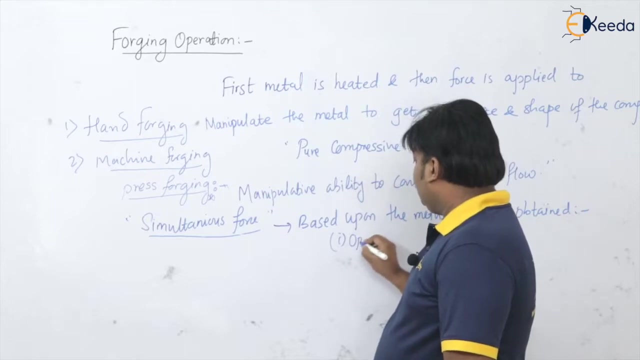 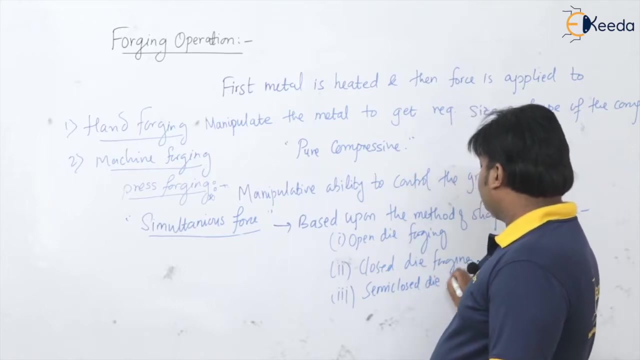 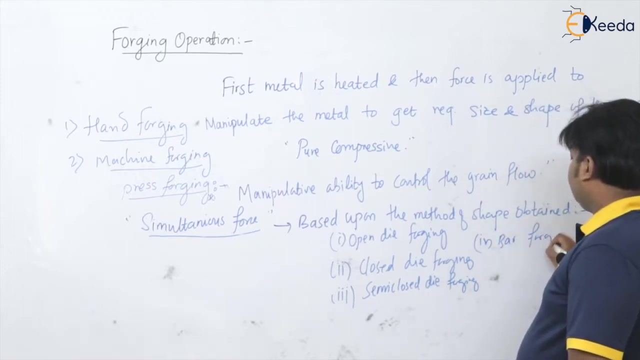 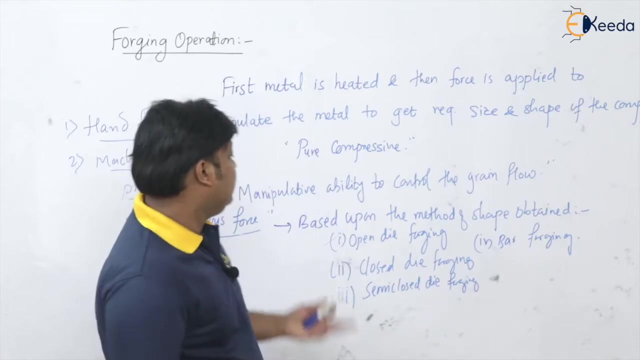 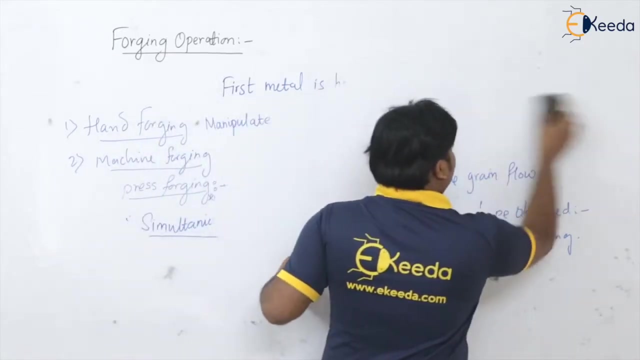 you the method of shape obtained. shape obtained: we are having number one, open die forging. second, we are having closed die forging. third, we are having semi closed. and fourth, the bar forging. the bar forging, let us see it one by one. so, open die forging, that is very simple if the metal is kept between the two closed dies and if you apply the force. 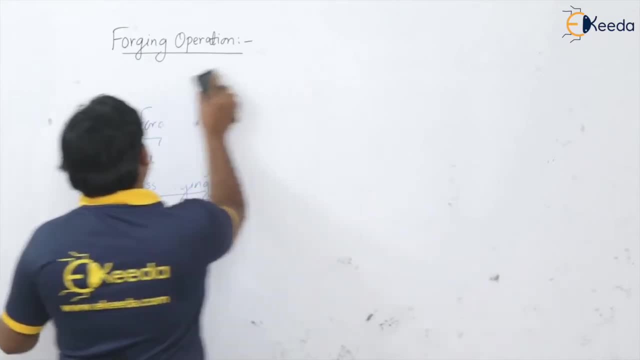 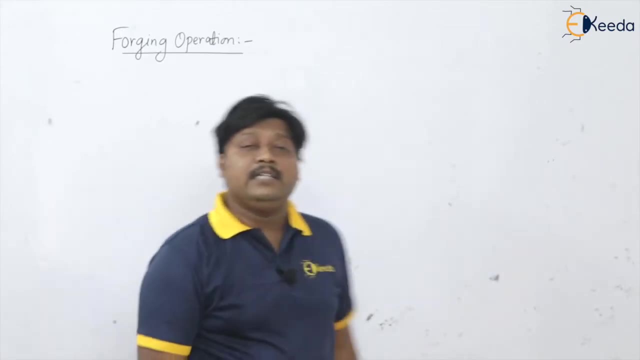 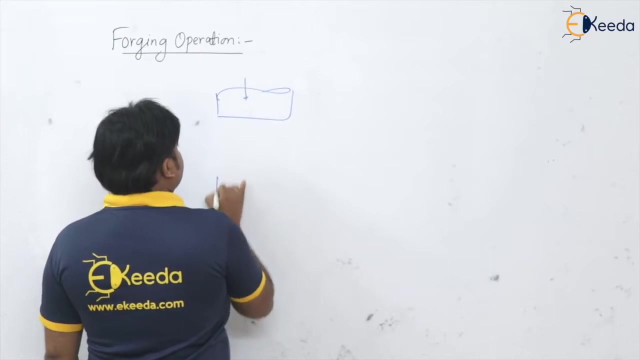 to get the deformation. so, in open condition, we are applying the force, isn't it? so this is the open die. forging is between these two dies. we are simply applying the force out of this. say, the lower die is stationary on the himalayan dimension, it must吧. 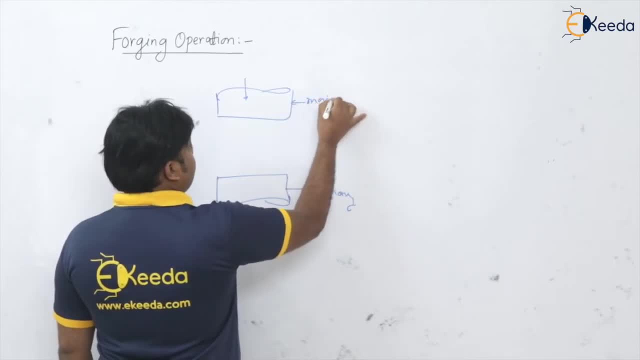 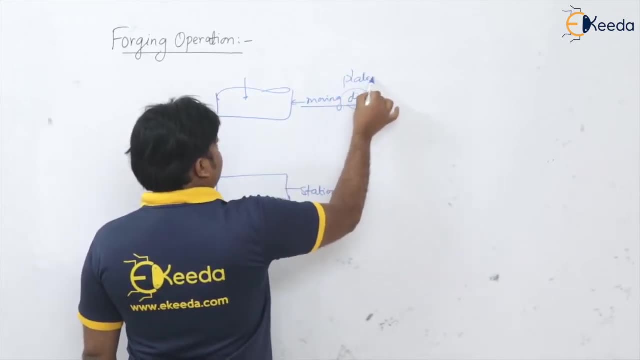 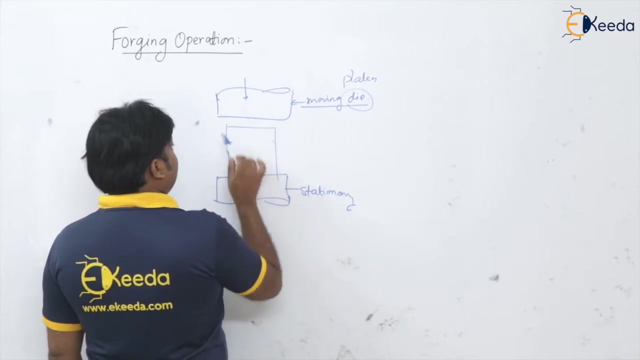 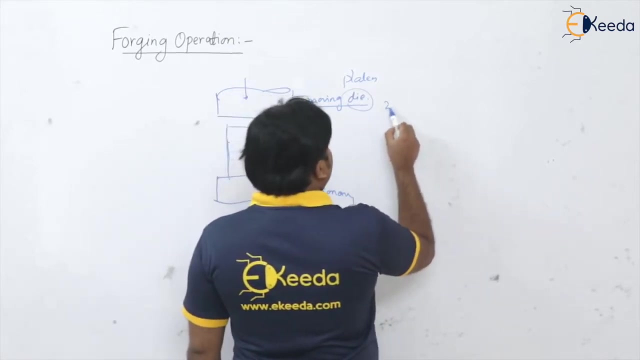 now we have cut off the wall of the 깊 and this is a moving die, or moving platen die is also known as the platen, and here is the material. okay, we are applying the force. so this is open die forging operation. then the next is what we are having, closed die forging operation, that is say, this is the die. 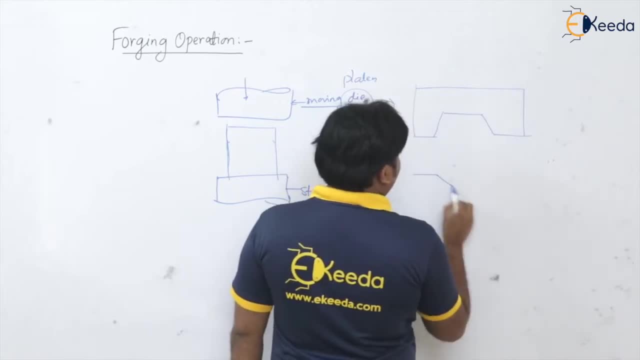 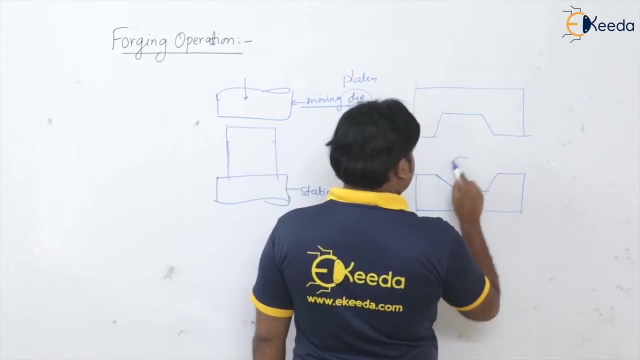 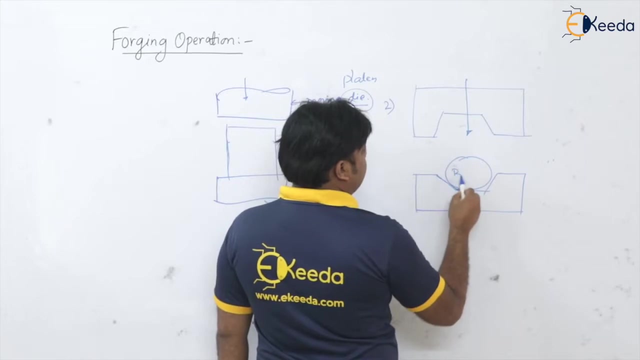 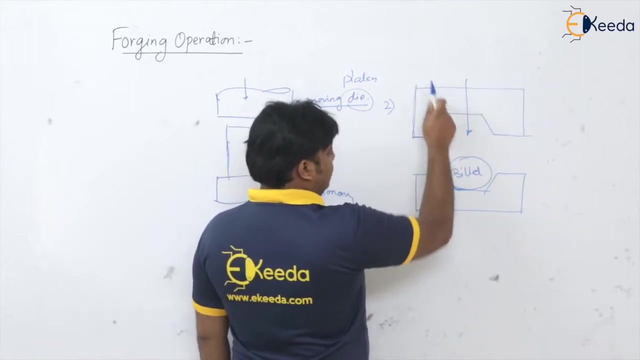 upper die and this is the lower die. so here the material is kept in the lower die, isn't it? and now you are applying the force, so this billet material is going to flow at each and every corner in the die when the die are meeting together and the entire surface here is closed, like this: 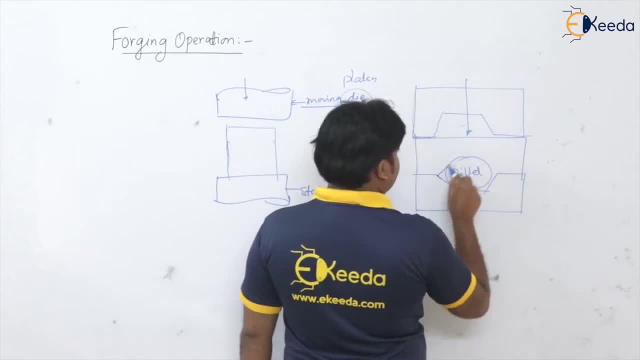 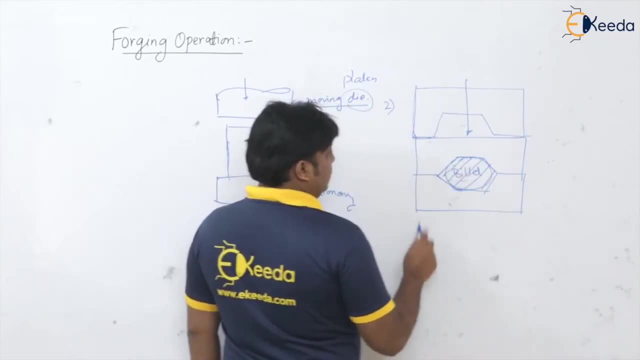 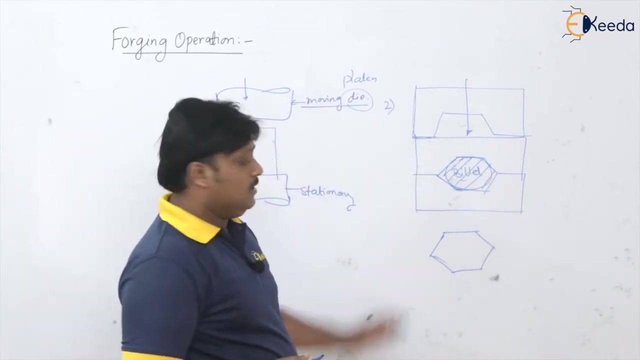 after some time, the die will be like this: okay, so that this billet material will flow to the each and every corner in the die. so this is the part will be get like this. so this is what enclosed condition, isn't it? when the two dies are closed. so this is a closed die forging operation. 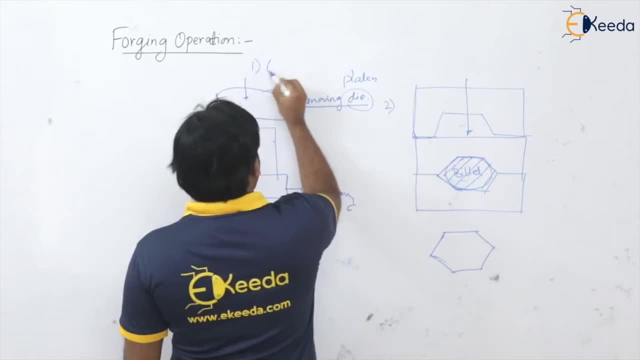 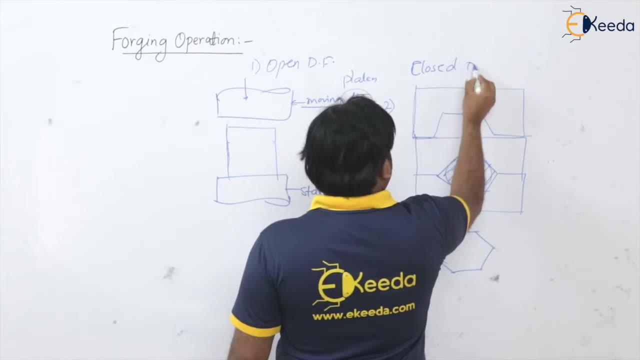 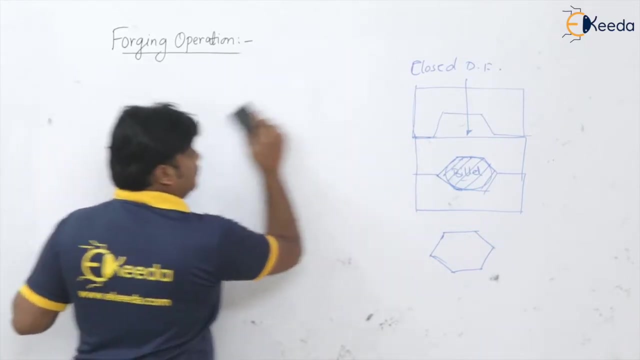 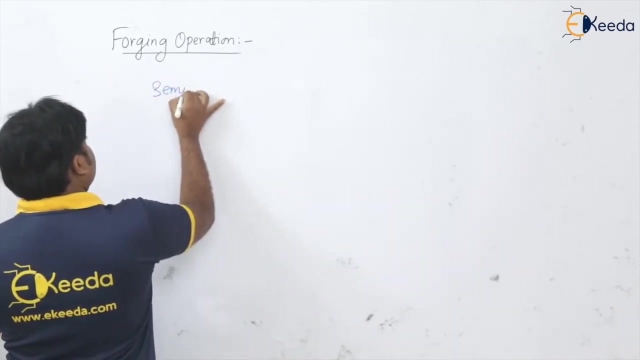 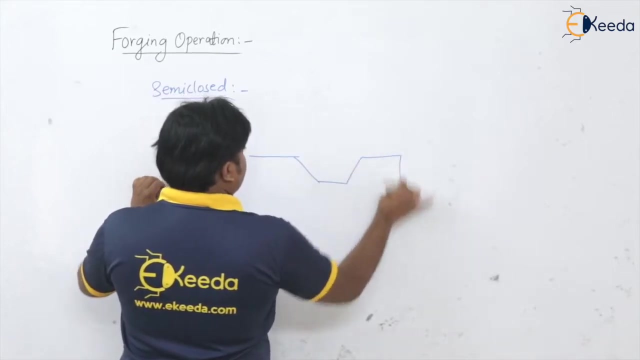 okay, this is the second. this is first open. die forging. this is the second. this is open. die forging operation is second closed. die forging- now the third is what we are having, that is semi closed. no doubt we are having the die for doing the work, okay, but here the 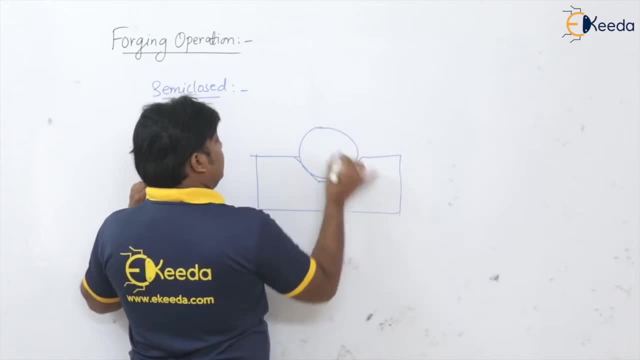 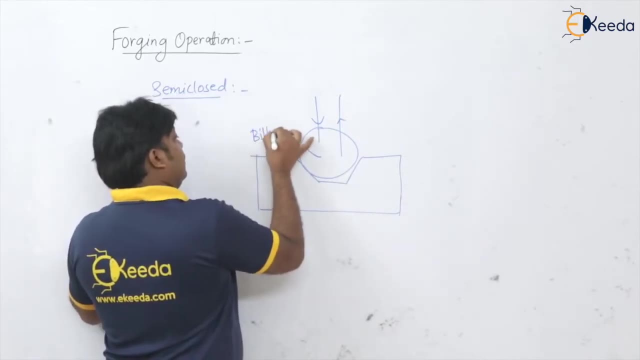 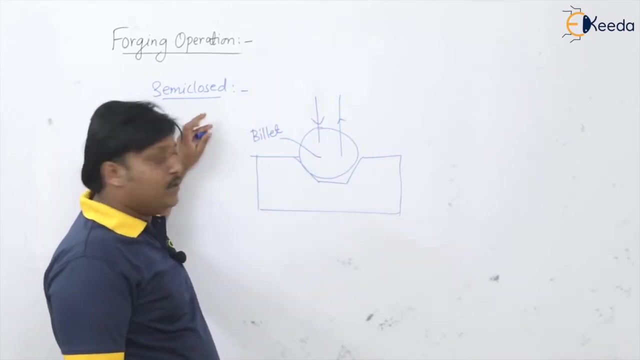 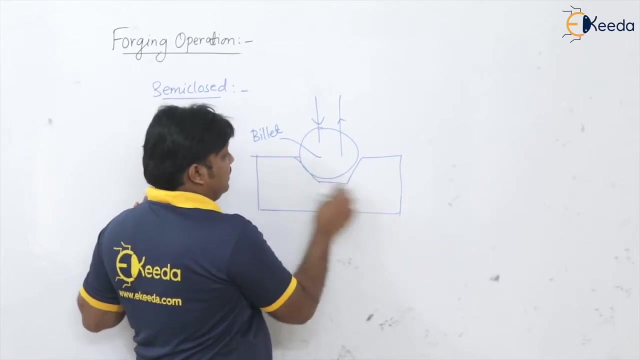 forces are applied in the open condition, just by changing the position of this billet material in between the strokes that are given by this, say, hammer, or that die, okay, so whatever the shape on the product is obtained by the die which is having the shape on the die, the same shape we are going to obtain on the 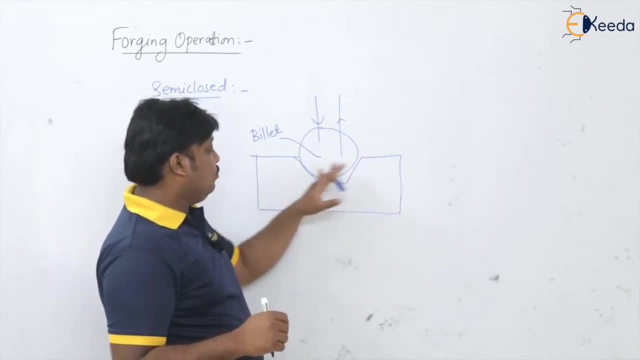 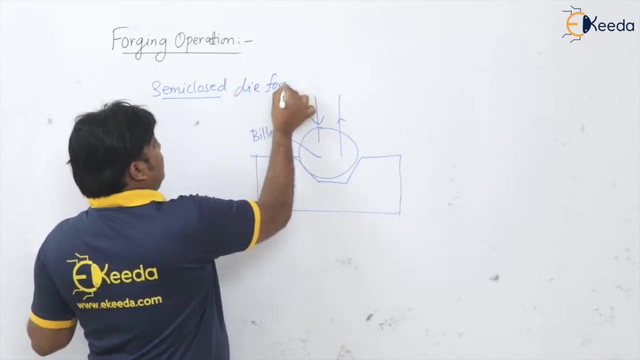 material. the thing is that here, by using this closed die only, the forces are applied in an open condition by changing the position of the billet in between the strokes. so that is why the name is the semi closed die forging operation. semi closed die forging option. this is the semi closed die forging operation and 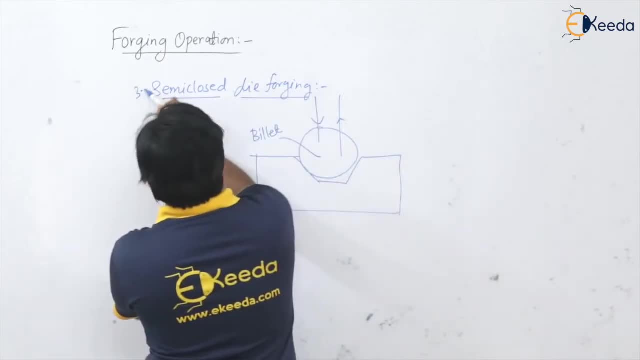 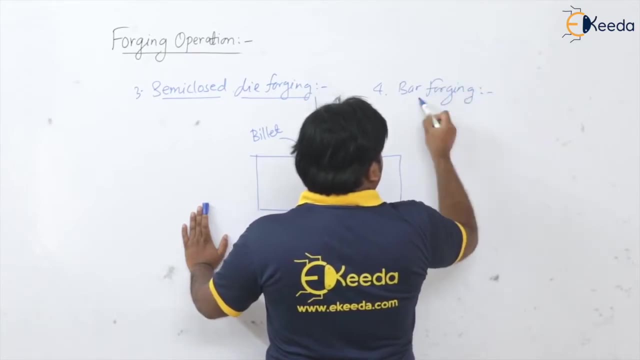 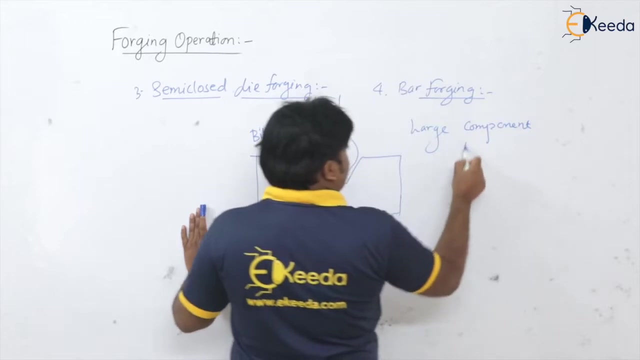 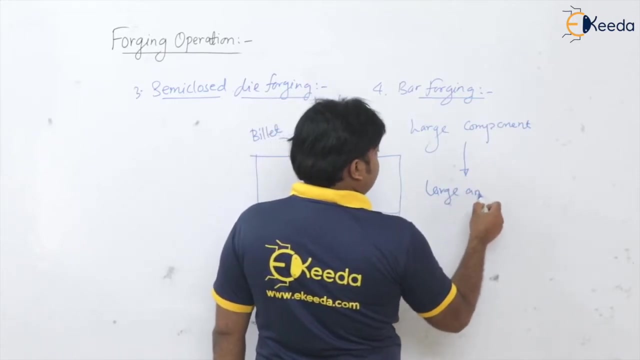 last one, that is we are having. this is third one and last one is bar forging. so whenever we are going to have the very large components, large components, so definitely if your component is very large, to deform this component by the in the forging you need the large amount of forces and power consumption is, isn't it? 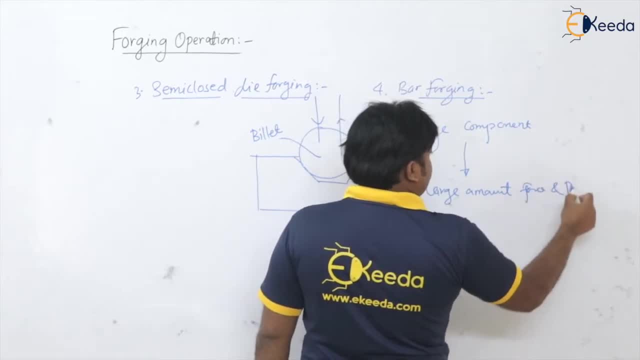 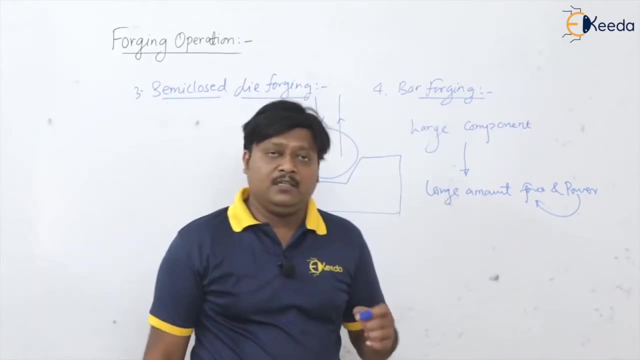 large amount of force and power to get this force, isn't it? so, in that case, what we are doing, instead of forging the product or component at a single stroke, we are going to have a little little forging of that part separately. okay, so instead of having the entire component forging at a single stage, at a single 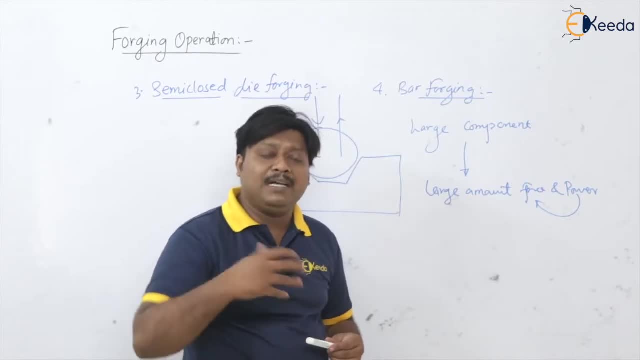 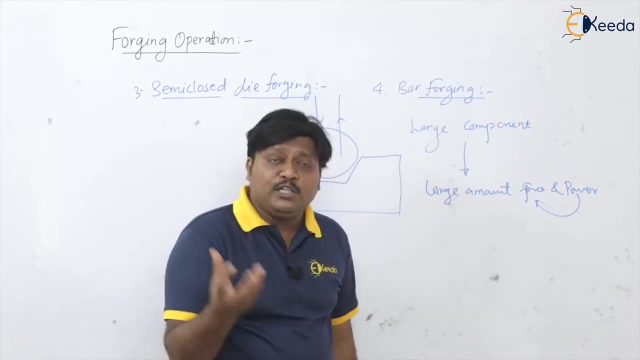 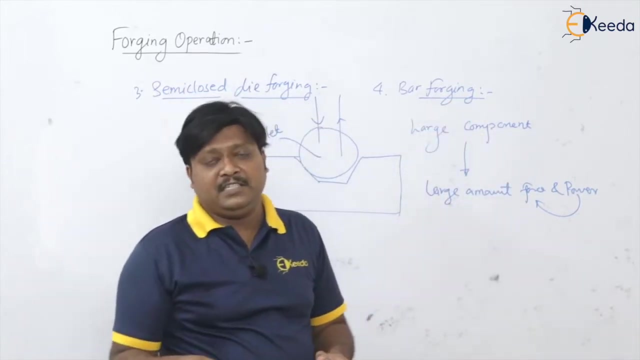 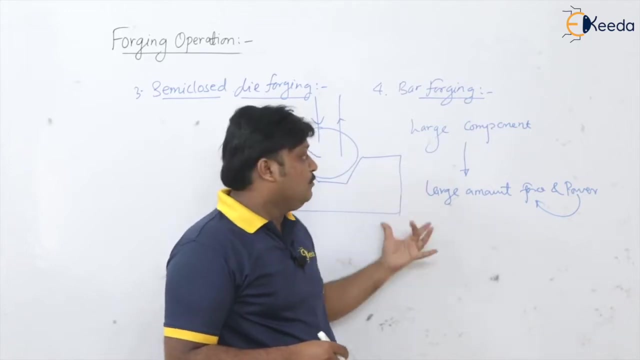 blow. we are trying to have the number of steps, number of passes, number of blows are required. we do this that by forging small, small portions, this large component should be forged so that technique, instead of forging the entire part at a single stage, now we are going to forge little, little quantity of 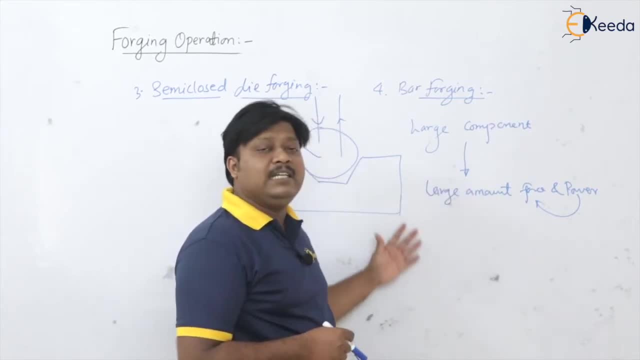 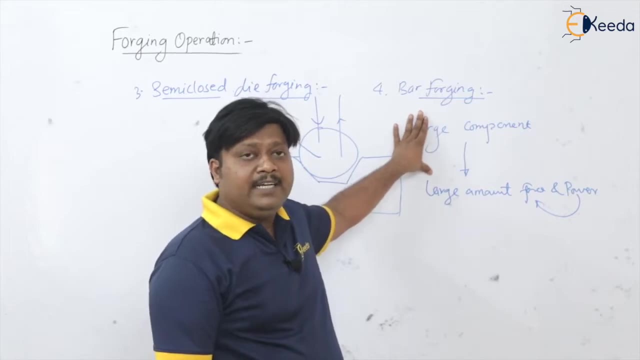 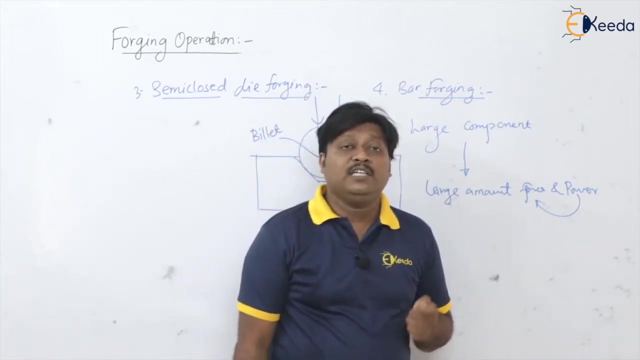 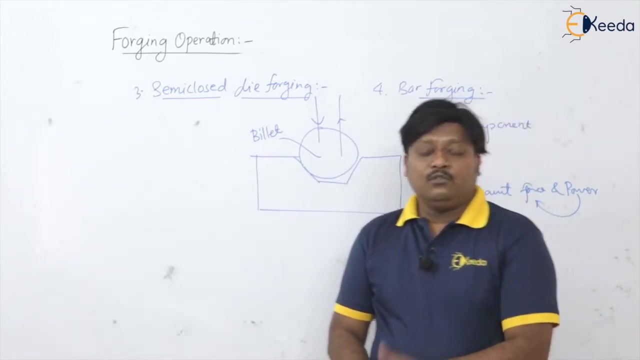 that part and using this little little amount of forging, we get this entire component. this is known as the bar forging. okay, so these are the techniques based upon the method of shape obtained by the positioning of the component. so this is open die forging. closed die forging. it is semi closed die forging. 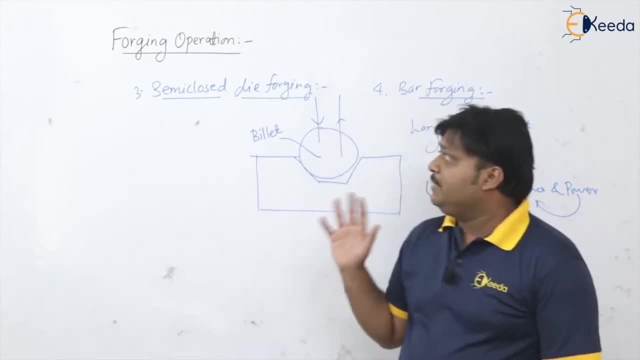 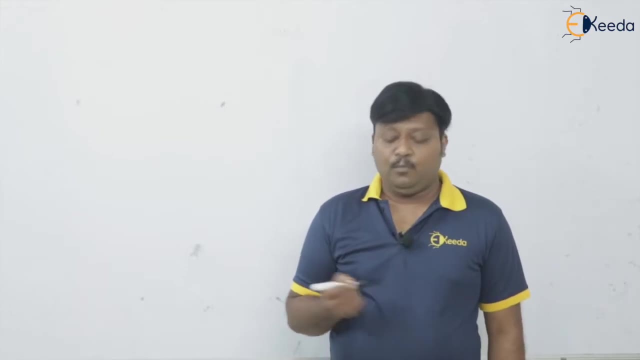 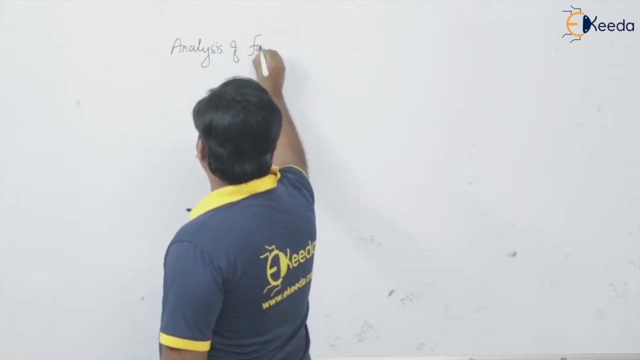 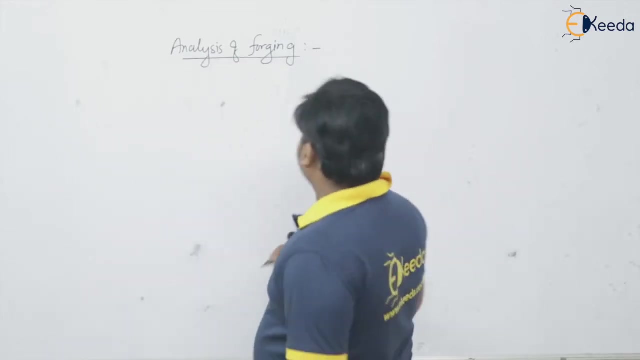 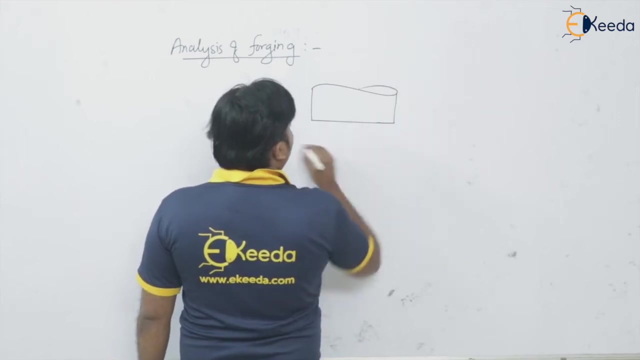 and bar forging. so these are, this is the basic classification of forging process. now we are going to see the analysis of forging operation, the analysis of forging. so for that say, I am taking here this top die which is moving, we are having the cylindrical billet here and 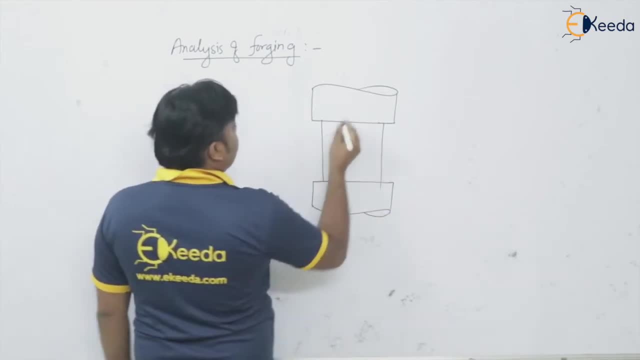 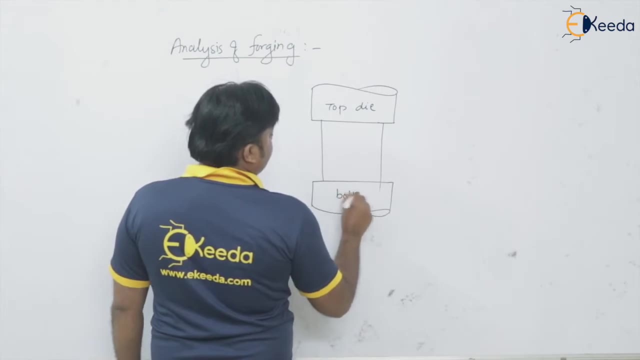 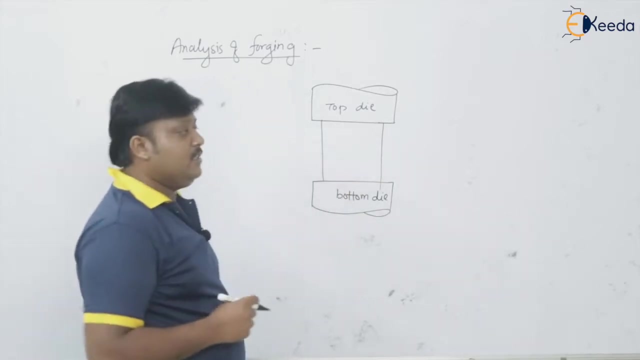 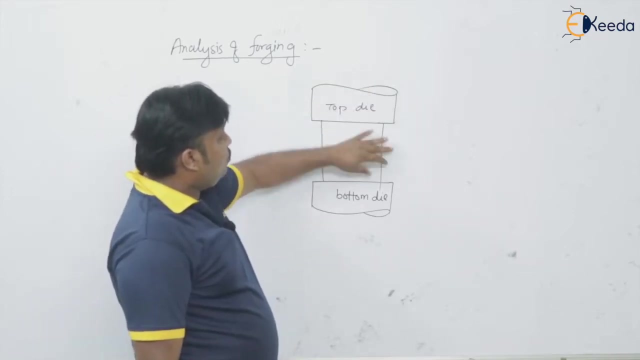 it is the bottom die or stationary die. okay, so this is top die, this is bottom die and this is our cylindrical billet. material or raw material is there. so see here in the initial condition of the forging, when the force is applied by this top die on to the workpiece. so there are the outward expansion forces. 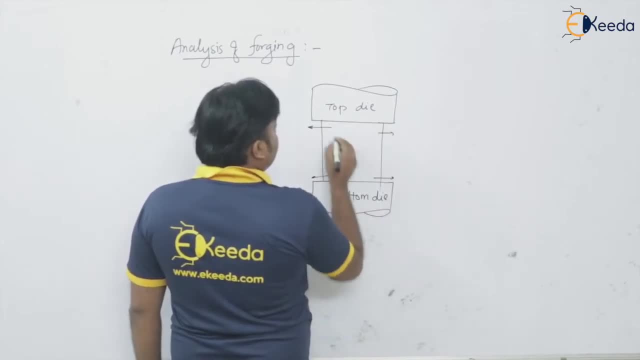 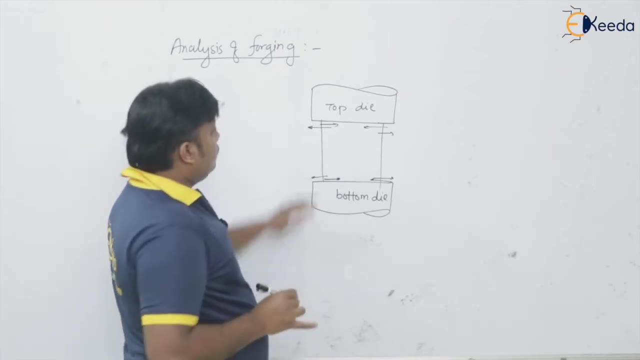 and the frictional, inward frictional forces on to the interface between the die and raw material. so initially, what happens there when the force applied by this top die on to this raw material or billet material? so at the interface of this raw material and this billet there will be the outward expansion forces and the 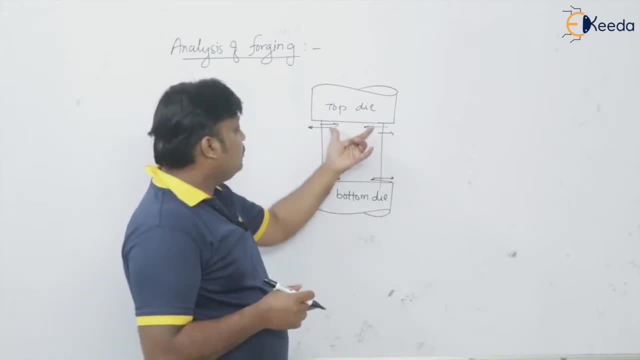 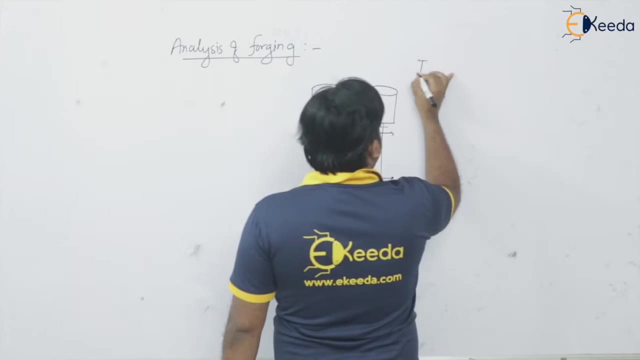 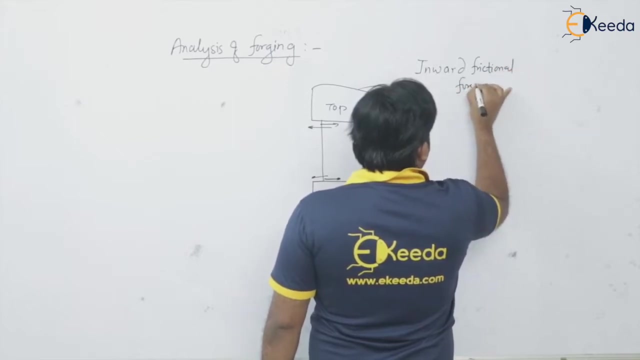 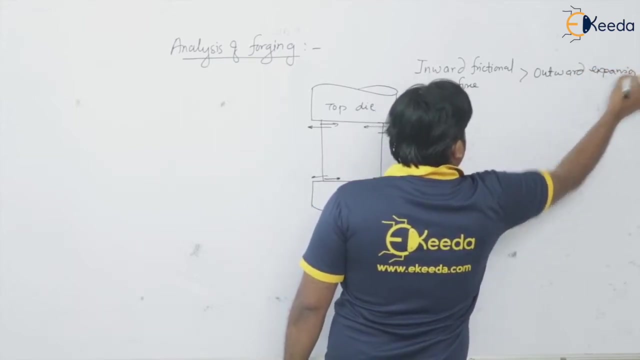 inward frictional forces are going to exit exist. so here, these inward frictional forces actually are greater than the inward frictional force, is greater than outward expansion force, expansion force. so because of that, what is going to happen? the raw material is going to repeat the conventional direction of the motion and therefore the downward fraction is included, and inward frictional force is not going to want to act onwards. ive is moving and outwardambient so thisようnasit Powder- following this λwT help that this is going to get the simulationsafe expansion 0f1 gene. the materials in the process external, foster the modeling of the different forces in a rendering side that is standard. Zx 1- shy, 1- fix. you have the overall current lick theon electron☆ Artㅋㅋ. 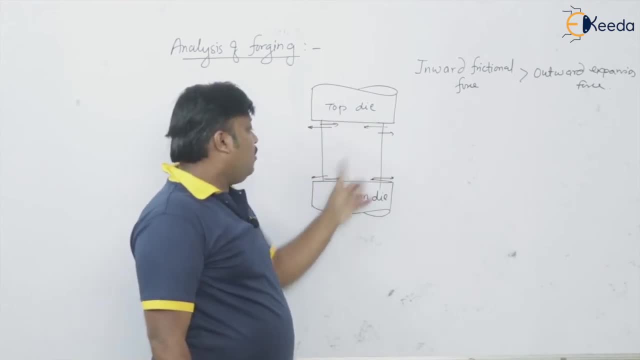 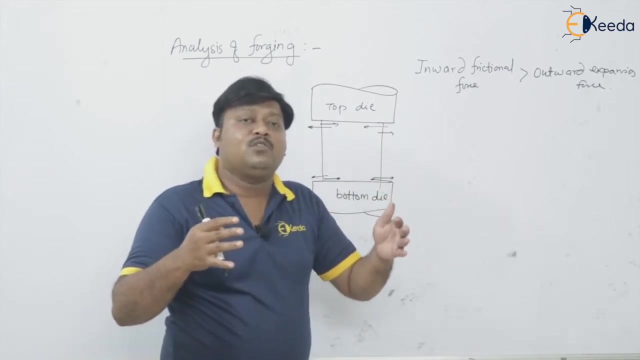 material or this billet material is going to stick on the die surface, okay. and when, say, the die is moving towards the center of this height of the component? so what is going to happen? see now, the outward expansion forces are goes on increasing, whereas the inward frictional forces are the same. so here, 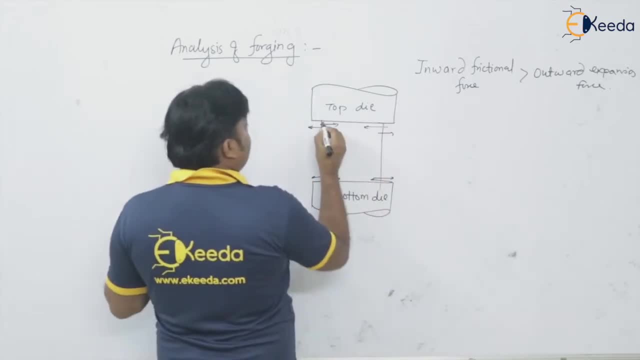 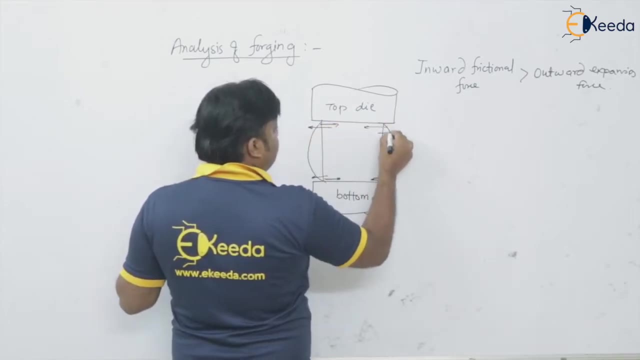 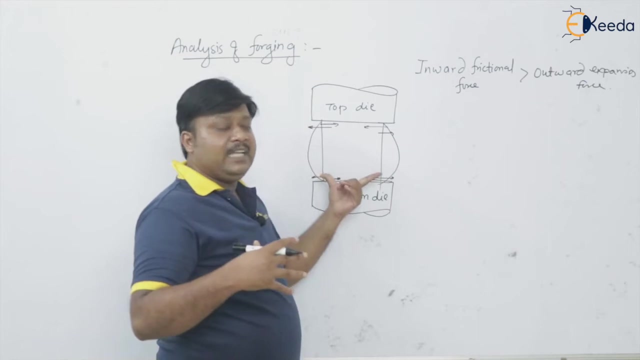 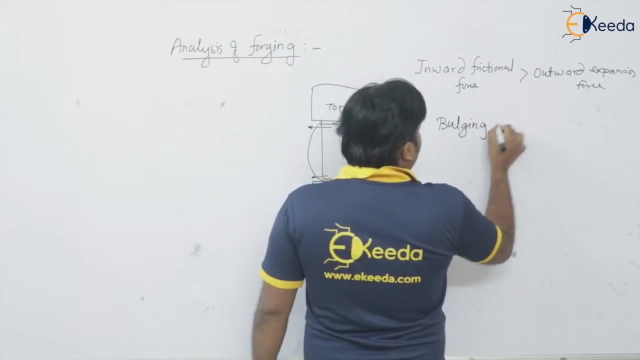 what happened as this outward expansion forces goes on increasing when the die is coming down, so there will be the bulging of this cylindrical raw material. okay, bulging means what they diameter is going to increase at the middle. that is a barreling. also, cabal disco bulging or barreling will be there, barreling. 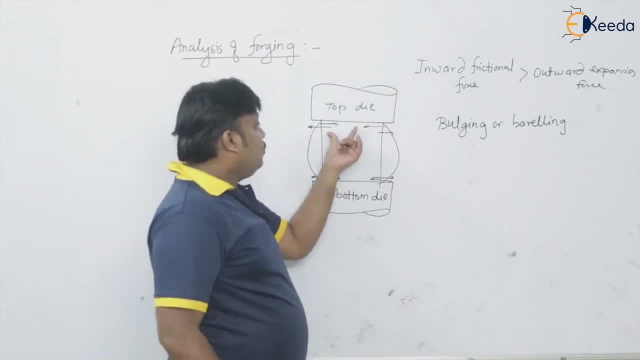 because of the. now the outward expansion forces are goes on increasing. now see the ordering of the die is increasing or accurate. ok, now we should focus on our overall operation. can see here this first part or first initial condition of this forging operation. we can call it as the sticking condition, where the 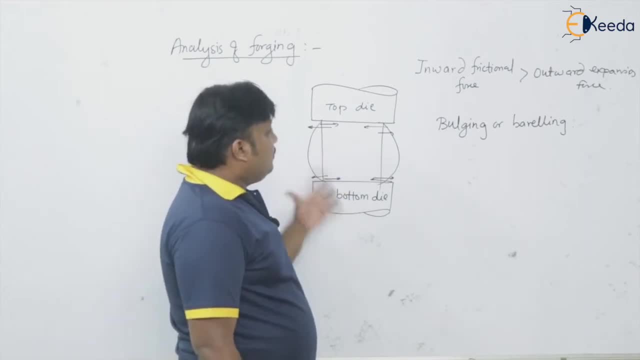 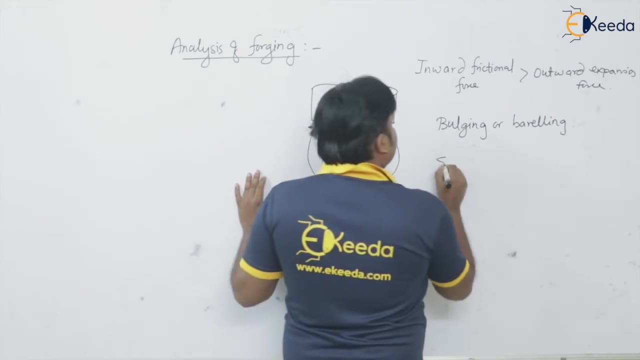 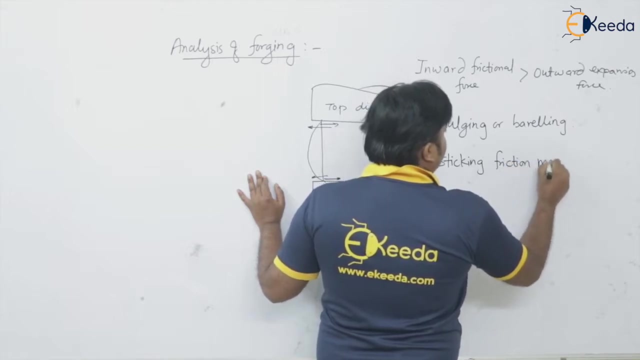 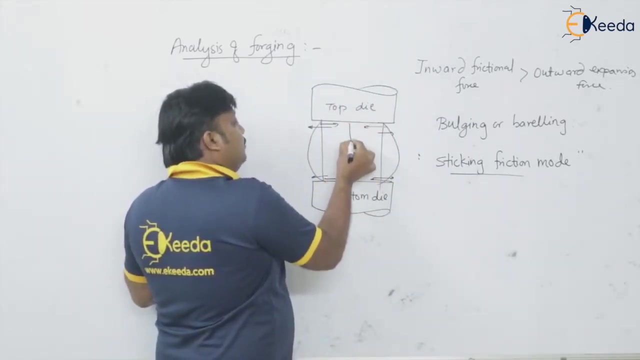 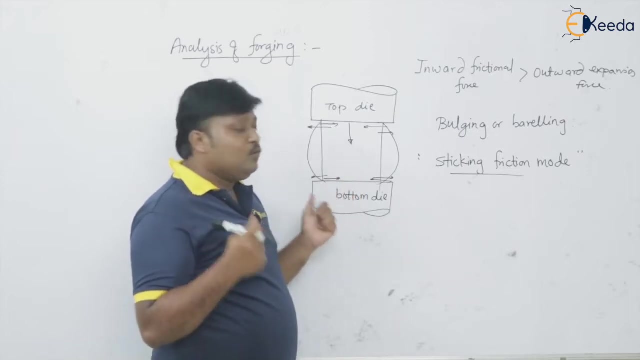 material is stick on the die surface and bulging occur. ok, so the first part of sticking friction model, sticking friction model. okay, now see the punch, now, sorry, the die, now moving ahead to get this billet material force. so what is happening at some moment or at certain time? what happened? the outward 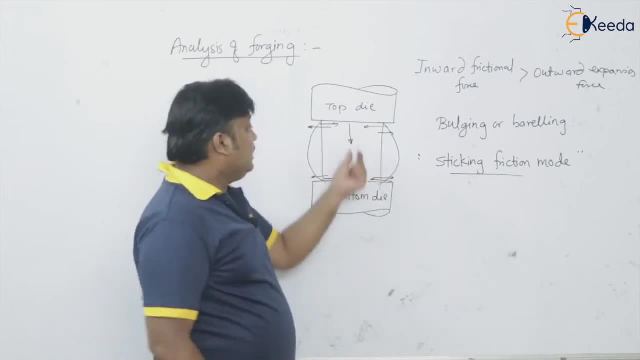 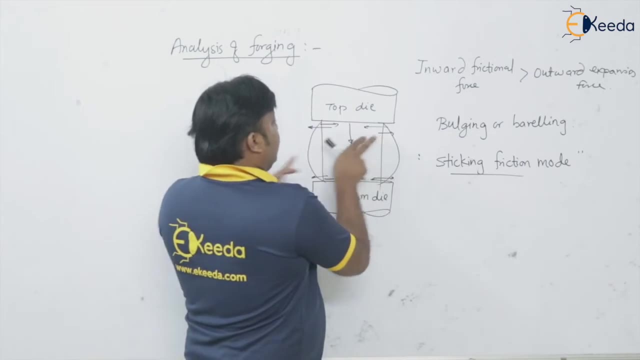 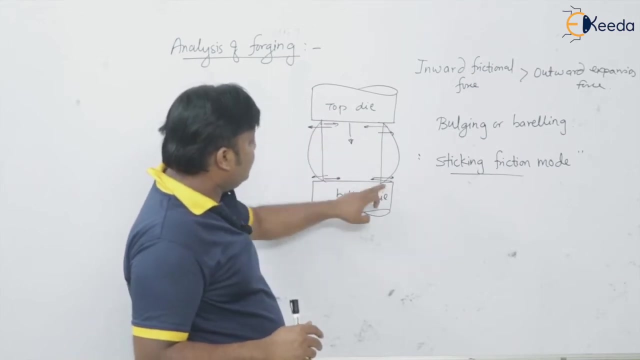 expansion forces are become more than this. inward fictional forces- okay, Peleca ha. inward fictional forces, Jota way. expansion for, say, Jada, hey, is Kiva Jessica? oh God, ha this material? gahoo, gahda a die surface cue per stick. oh, gahda, okay, or is Kiva jesse? at the ends it was get stick to. 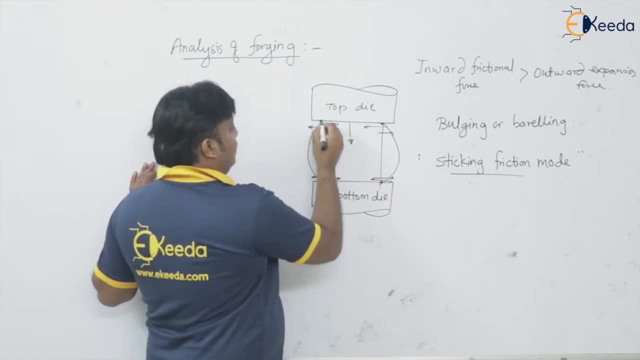 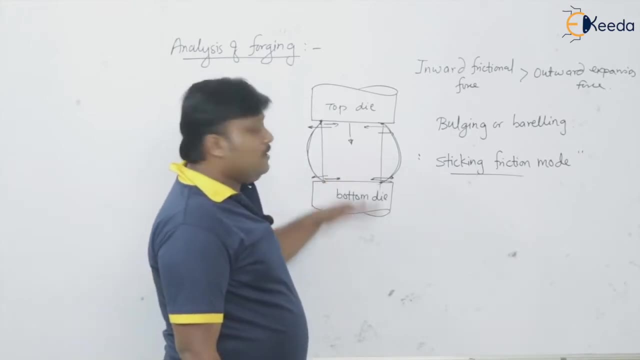 the plate or the die and there is a occurrence of battle in or bulging. but now what happened? after certain time, the inward fictional forces are stationary, they are constant, but the outward expansion forces goes on increasing. that's why what is going to happen now, the material is now going to 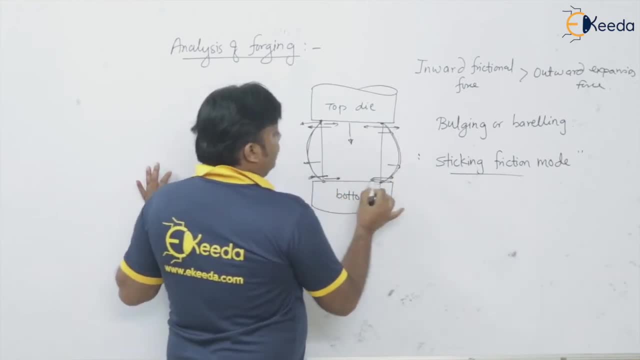 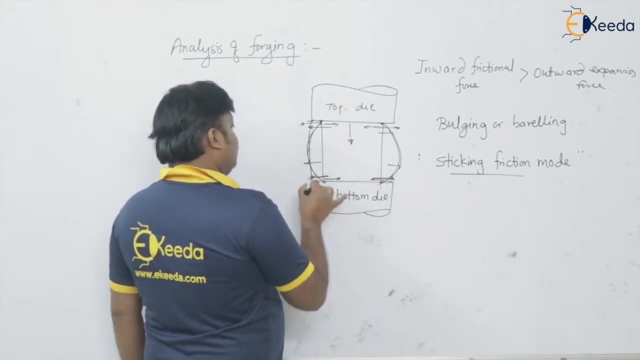 slide material is now going to slide over the die surfaces. okay, and because of that, now we are going to get the die here. okay, if you flip the die we have into here and there and now, when you momentum, now fifteen, viewing this, because the die with this direction, it is becoming weak and here we are going to get. 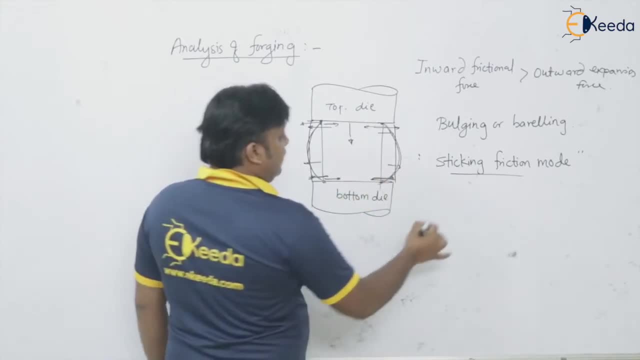 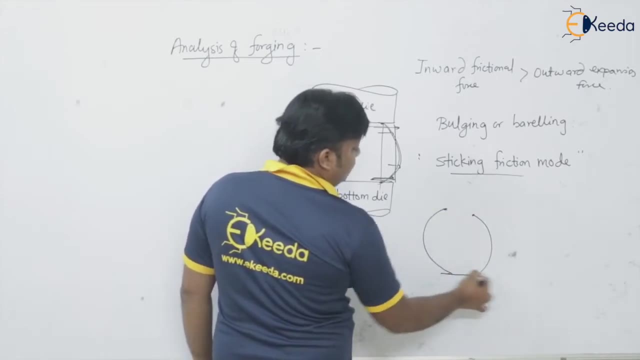 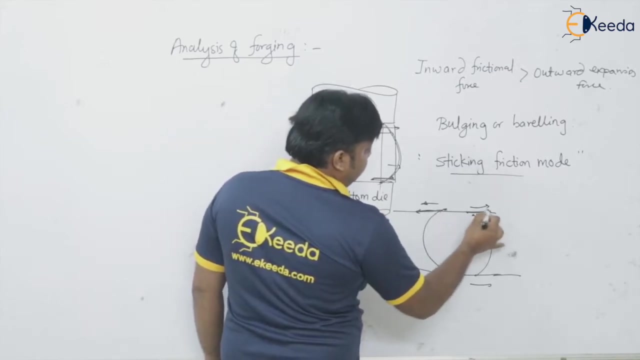 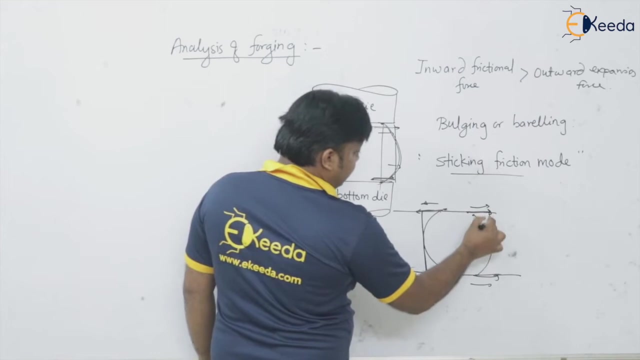 the straight cylinder. see, there was a barreling at ends. the material was sticking to the die surface. now, what is going to happen now? because of this, outward expansion forces are more now. now the material is now going to slide over this surface of the, this die, and we are now getting the straight cylinder. 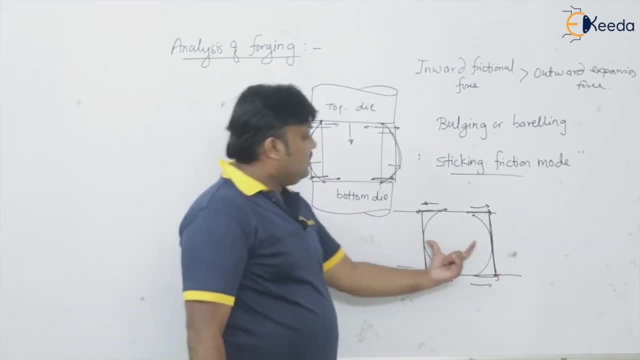 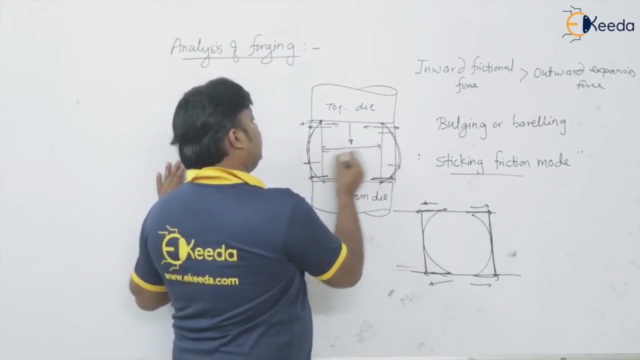 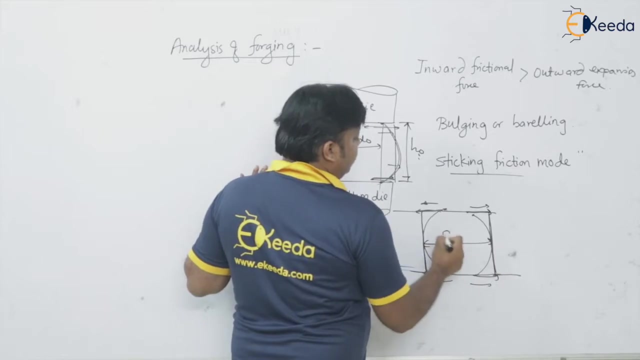 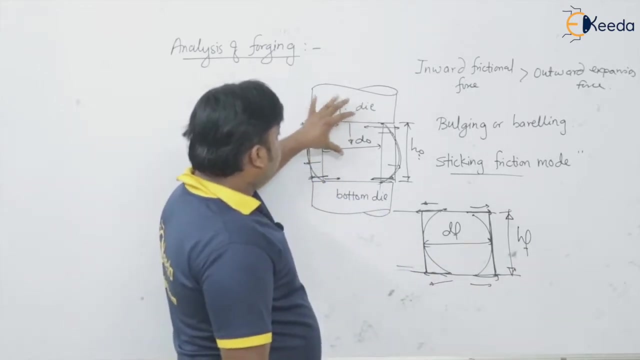 isn't it okay? so now bulging is disappear and you are getting the straight cylindrical, surface, cylindrical, this workpiece, having we change the dimension, that is now this suppose, original diameter. do one there. initially original height was there is initially HO. now the diameter becomes D, final and height becomes H, final. so we can see, because of this, upsetting. this is nothing but the open die forging between the two dies. we are compressing or deforming the material. this is the upsetting process. so definitely there will be the decrease in the height and increase in the diameter. okay, so this, this second part of the die, is: 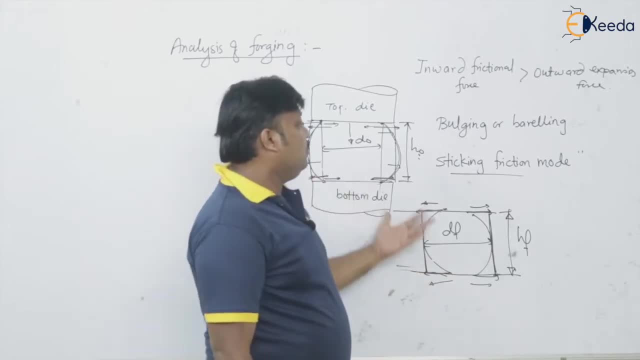 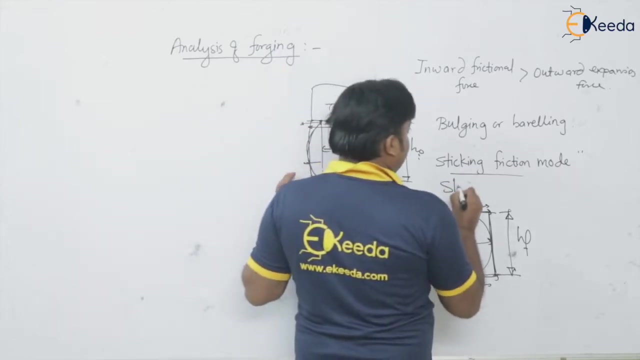 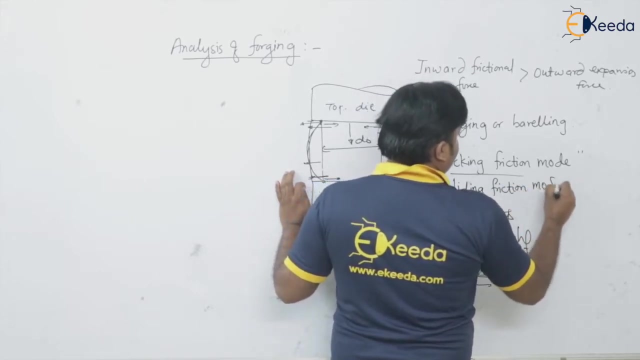 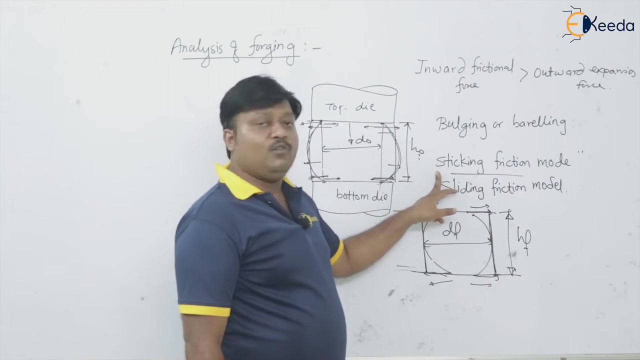 difference in size according to the defected area, given the difference difference in width between the die. so we're just starting. when we called the systemнул two gender. we're going to use this function, λm and the, the sticking friction model first and then sliding friction model. see, because of this. 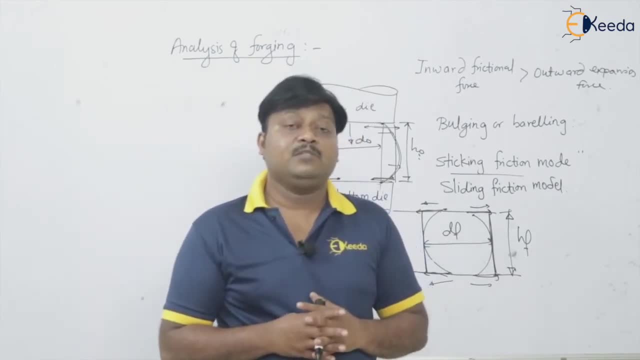 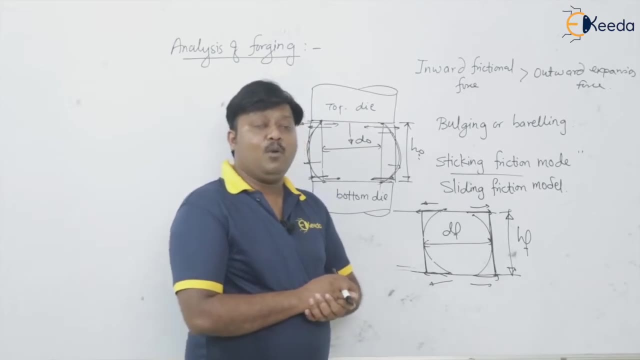 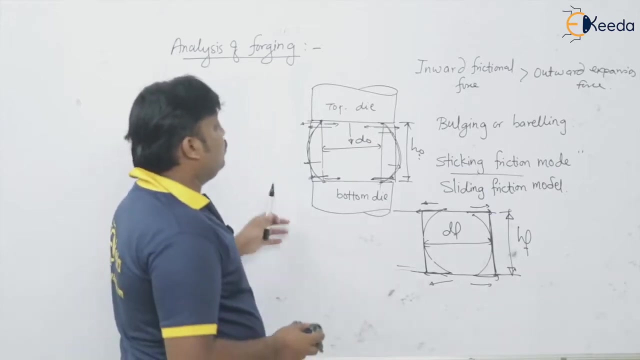 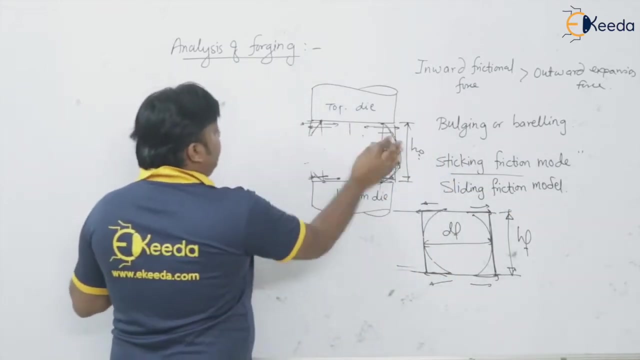 that is, the initially inward expansion forces are more than outward expansion forces. we are getting the very accurate dimensions in case of the forging operation. so this is about the basic thing, about the analysis of the forging, on which base we are doing the analysis. that is, these are the two conditions. okay, now see one more thing i want to discuss here. that is about 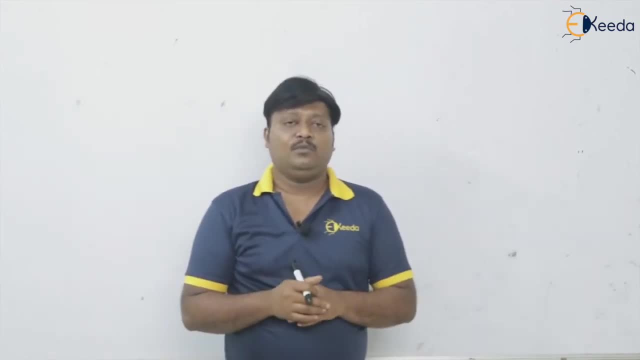 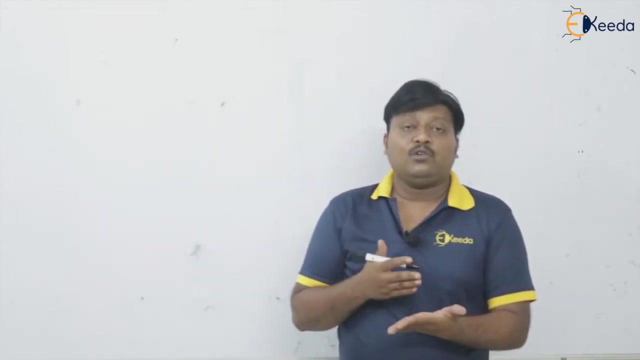 the open die forging and closed die forging operations. see as this operation, as just now we discussed, is what is a open die forging operation, but when we talk about the closed die forging operations, okay, so i want to talk about the volume of the raw material that we are going to take for the open die forging operation and closed die forging operation, see in generally: open die condition, open die forging operation: whatever the volume of material of the product or final product you want to achieve is taken as the volume of the raw material, that is, volume of final product. 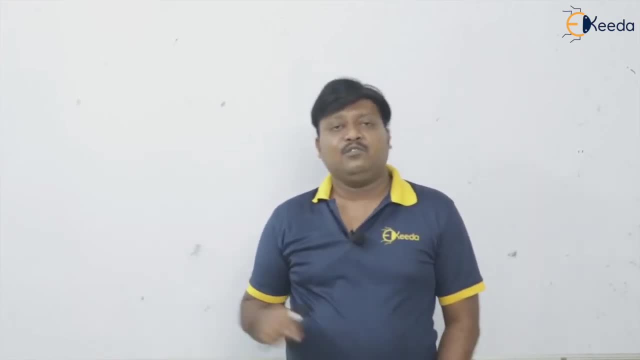 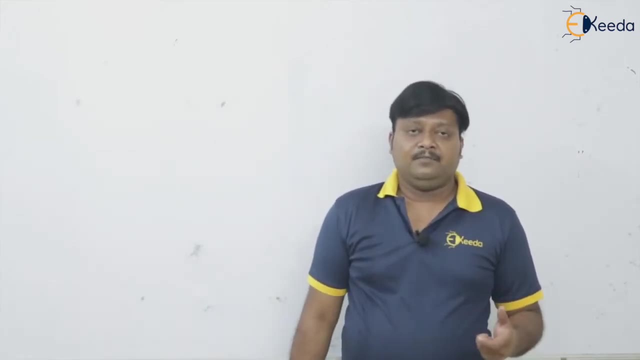 is nothing but the volume of the raw material you are taking for the forging operation. but when you talk about the closed die forging operation you have to take, say x is the volume of final force product, then if you want to the, you want to take the raw material. for the forging operation, then the volume of that raw material in the closed die forging operation is 10 to 20 percent of this volume of the final product. okay, so why it is so? so during the close die forging operation we really want to confirm that the material should reach to the each and every cavity or 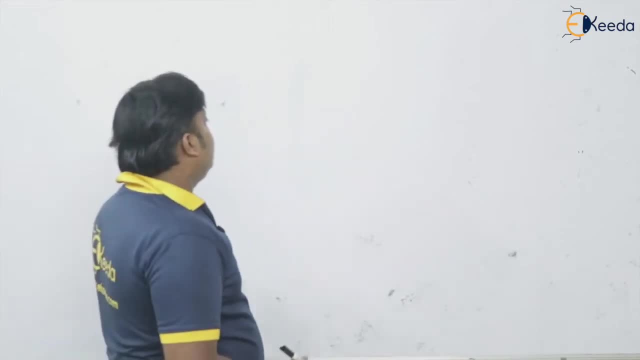 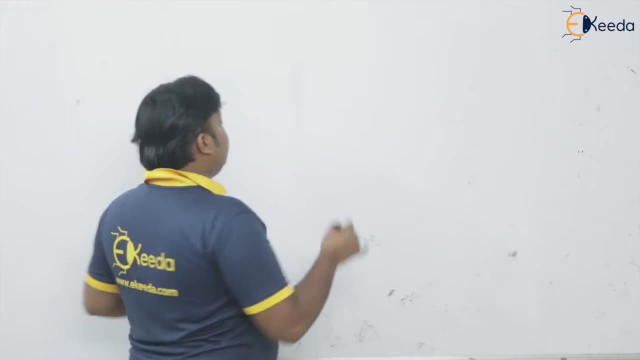 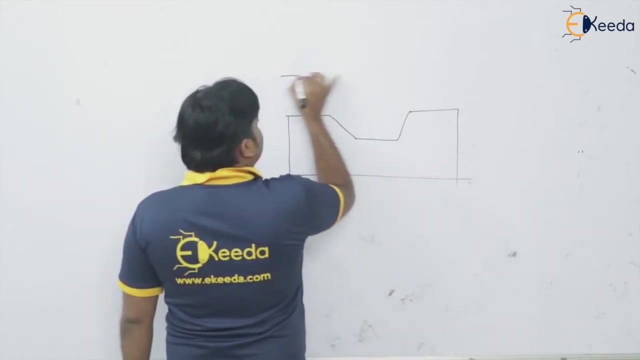 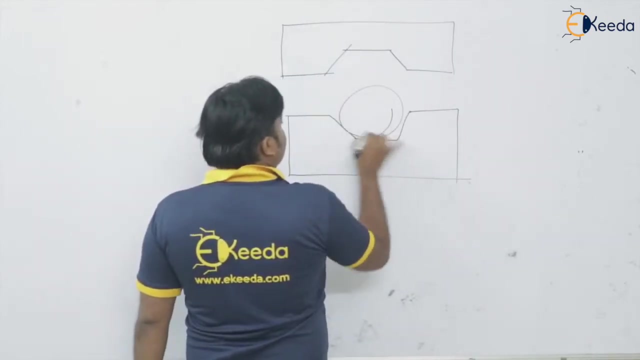 the impression that you are having into that closed die. so once the die is going to close, we cannot see how the material flow is going to happen where the material is flowing in case of, say, the closed die forging operation, isn't it so for that reason we are providing, so the volume of this raw material in case of this closed die forging. 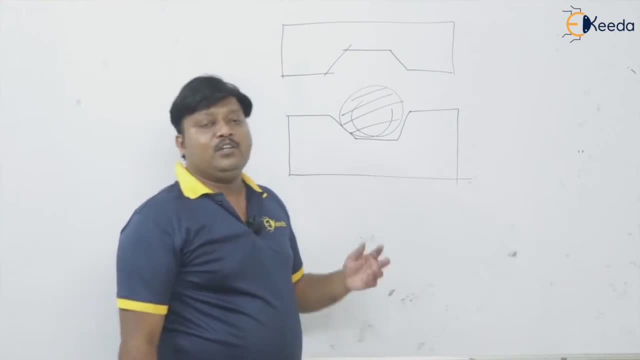 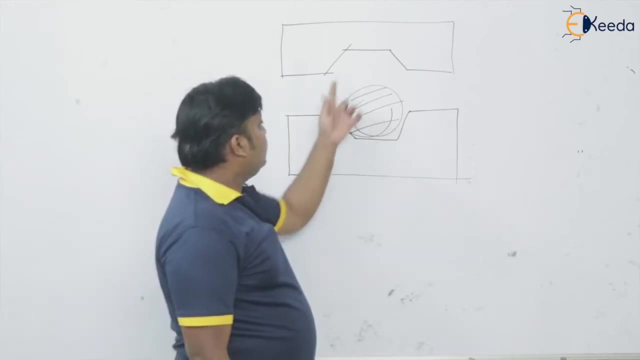 is 10 to 15 percent more than that of the volume of the final product. okay then, sir, you will ask the question that, sir, where this, this extra material, is going to accumulate, isn't it so once? no doubt, the actual volume of the component or product is x only. 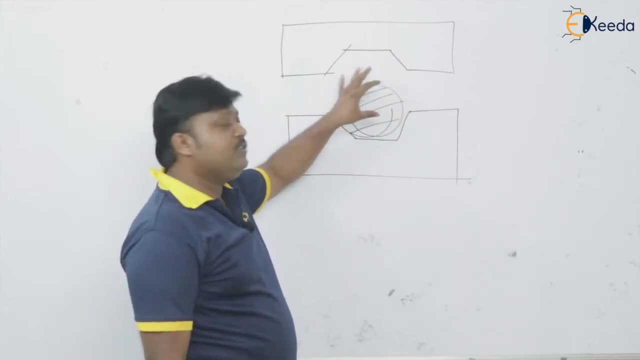 sorry, that is going to fill in the cavity when we put the extra material. now the thing is that where this extra or excess material that we have provided will go once these dies are closed, where the extra material will go after filling of the each and every impression or each and every corner in the die. so for that. 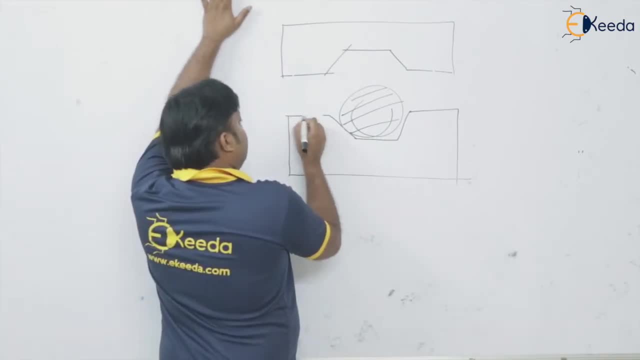 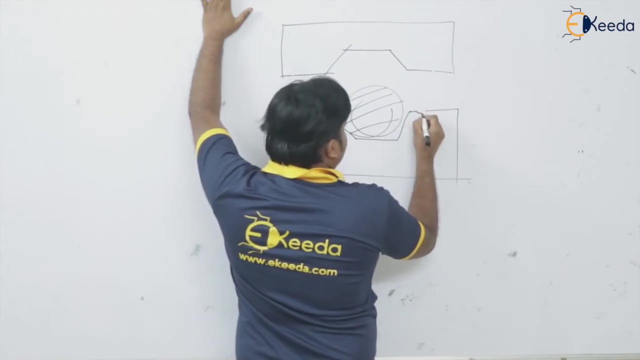 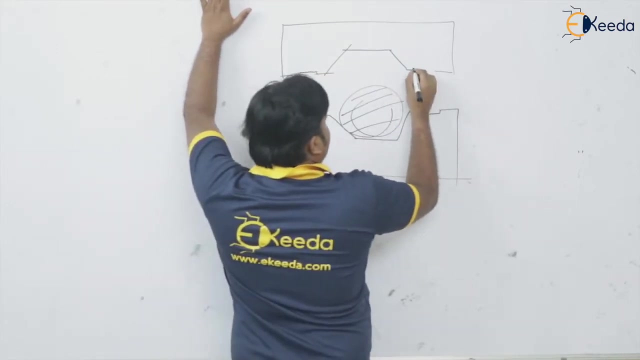 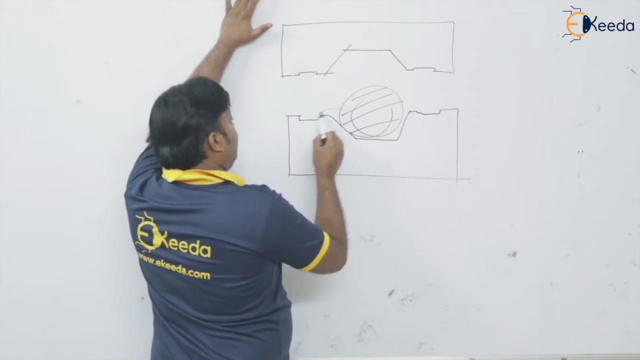 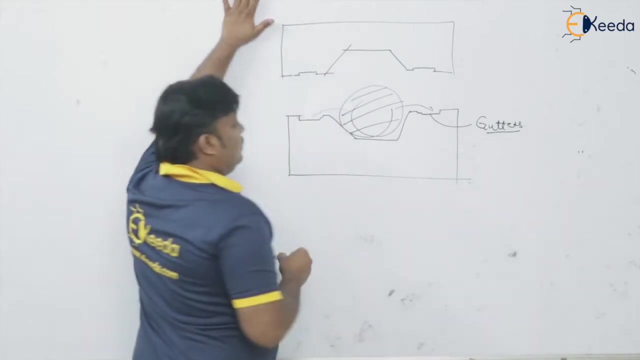 reason: see in the closed die forging we are providing the gutters. we are providing the gutters into the die so that after filling off the mold cavity by this material- billet material- this excess material will go and accommodate this gutters. these are the gutters which are provided in the closed die forging. 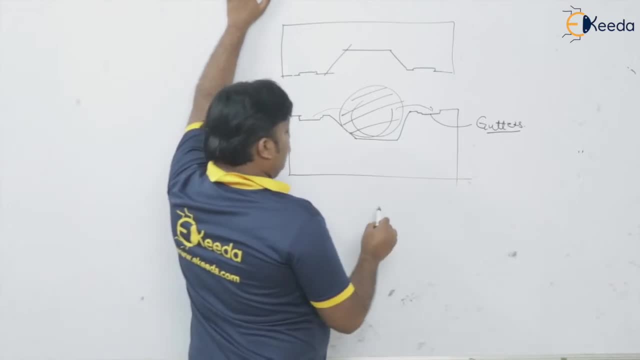 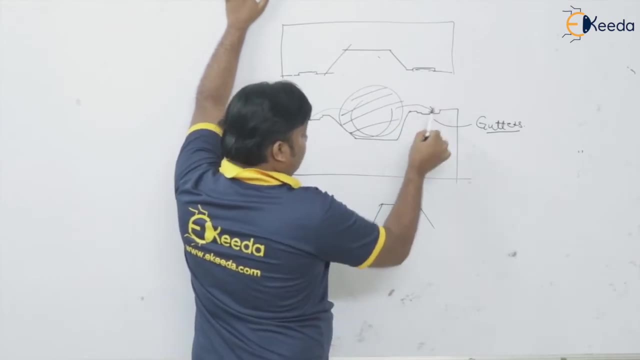 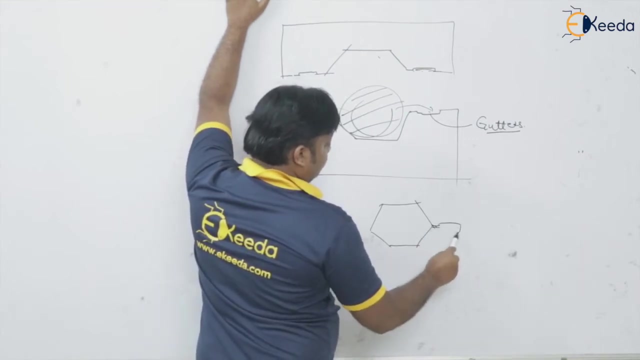 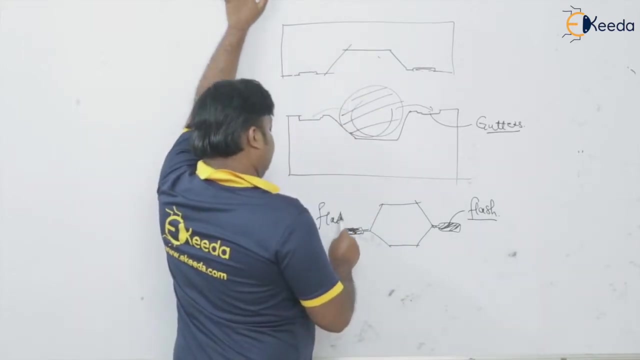 okay, and once the operation is over, once you get the product, so this extra material is going to fulfill into the product, it fulfill into the gutters and you will get the final product like this. okay, so this excess material will coming in the form of the flash. this is the flash, please remember. so this is the flash, and 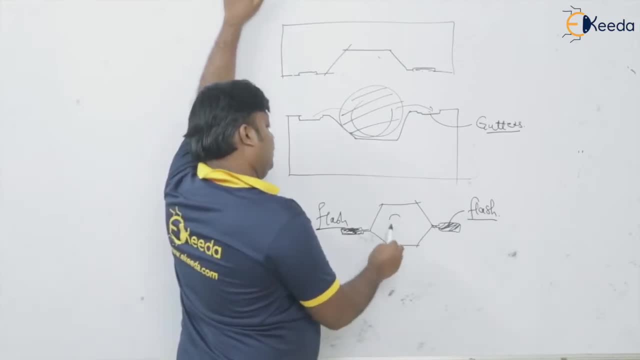 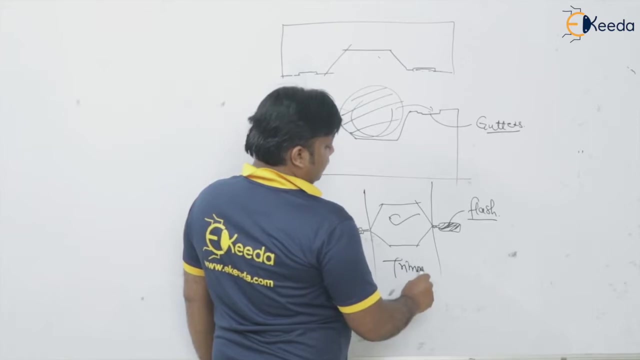 of course you want this final product, isn't it? so this is the unnecessary attachments to the main product. this in the form of flash. so this flash can be cut by the trimming operation. this flash can be cut by the trimming operation and you will get the required product. say: this is a 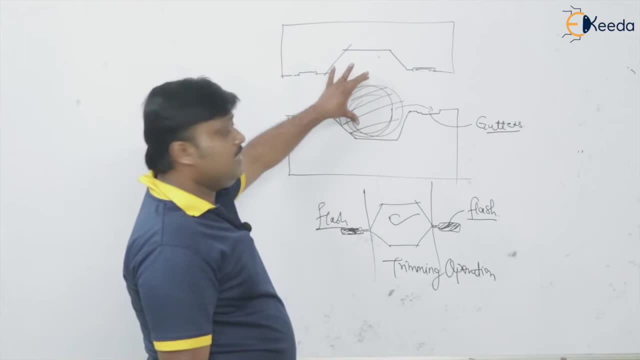 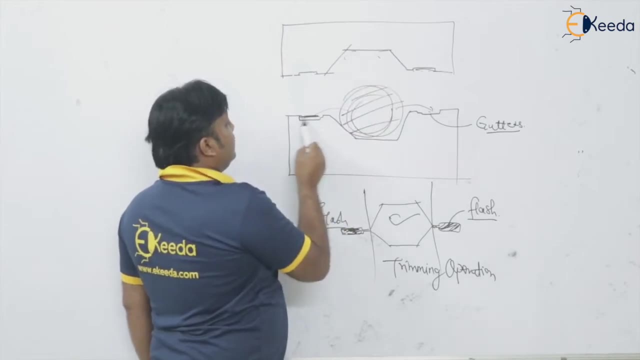 example of, say, coining, so pure, compressive stresses it. close diphorching operation. so after that you should like tiny comedään high meet, fazer se kr Walt compassion eh cse klose. the forging operation. so after making the impression that is available in the die, the excess material. 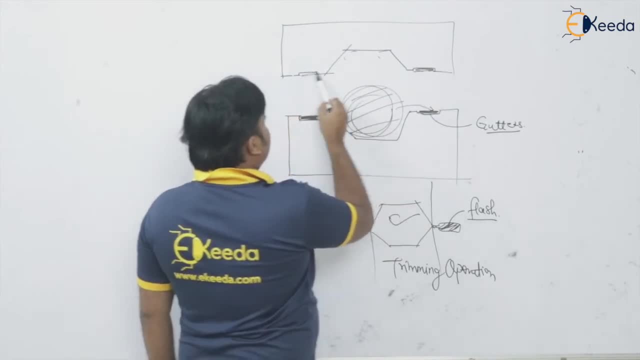 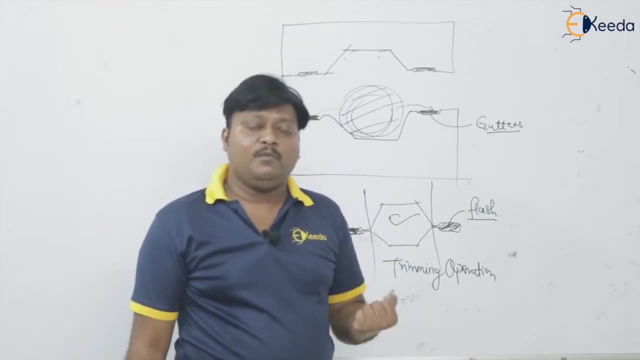 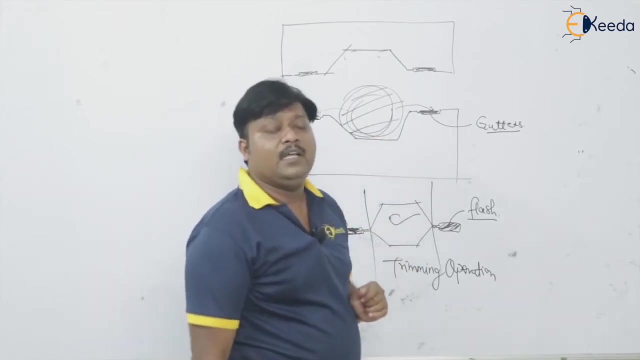 will go and accommodate the gutters and come in the form of flash. so that is the reason why the volume of raw material for the closed die forcing is 10 to 15 or up to 20 percent more than that of the volume of the final product. please, 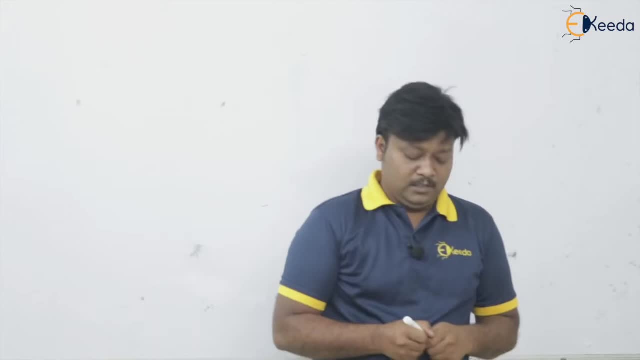 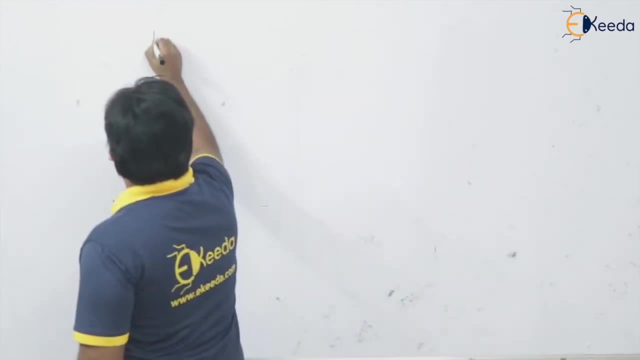 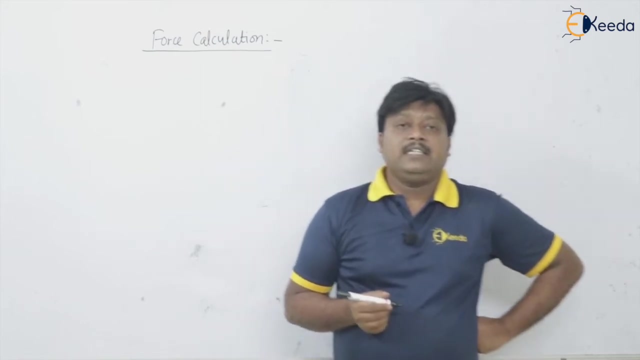 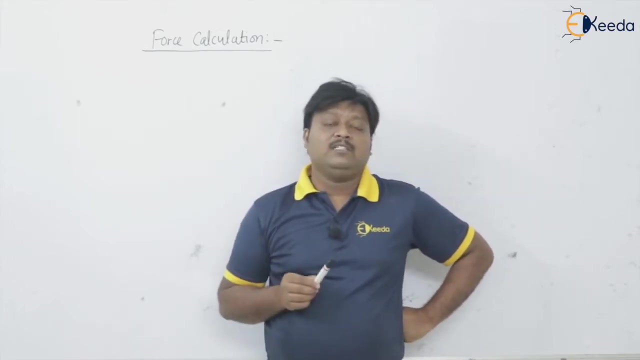 remember this. okay, dear students. now in this video we are going to see the force calculation for forging operation. the force calculation see. so if you look at the analysis of forging operation. so the analysis of the forging operation is basically done with the two models. one is the sticking friction model and the second 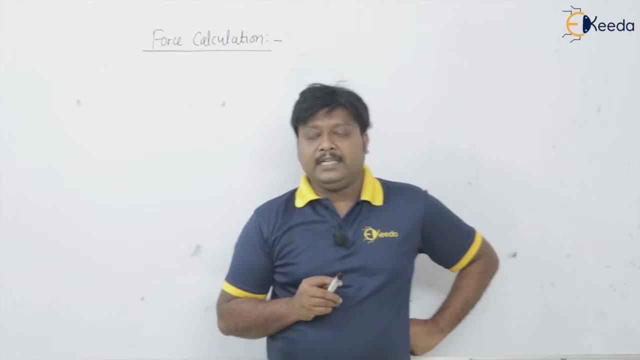 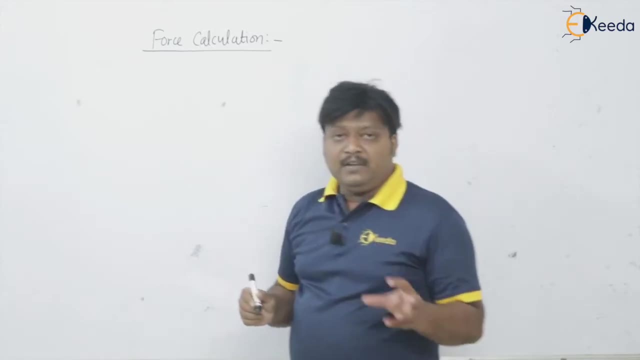 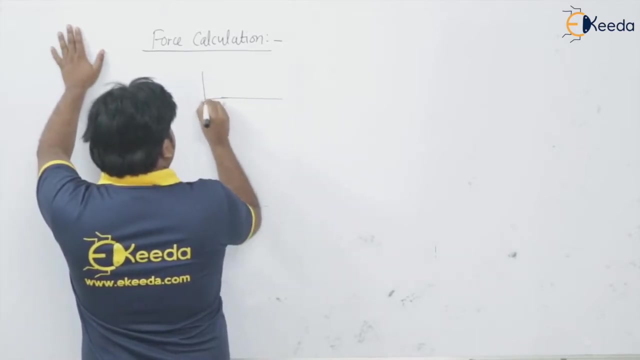 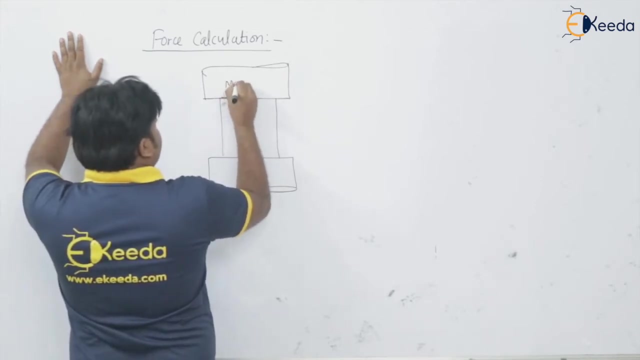 model is the sliding friction model. okay, so let us take for example- here I am taking this- the open die forging operation. so here say, this is the moving platter and the bottom die is the stationary platter. Okay, this is moving and this is stationary dies or Platter. this is the workplace. 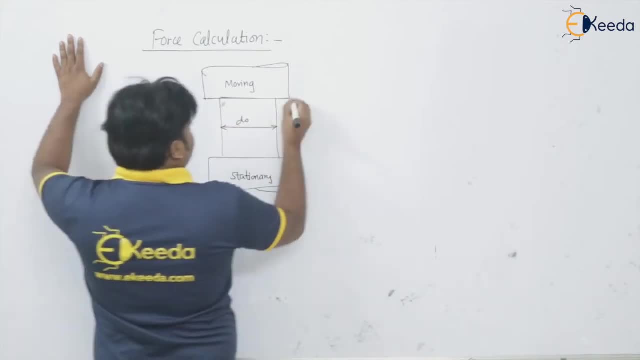 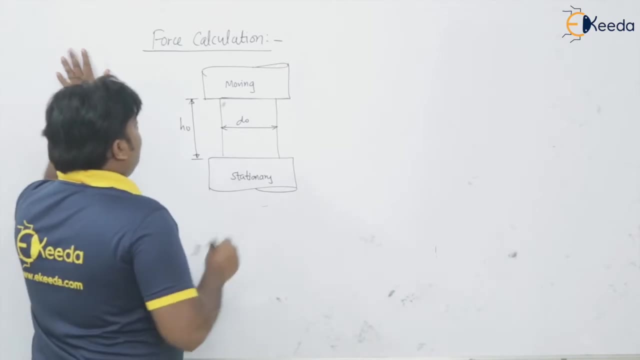 having original diameter, the original and the original height at edge origin. okay, when the force is applied by this moving platter on to this walls- and these must конечно mean that half of this is going to be at the- is the cylindrical billet, of course cylindrical billet, then what is going to happen? so, when it 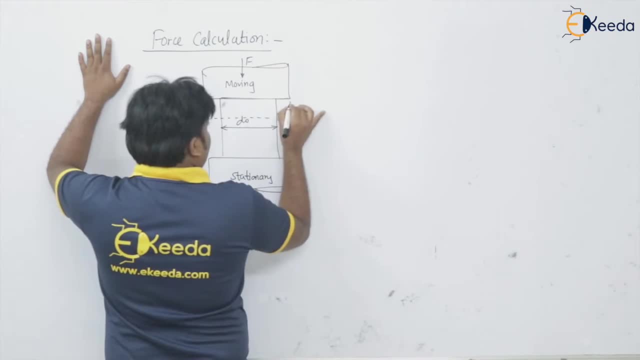 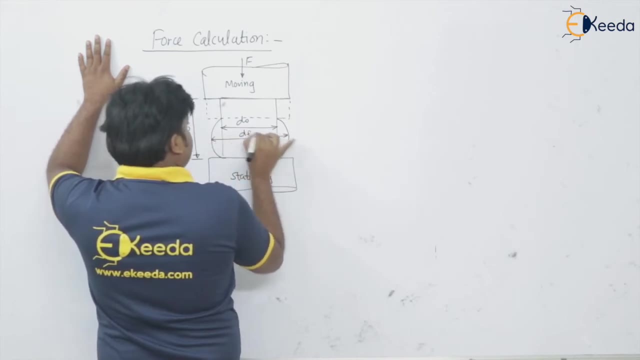 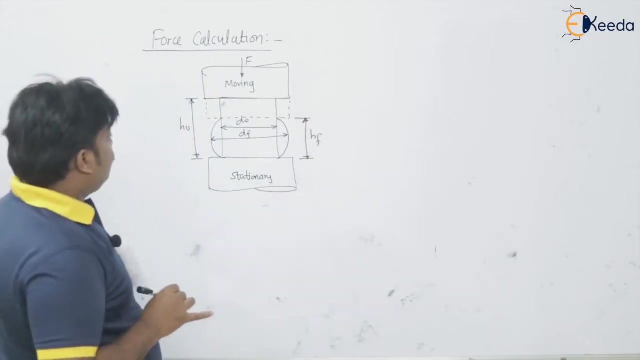 will come down. so there you will get the increase in diameter. this is the d final and the decrease in height. decrease in height. okay, so now, if you apply the volume constancy principle, of course volume constancy is valid in the metal forming operation, so i can write original area into. 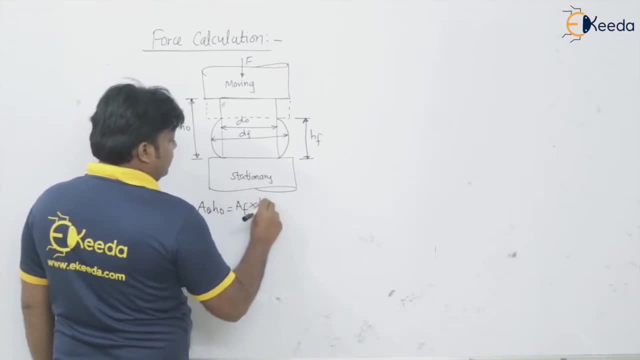 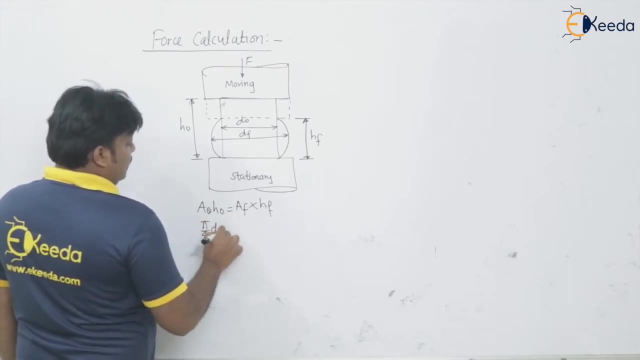 original height is equal to final area into final height. this is nothing. but the area into length is a volume. so original area is pi by 4. d original square into h. original is equal to pi by 4. d final square into h. final pi by 4. pi by 4 get cancelled, so the relation between the diameter. 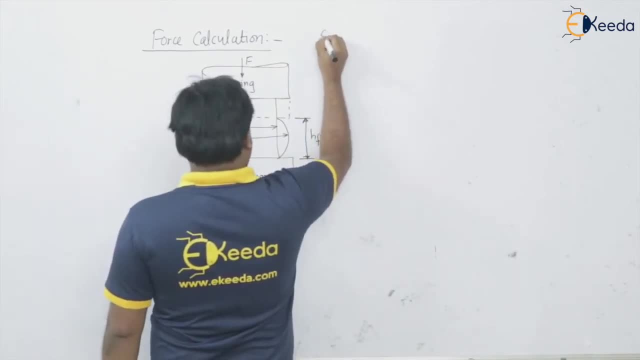 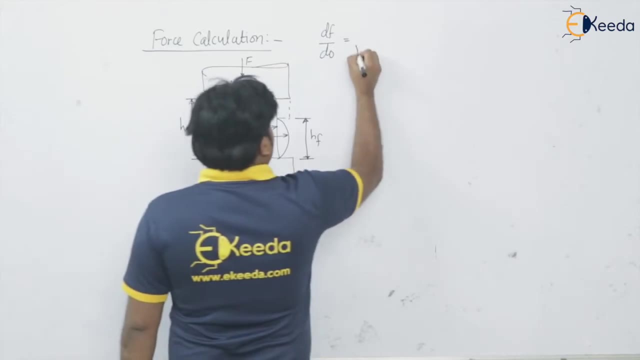 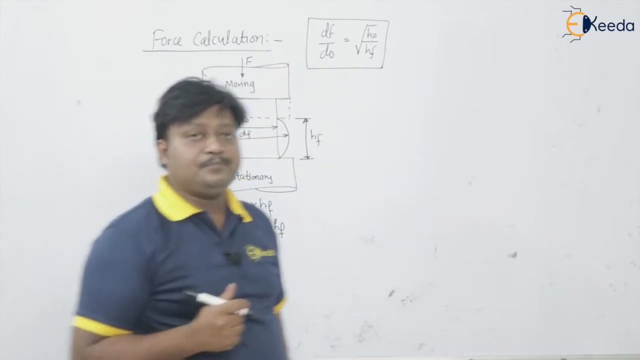 and the heights we are getting like this: that is d final divided by d original. i can write: d final divided by d original is equal to under a top, under root of h original upon h final. okay, so now basically see the main assumption for the forging force calculation, that the 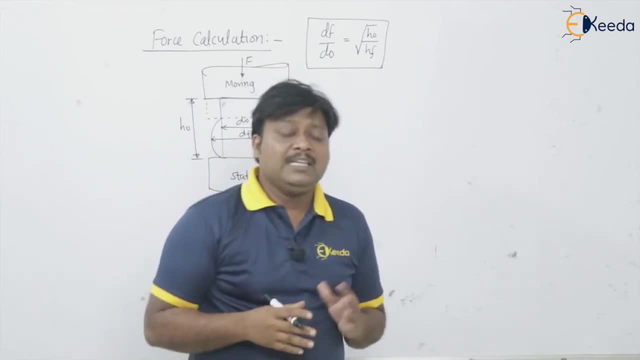 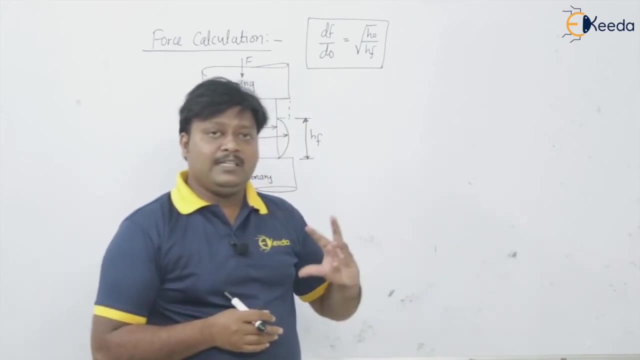 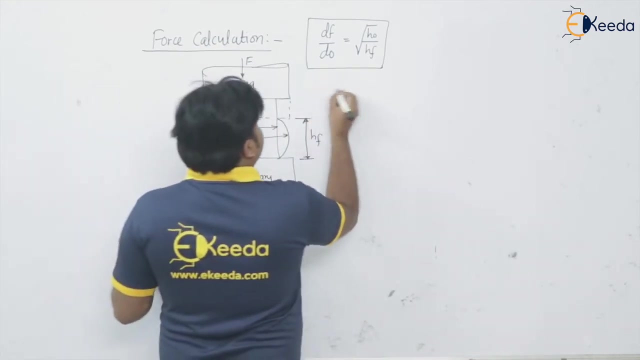 force in the forging operation is the maximum force at the end of the operation. please remember so: maximum force at the end of the operation or the at the end of the stroke here. okay, now here we have to find out the minimum initial force: f initial, of course, minimum. we are going to find how to calculate this minimum initial force that. 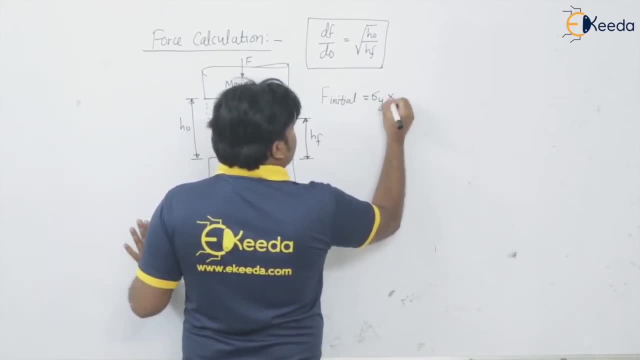 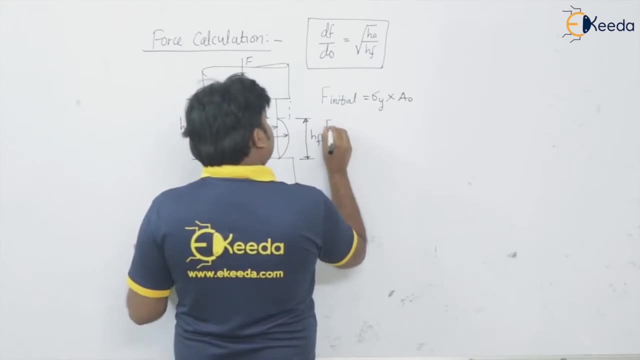 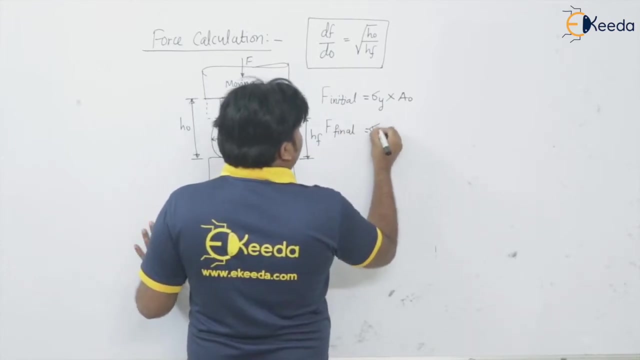 is the yield strength or simply you can say the flow strength of the material into original area. is that it? at the same time, if i want to have the final minimum area force, f initial, then f final minimum, then it should be sigma y into a final. and you know a original is pi by 4 d original square. 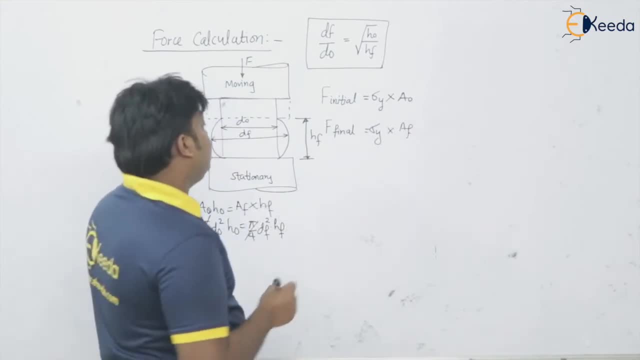 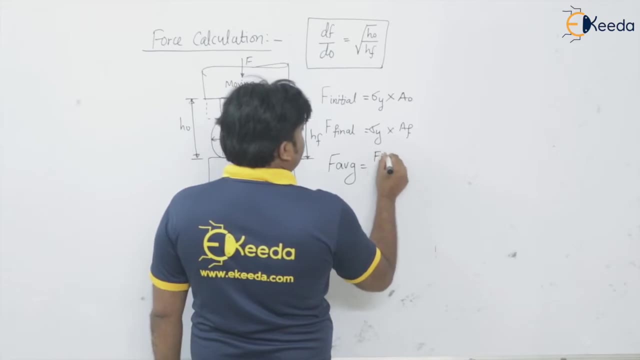 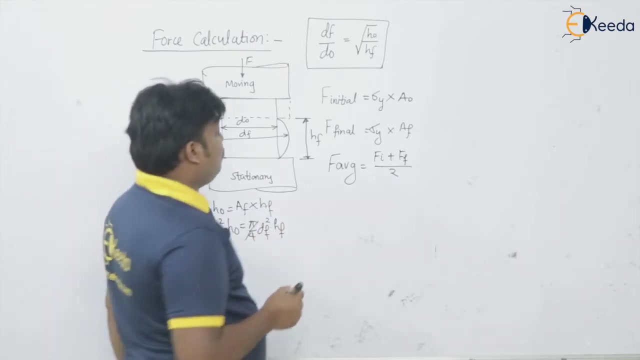 a final is pi by 4, d final square. once you get this two value, we are going to have the f average, that is, f initial minimum plus f final divided by 2.. now if the efficiency of forging given into the operation, general efficiency of forging, is how much? 0.5 to 0.6, that is, 50 to 60 percent. 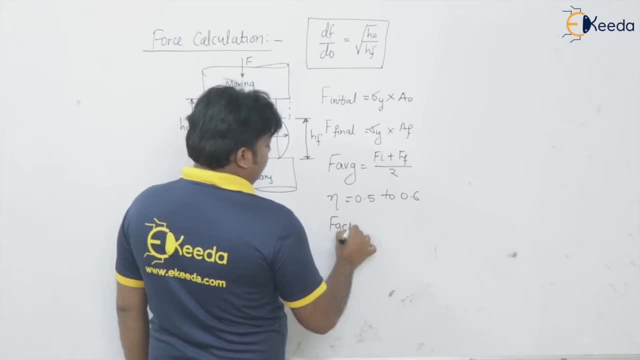 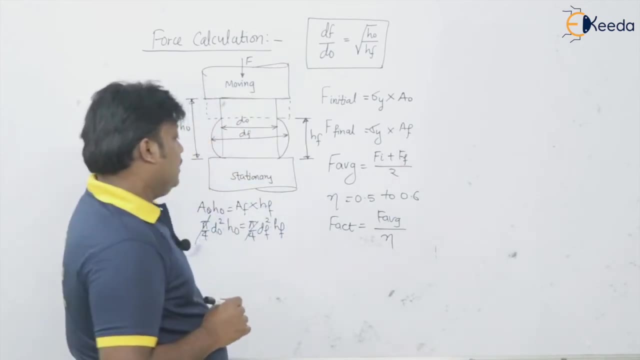 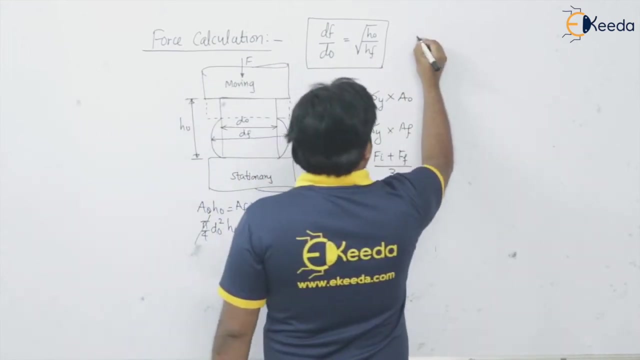 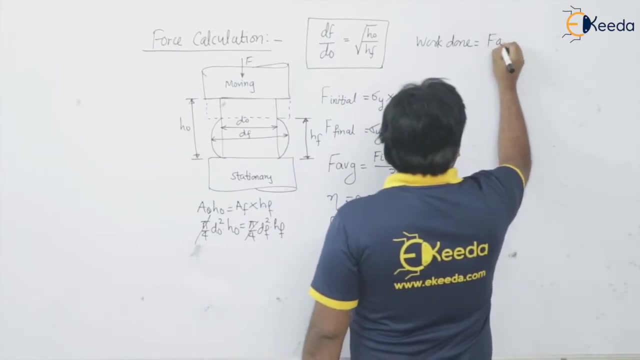 if it is given, then the f actual will be what this ef average divided by the efficiency of forging isn't it now? from here we got this full f actual and ahead of this, i want to find out the work done or energy required in this operation- forging operation- then it will be f actual into how much over 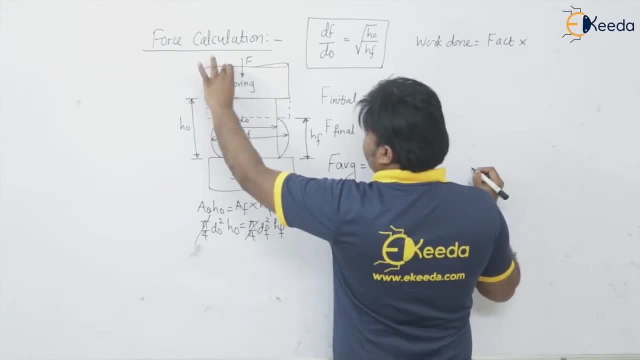 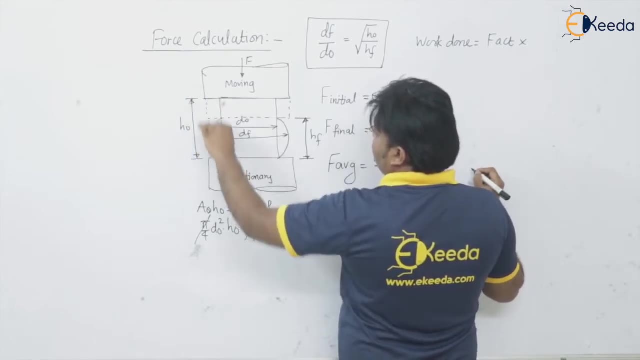 distance it is traveled. so a platen: yaha se, yaha aya, isn't it so? original height: it's not. and final height: h final, isn't it? so you get this distance. what is the displacement actually h or original, rather than the distance distance. what is the displacement actually h, original, and then the 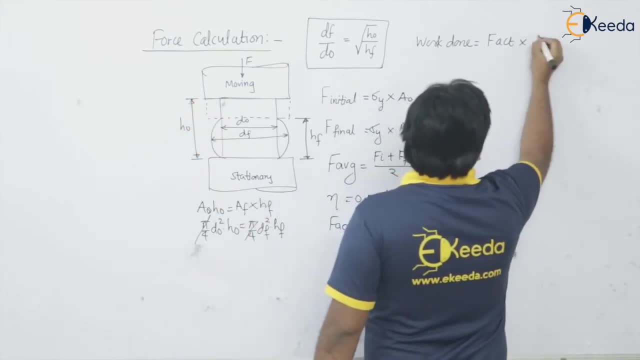 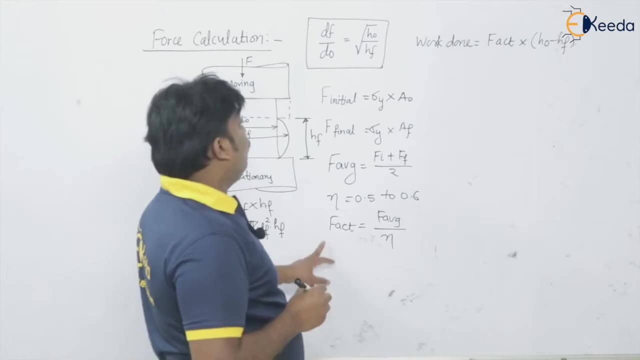 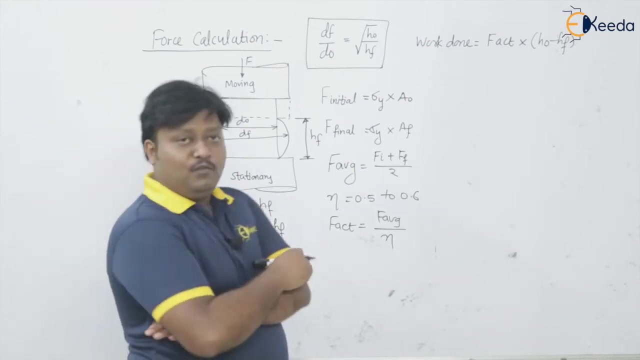 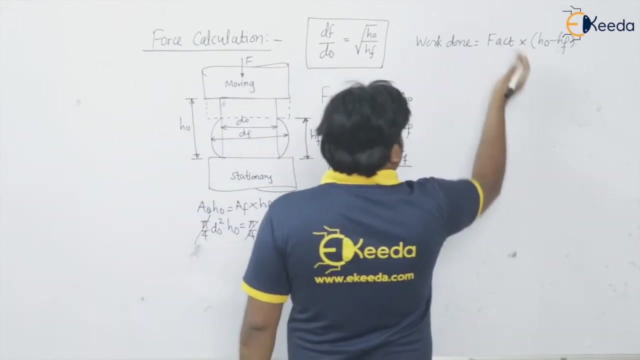 minus h final. that is, the displacement of the platen is a needle. that is h original minus h final. okay, so this is the force and the work done. now let us say if this forging operation and the drop forging operation- okay, having the same work done, support the same work done- is. 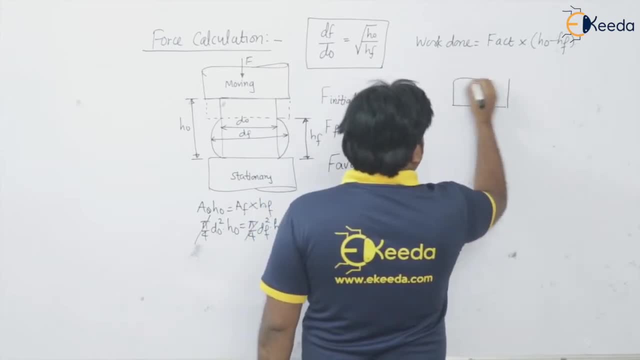 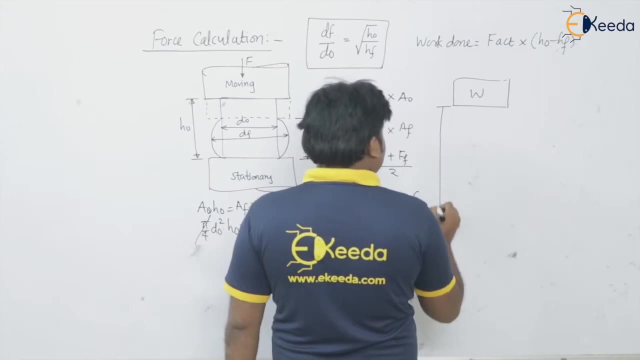 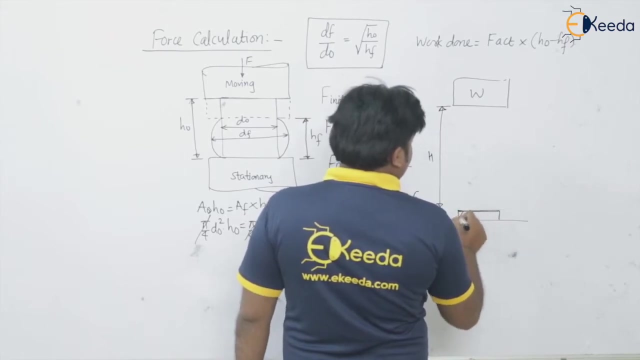 going to done in case of the drop forging operation. here is a weight of hammer. this is the hammer of weight w and it is freely falling from height h onto the workpiece on the say ground. okay, this is the workpiece to get the same amount of work done in case of this. 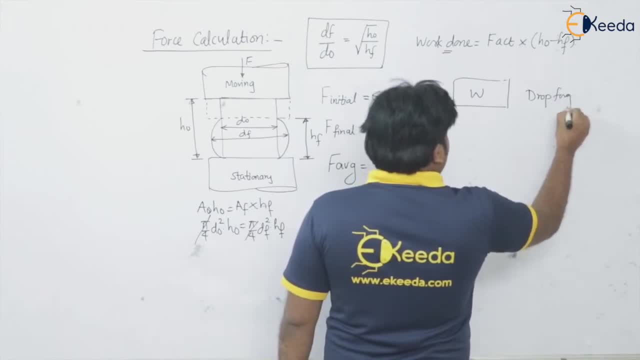 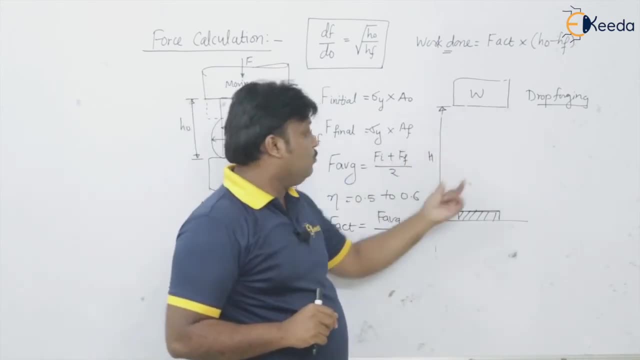 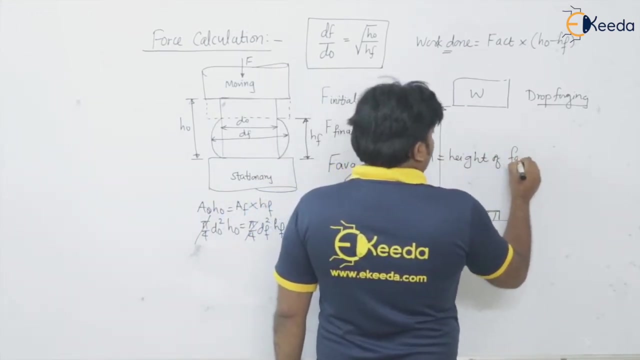 drop forging operation. how to calculate the height of fall of drop forging operation, this hammer, if the weight of hammer is known to you, how to how to calculate the this height of fall? so so here, what is going to happen in drop forging this? uh, potential energy gets stored by. 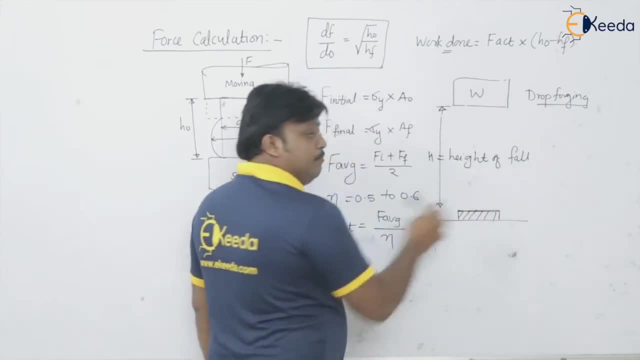 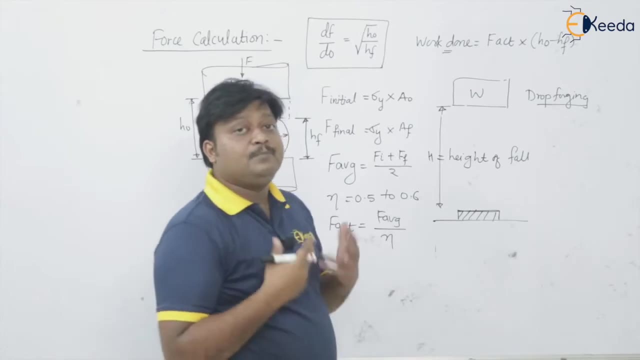 this hammer is converted into the impact energy, isn't it no? and we know that the impact energy is twice of the potential energy in case of the sudden loads. isn't it so for that? impact energy is twice of the potential energy in case of the sudden loads, isn't it so for that? 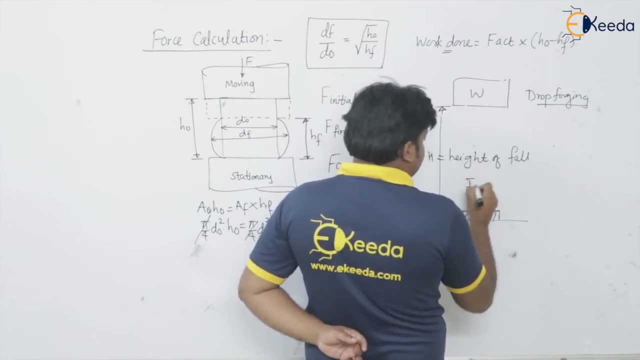 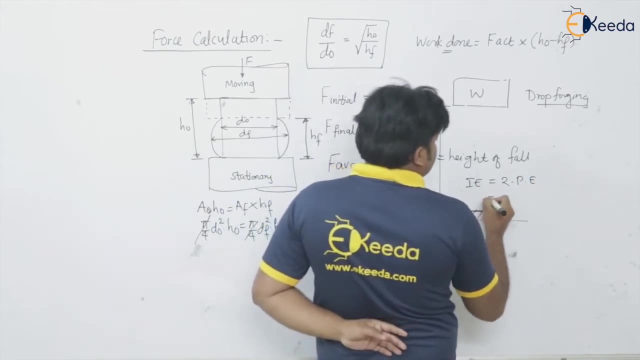 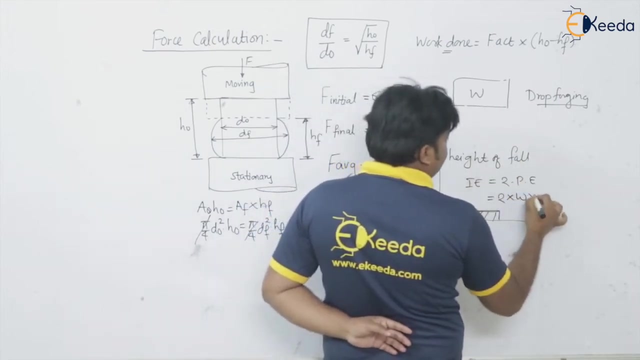 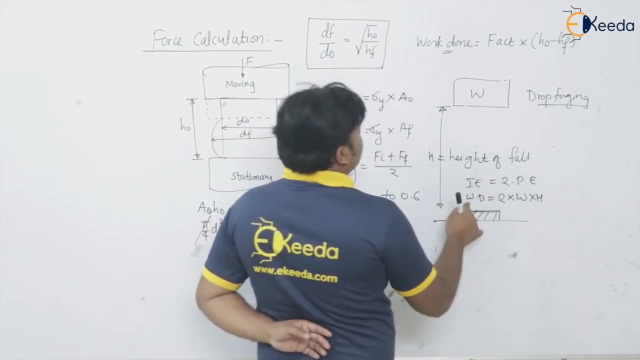 if i write the potential, the impact energy is equal to twice of potential energy. solid impact energy. it is nothing but two times. what is potential energy is w into h, w into h, isn't it? and this is impact energy. nothing but the work done, isn't it? and this work done we are having. 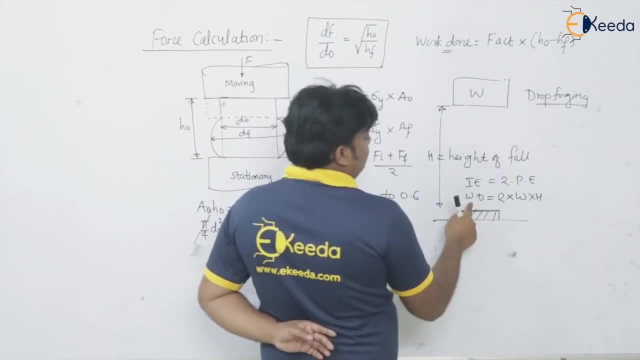 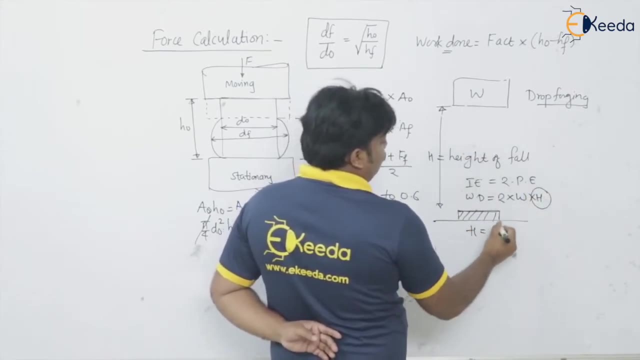 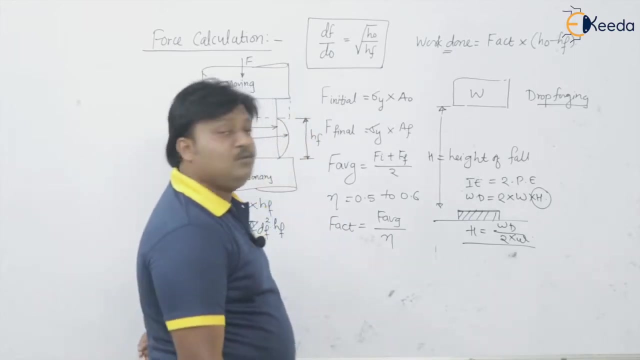 here we are getting from this equation, and if you put here this work done, you put here the value of this weight of the hammer, w, you will get the height of fall that h will be equal to this work done divided by two times w. okay, so in that fashion we can also able. 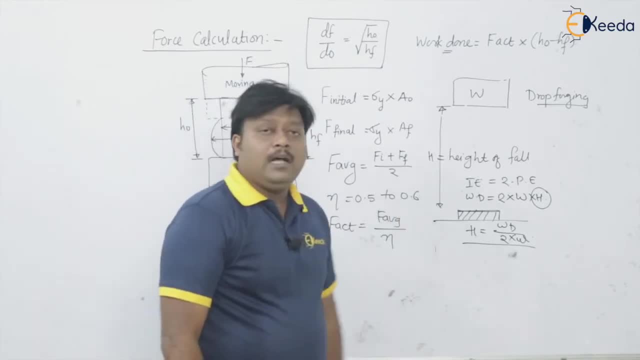 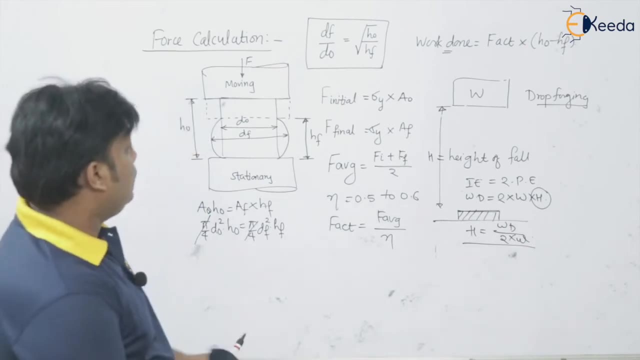 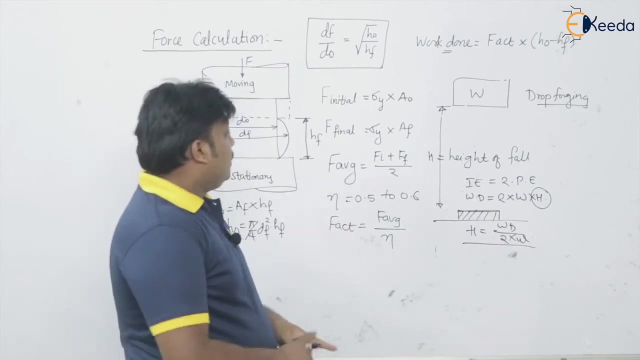 to calculate the height of fall in the drop forging operation. okay, so this is the actually methodology to form the force, but here, uh, nowhere in this uh discussion, we have talked about the coefficient of friction. okay, so when the coefficient of friction is given into the equation, please remember that this force actual. 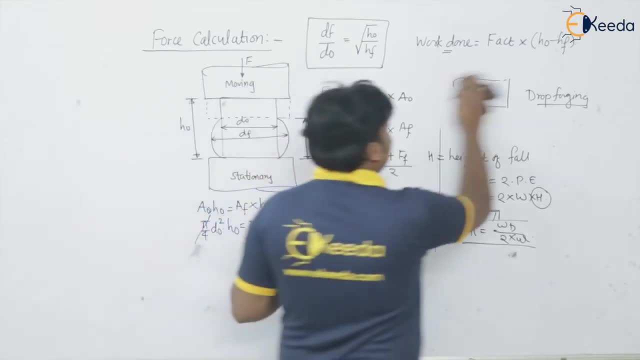 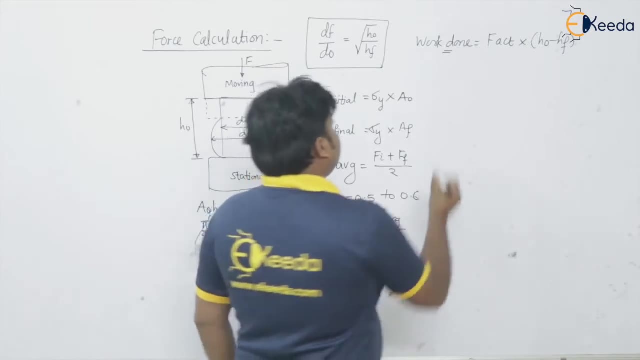 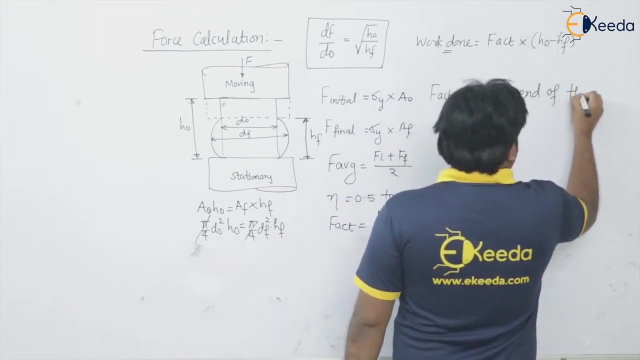 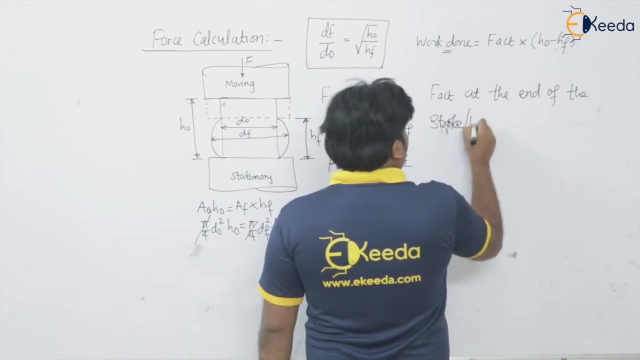 force is basically given as this f actual. we can have directly f actual force forging at the end of the operation or at the end of the stroke. f actual at the end of the stroke or blow, or stage end of the stroke or blow. that is f actual is. 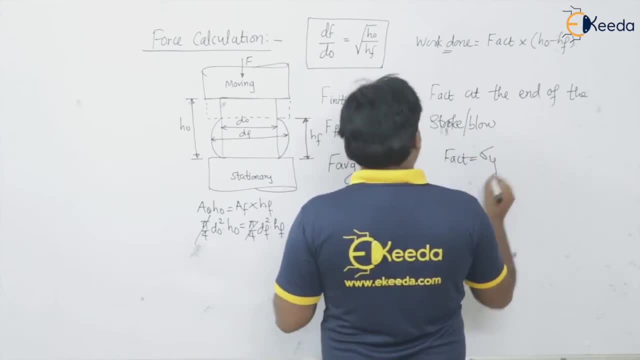 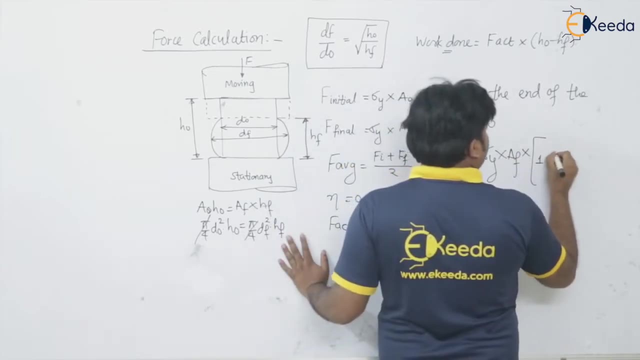 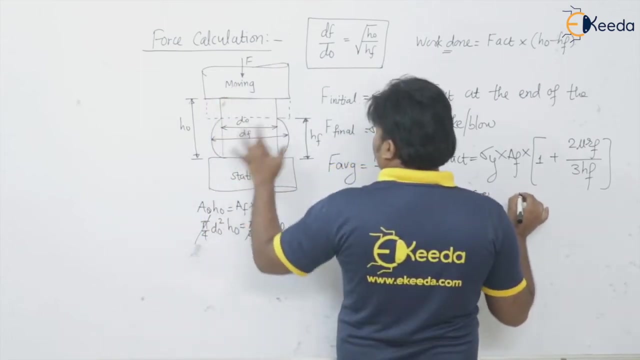 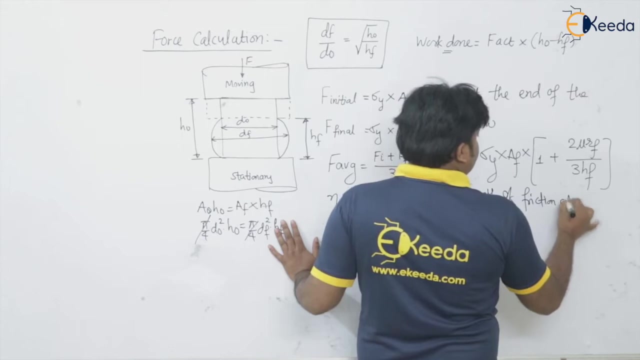 given by this Sigma y into final cross-sectional area, but when the friction is there, it is given as into 1 plus 2 mu R f divided by 3 times hf, where mu is a coefficient of friction at the die and material interface or billet material interface coefficient of friction at die and workpiece interface. 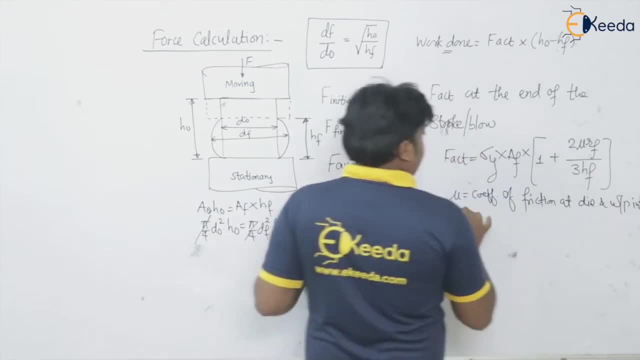 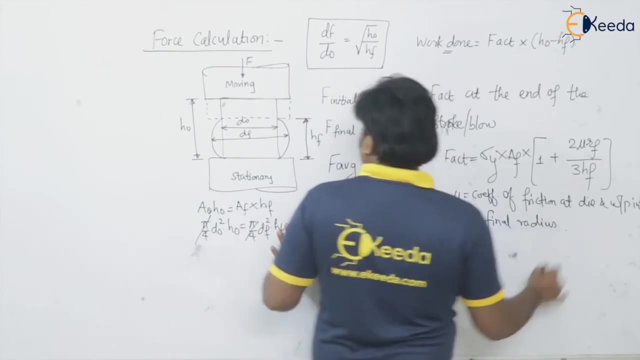 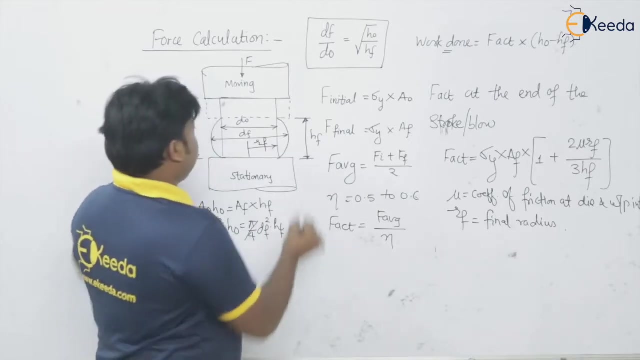 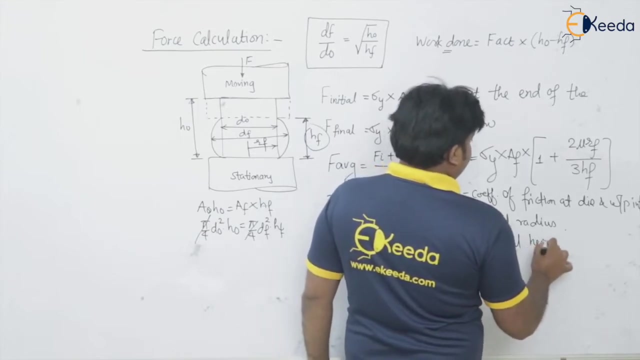 and rf is the final radius of the workpiece. what is final radius? this is the rf, that is df by 2. that is the rf. and hf is this final height and hf is the final height. so this is the actual force at the end of the stroke. we can get directly from this formula. 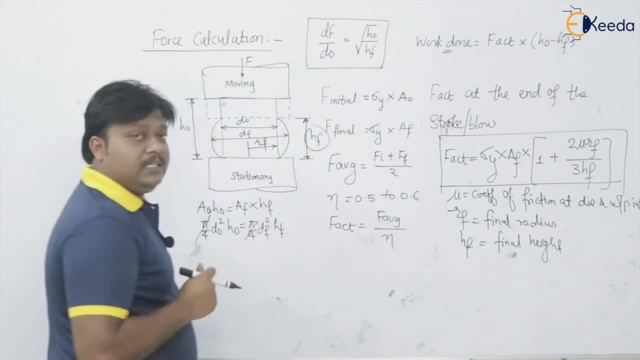 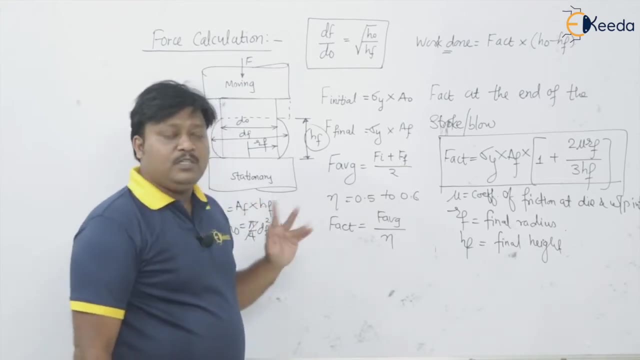 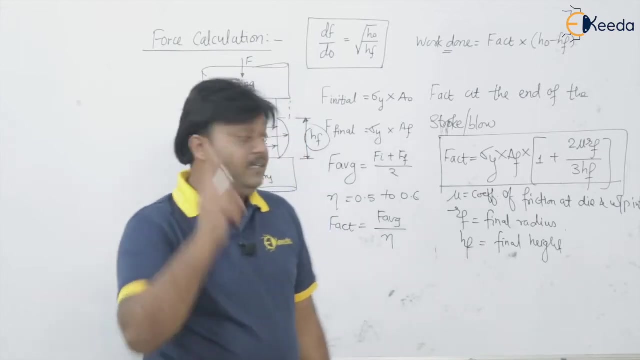 ah, no, not we can able to derive it, but no need here. as far as gate examination is concerned, try to have the formulas, whichever we have explained in the class. no need for the derivation. okay, so f actual. here you can calculate when, when, when, the coefficient of friction is given to you and 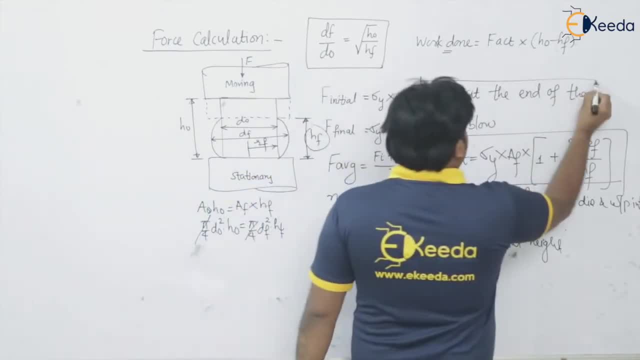 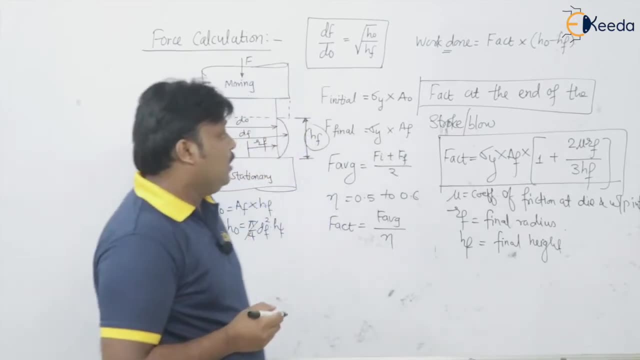 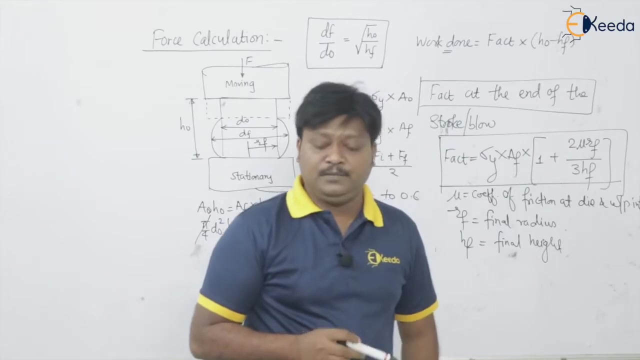 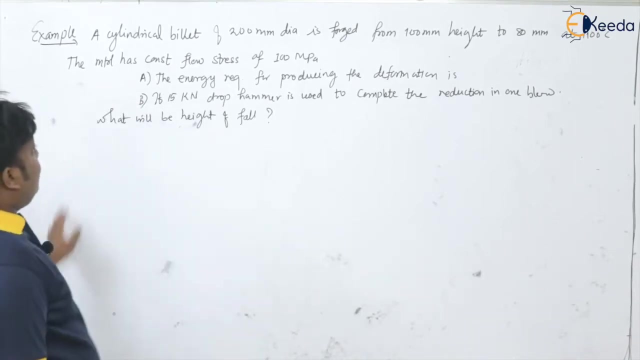 asking for what they will ask: find the actual force at the end of the stroke or end of the operation or at the end of the, the, the. so this is how we can able to calculate the force in the forging operation. so let us see this example: on the forging, a cylindrical billet of 200 millimeter diameter is forced from 100 mm height. 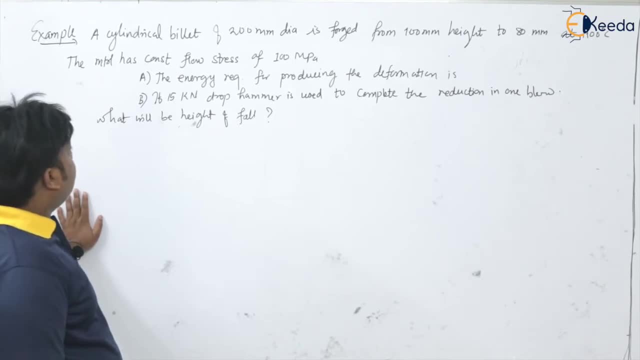 to 80 mm at 1100 degree centigrade. the material has the constant flow stress of 100 megapascal. so number one, we have to find out the energy required for producing the deformation, and the second bit is if 15 kilo newton drop hammer is used to complete the reduction in one blow. 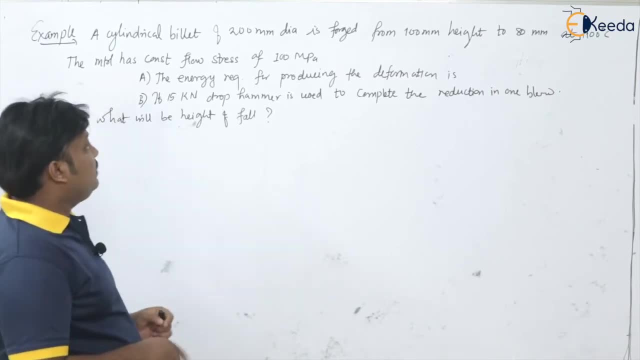 what will be the height of fall. so we discussed already how to calculate the work done and the height of fall. so let us see: the initial diameter is 200 meter and the depth of fall will be 200 meter and from the height, original height, say 100 millimeter, to the final height, 80. 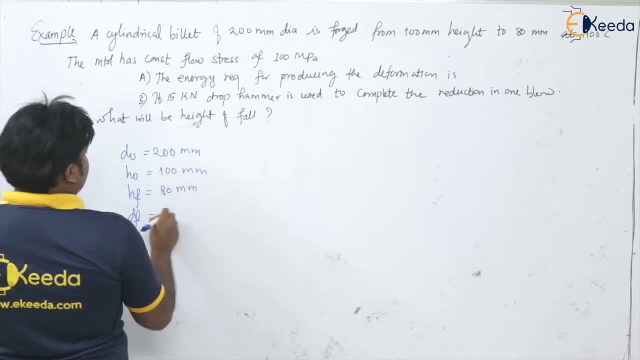 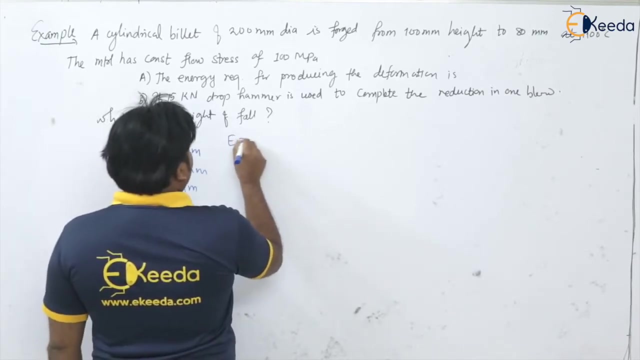 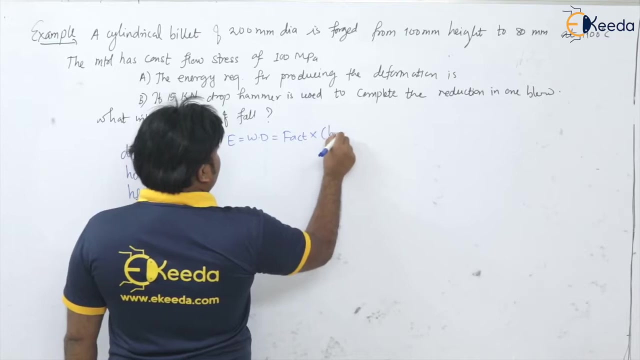 millimeter, isn't it? so final diameter is not available with us that we will see how much the Sigma flow or Sigma Y is given as 100 mega Pascal. okay, we know that how to calculate the energy or work done in the forging operation is equal to this: F actual into H original minus H final. we know this. so first of all, to 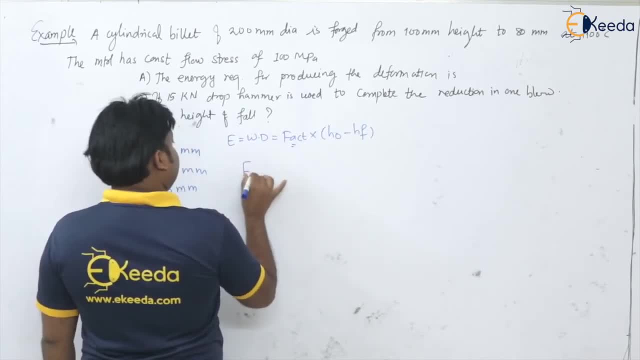 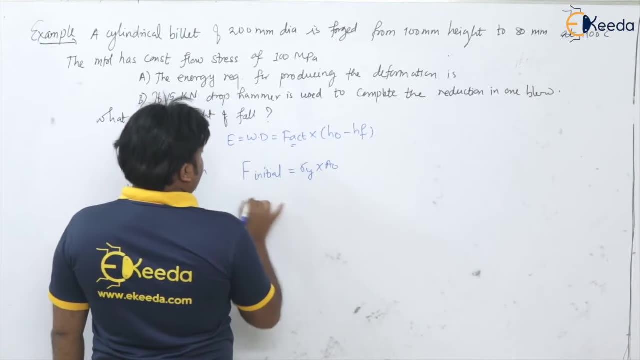 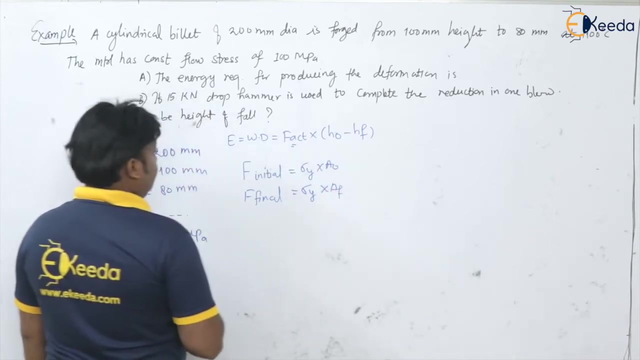 calculate the F actual, we need to calculate EF initial minimum that is Sigma Y into a original and we have final minimum- it is Sigma Y into final cross-sectional area. so for that we required final diameter in the form of sigma Y into a original and in the form of sigma Y into final. 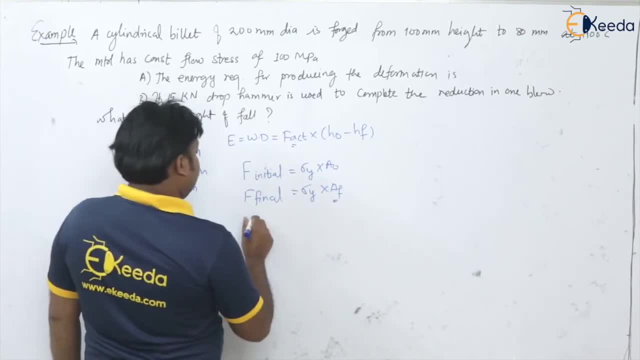 isn't it? so by having the continuity equation, A naught into H naught is equal to AF into HF. so what you got here, pi by 4 DO square into HO, is equal to pi by 4 DF square. pi by 4, pi by 4. 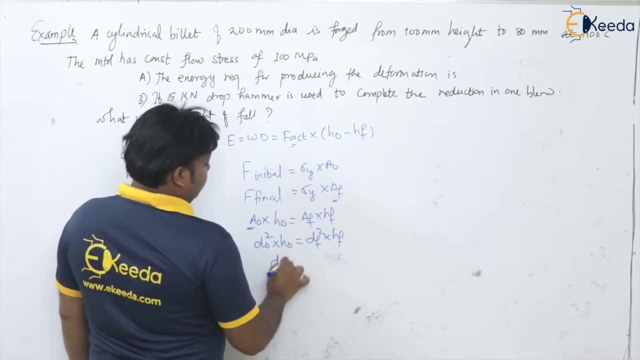 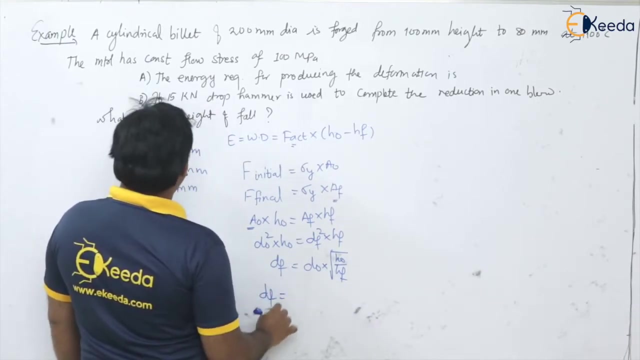 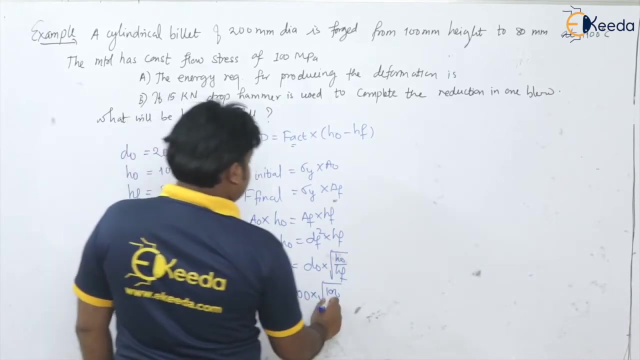 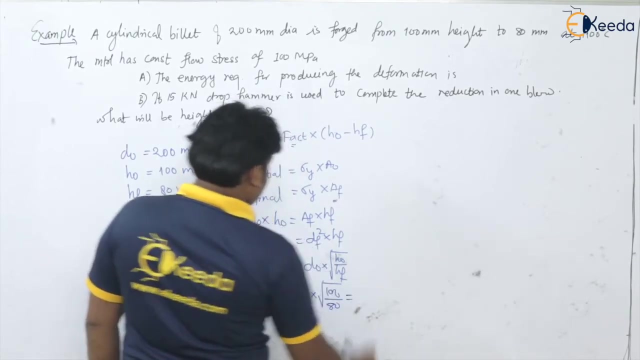 get cancels into HF. so DF will be what DF will be DO into root of HO by HF, isn't it put the values: DF is equal to original diameter 200- into root of H- original 100, so so, and H final is how much 80. so what will be the final diameter? 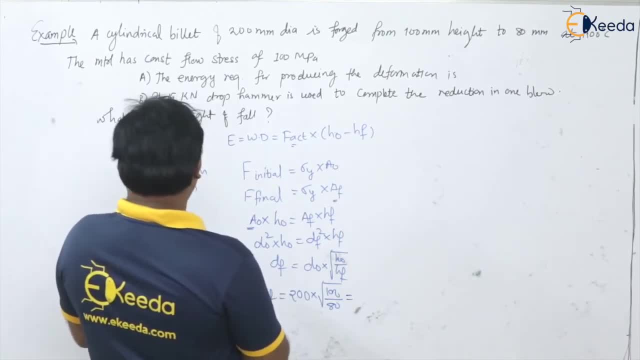 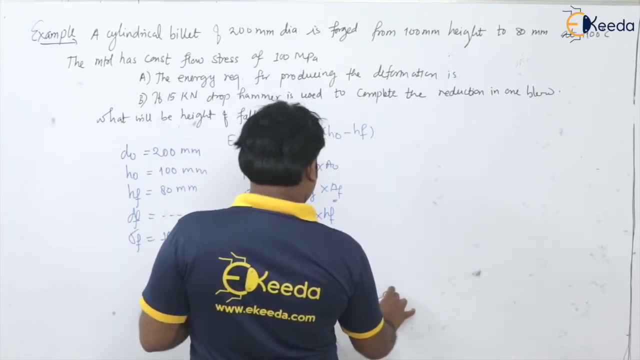 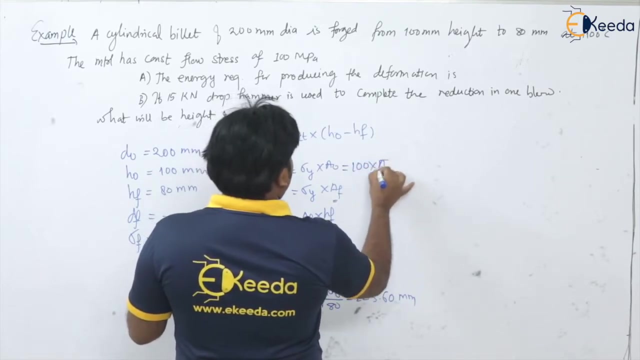 100 divided by 80, root of the answer into 200, so it is 223 223.60 millimeter. okay, so we got the final diameter by the volume constancy. now here, what is here finisher minimum Sigma, flow or Sigma? why is how much hundred into a original debit? 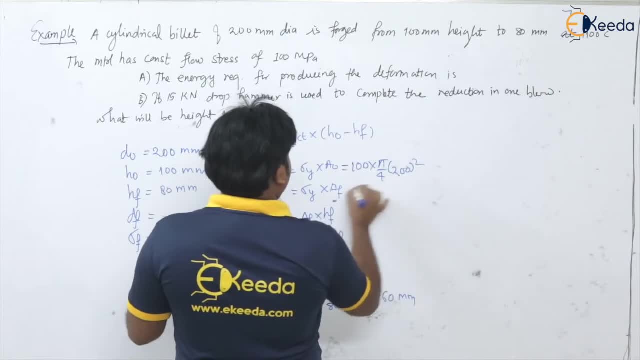 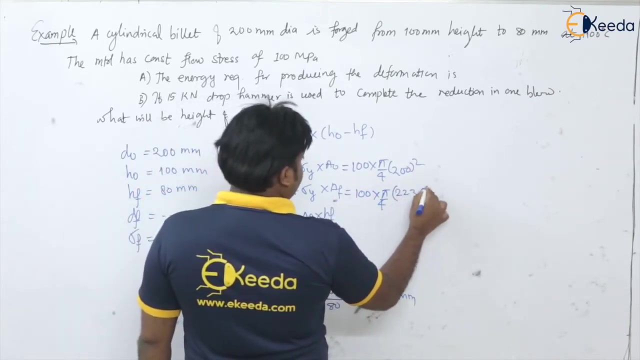 for the original, that is 200 whole square and Sigma, sorry, add force minimum, at the final stage it will be hundred into pi by four, 93, final stage confrontation. also these point six. so that means the diameter is equal to pi by four D. how muchров prime steps kimaya by four, that is two hundred, and into AP of 4 D, original, that is 200 whole square and the sigma, sorry, at force minimum and at the final sex it will be hundred of più pi, if I've. or how much diameter is the final? say Gayat also, it is 0.69 square. 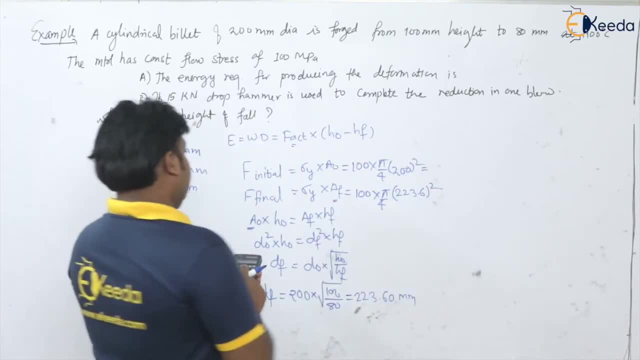 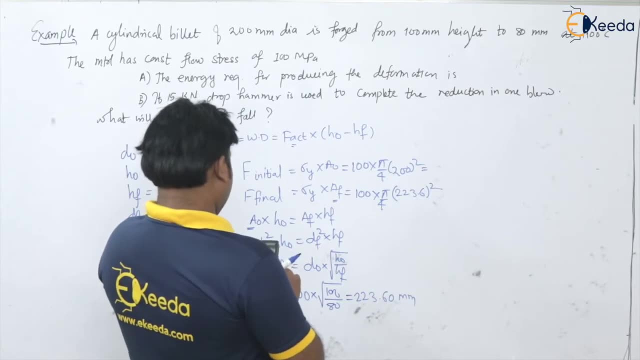 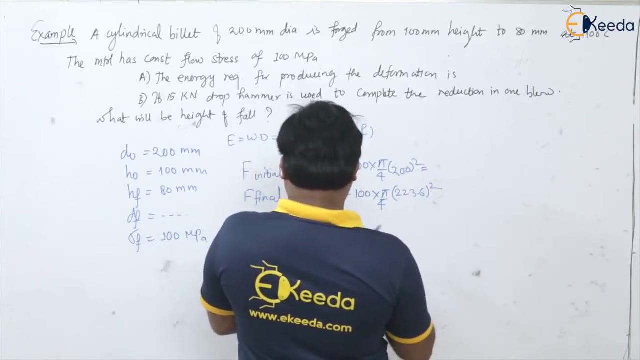 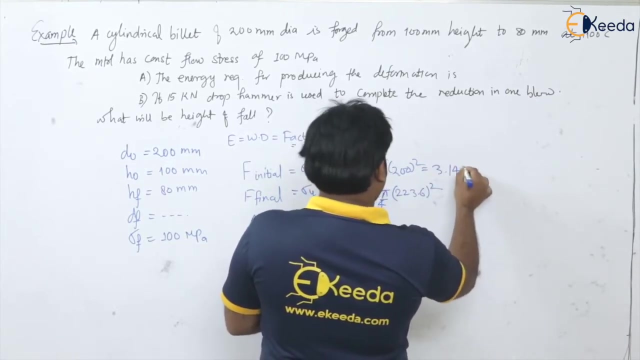 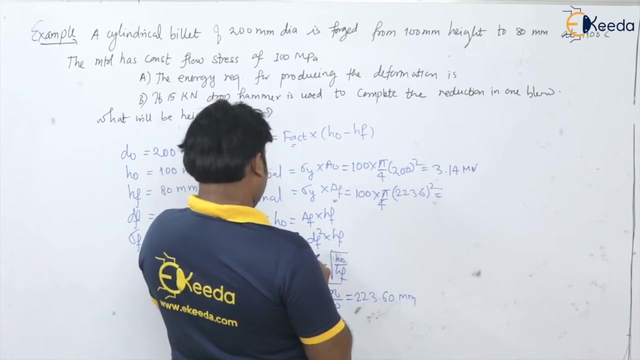 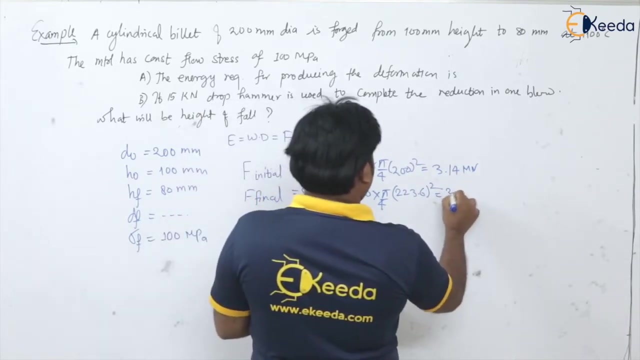 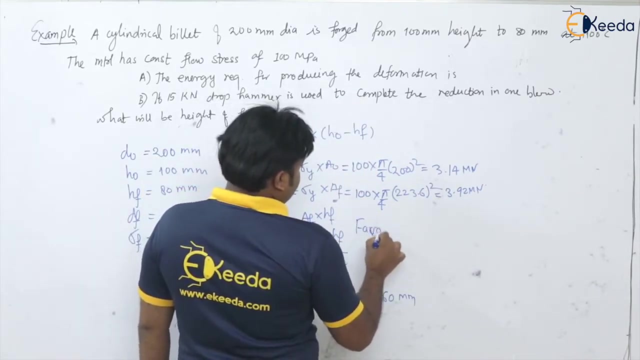 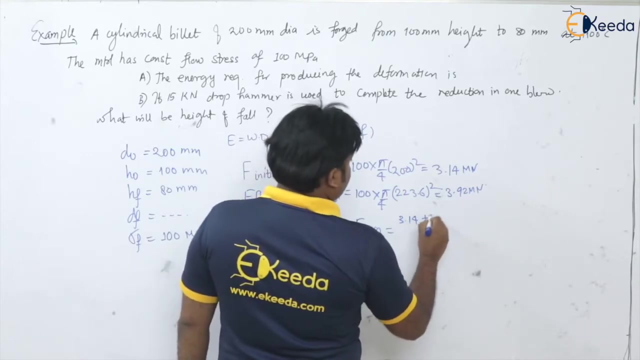 So get the values: 200 square into 200, square into 25 pi. It is in kilo Newton I am writing, or it is mega Newton, 3.14 mega Newton, and it is 223.6.. Square into 25 pi, So it is 3.92, 3.92 mega. Now, if you have the average value, it will be this: F initial plus F final, minimum divided by 2, that is, 3.14 plus 3.92 divided by 2.. 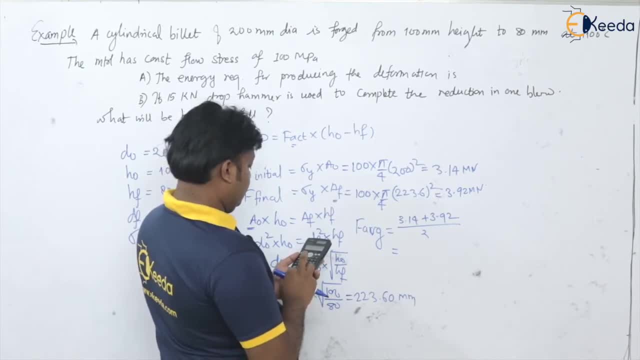 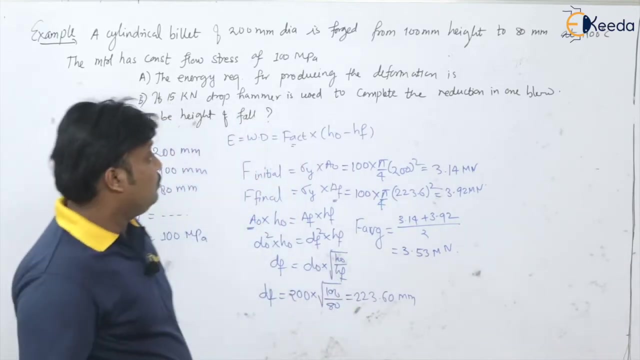 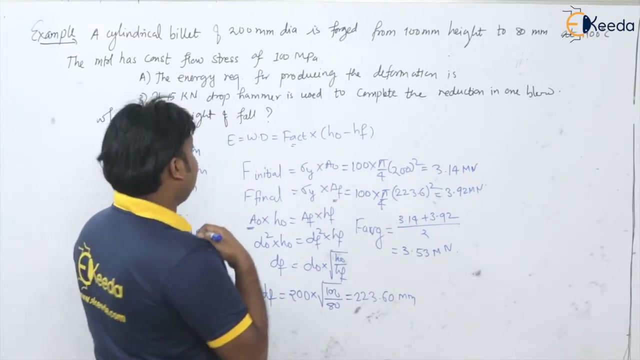 So plus 3.14 into the power 6 divided by 2. So the average value will be 3.53 mega Newton. Okay, So once you get this force, average force efficiency is not given, So we take directly force here. 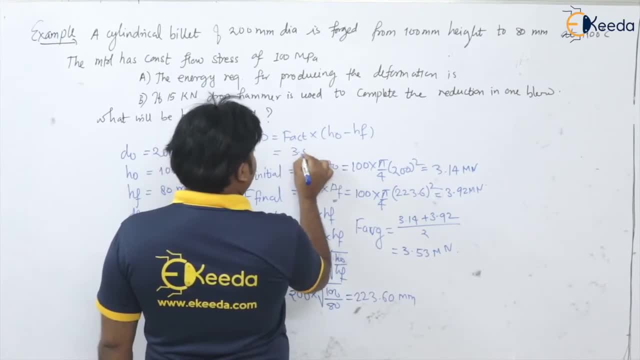 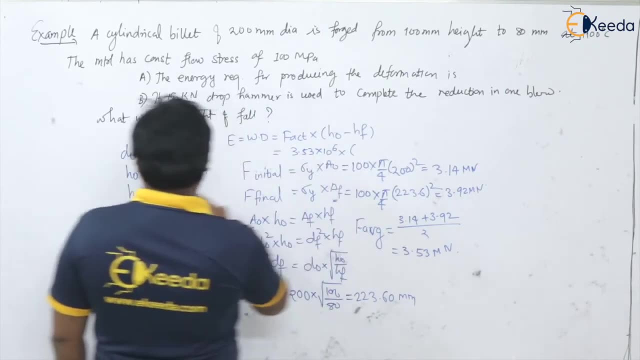 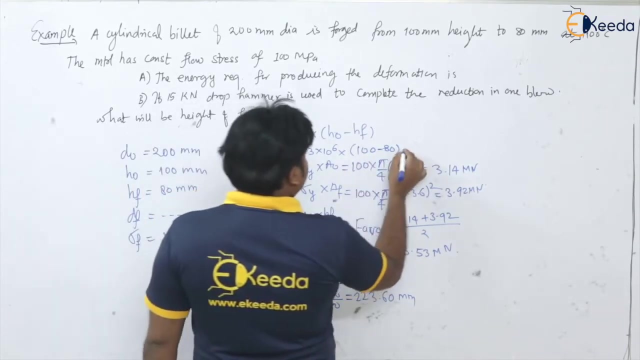 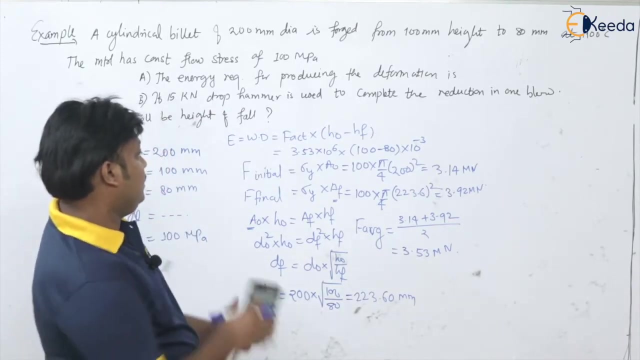 That is F. actually is 3.53 into 10 to the power 6.. 10 to the power 6 into the original height was 100 millimeter, minus final height, 80 millimeter, So it is millimeter. So convert it into meter into 10 to the power minus 3.. Isn't it So how much? 3.53 into 10 to the power 6 into 20 into the power minus 3.. 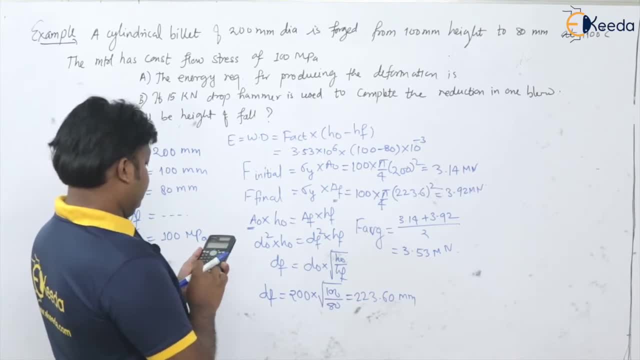 So how much? 3.53 into 10 to the power 6 into 20, into the power minus 3 meter, into again 4, into 2 minus 3.. M2 e to the power 7 죽. So this two particles are equal in number. 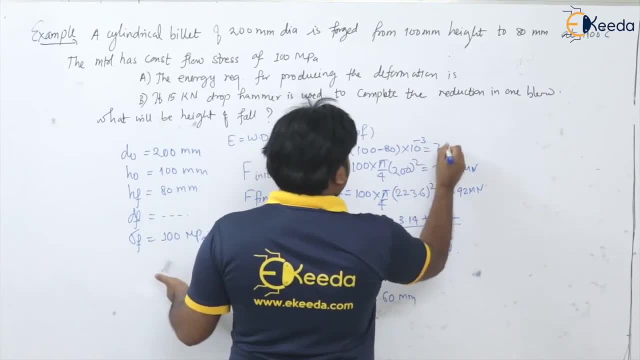 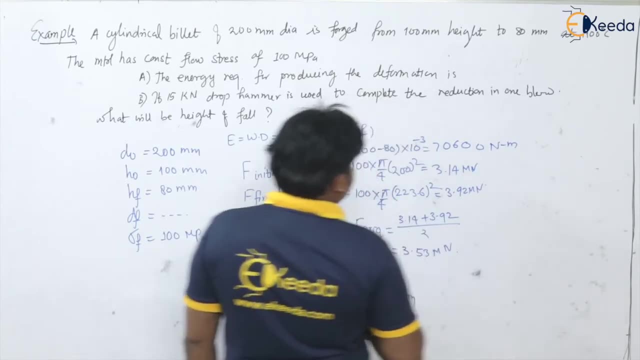 If there are two particles, you can write it as equal to the exact momentum of thiserdนนah number. So what is the unknown Ruslansee? so do Newton meter, isn't it? or it is 70.6 kilo Newton meter. so, after having this work, 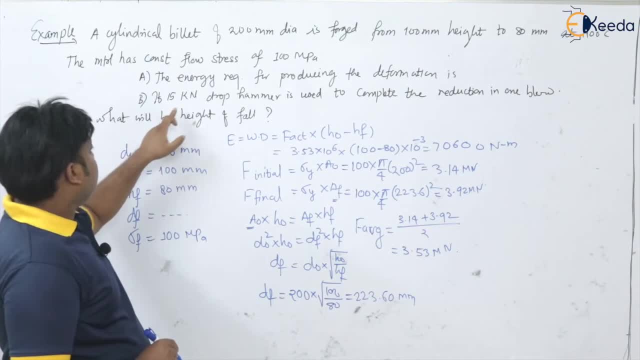 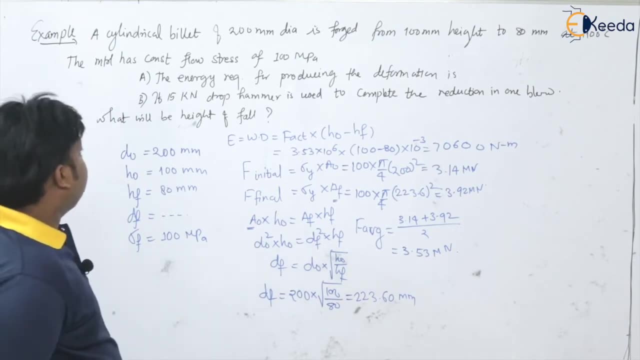 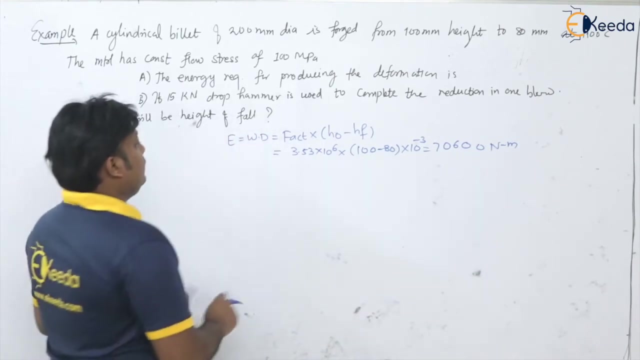 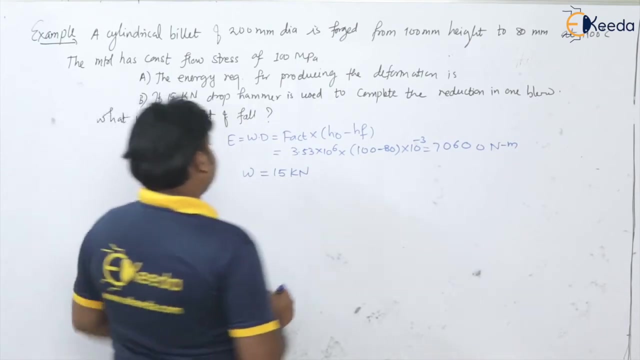 done, calculation. what is the next question they are asking? if the 15 kilo Newton drop hammer is used to complete the reduction in one blow, what will be the height of fall? okay, now see the drop hammer weight. the weight of drop drop hammer is how much? 15 kilo Newton, isn't it? and what is work done in the case of? 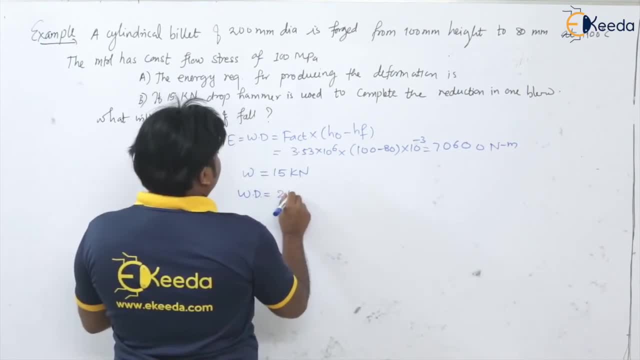 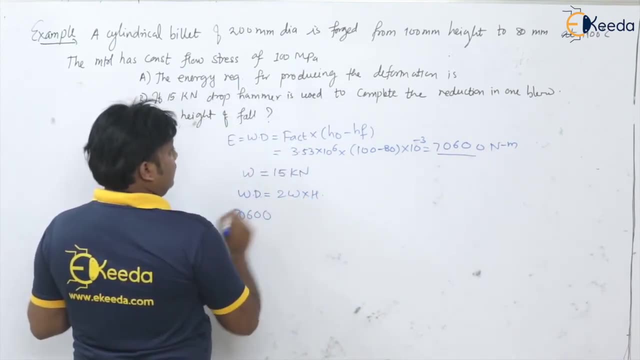 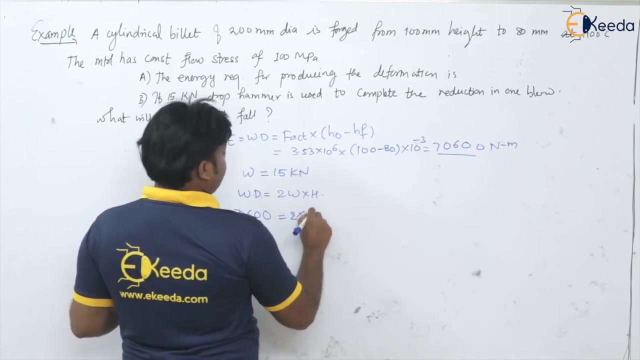 drop forging. we know that it is 2 times W into H. so how much work done. we got here: 7, 0, 6 0, 0. this is in a single stroke. then it will be 2 times weight of the hammer is 15 into 10 to the power 3 Newton. 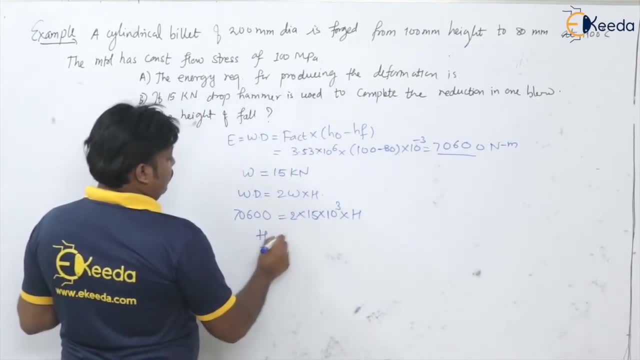 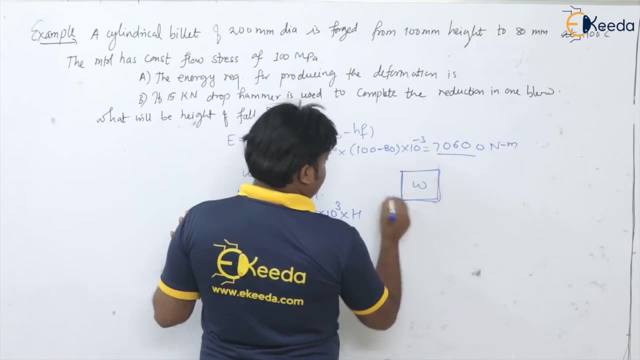 into H. so if you calculate the height of fall, say this is the weight hammer of the weight of the hammer and it is falling from this must hide on to the work piece to produce the work done off 7, 0, 6, 0, 0 Newton meter. so how much it is? 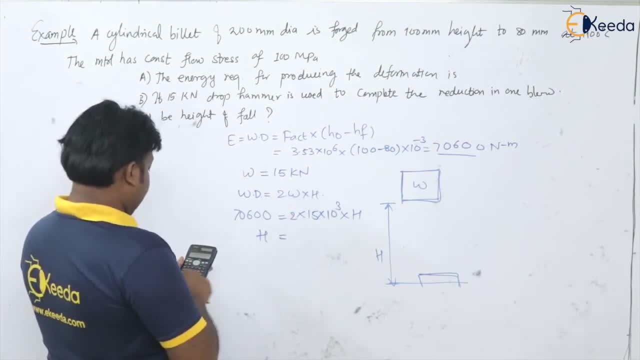 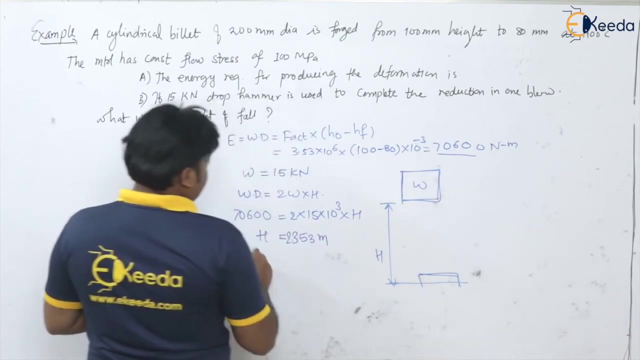 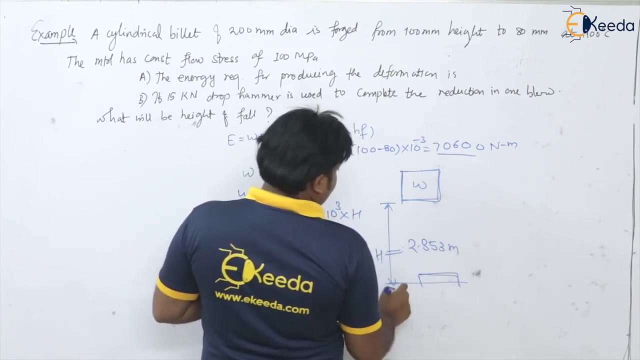 7 6 0 0, 7 0 6 0 0 divided by 30,000, it is two point three, five. two point three, five three. it is two point three, five three. and this height: two point three, five three. through this. 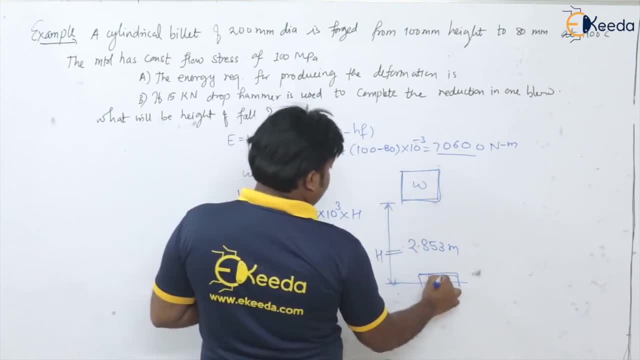 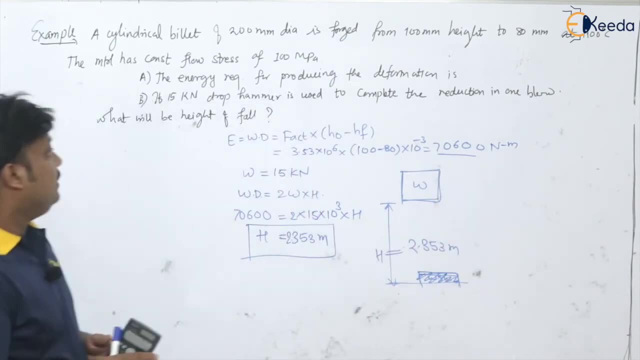 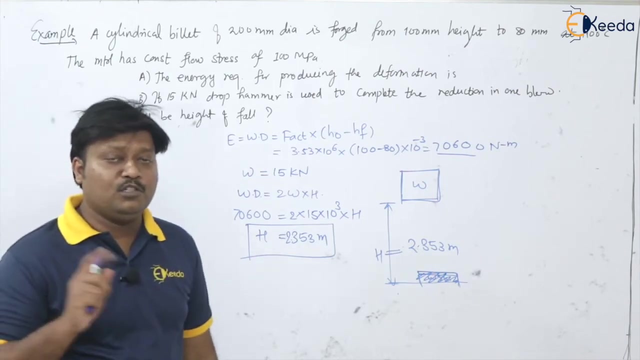 height, it will fall on to the work or billet material to get this much work to be done. okay, so this is how we can able to solve the question on the force calculation for the forging operation. now one more question I want to take here. I will not. 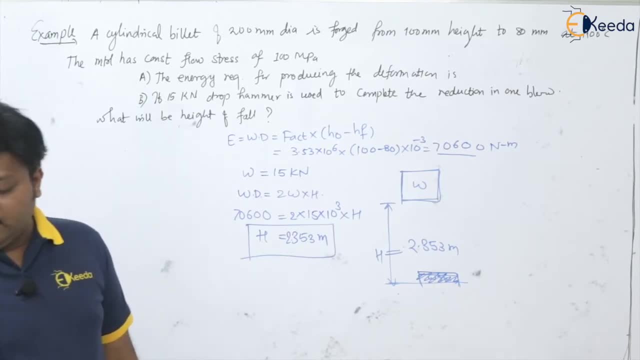 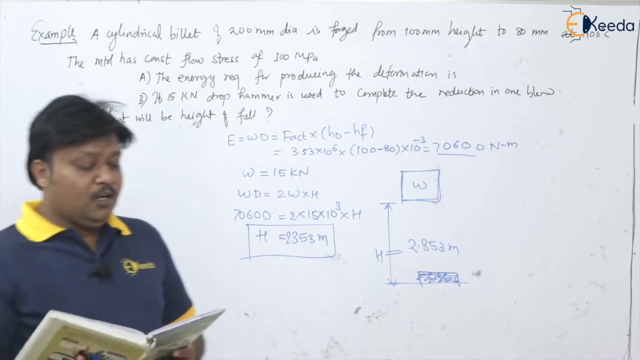 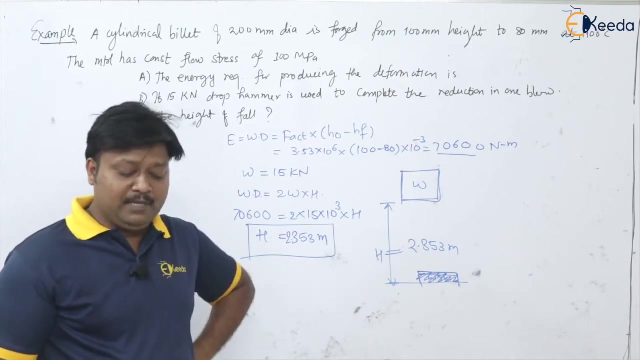 write this question. what I will do. I will read it, so listen carefully. a solid, cylindrical stainless steel work work piece of 200 mm diameter and and 150 mm height. This component is reduced by 50% in height with the flat die in open die forging, Assuming the flow stress of the material 1000 MPa and coefficient of the friction. 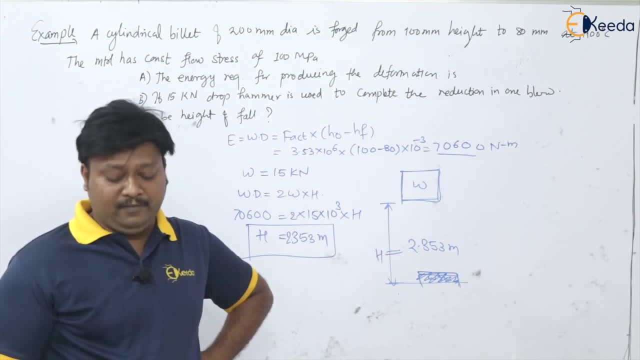 is 0.2 at the work and die interface. Estimate the forging force at the end of the stroke. Variables are 20.8 kN, 31.0 kN, 78.6 kN and 88.6 kN. 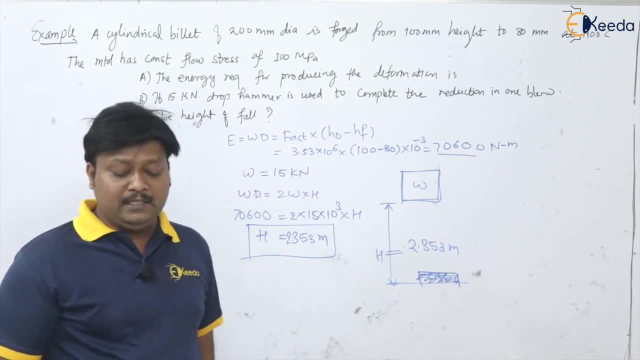 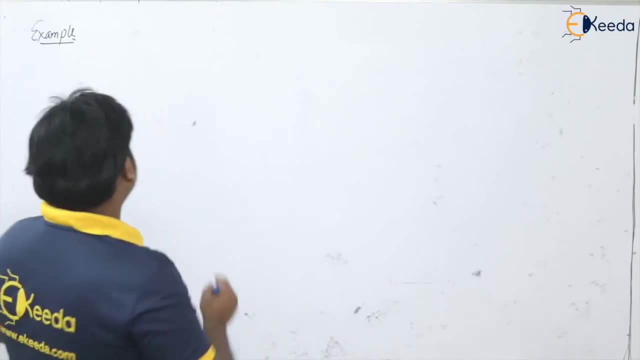 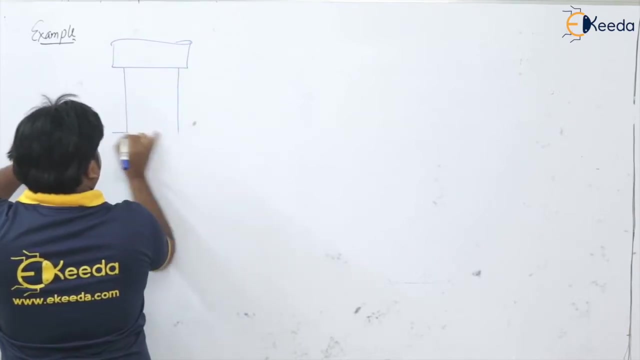 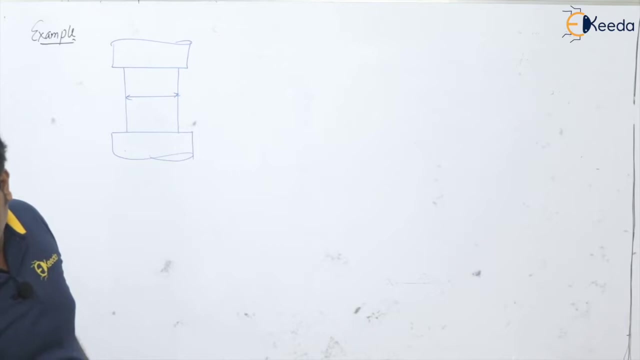 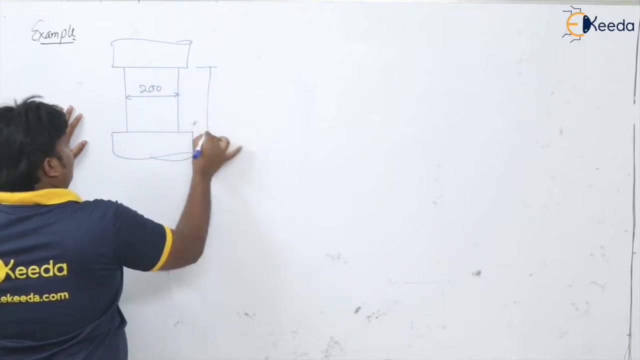 Cylindrical stainless steel workpiece of 200 mm diameter and 150 mm length. I will draw the diagram so that you can understand. I will write down the given data: Cylindrical workpiece between two flat die. Flat die is diameter is 200.. Original diameter: 200. And height is how much It is: 150 mm. 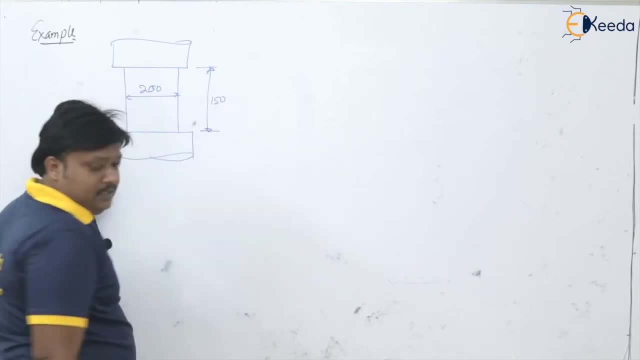 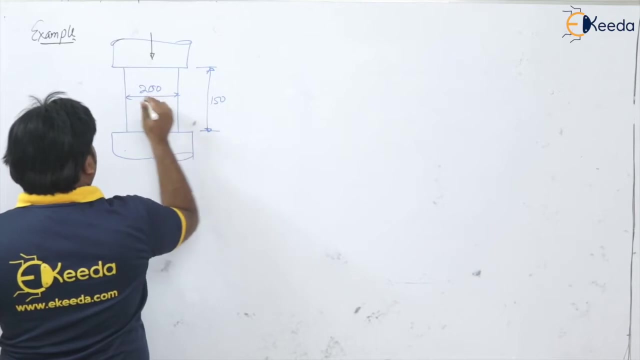 Okay, These are in millimeters. And what is they are saying? This component is reduced to the 50% height. So height is getting reduced by 50%. when this moving die will come down and apply the force, So after some time there will be the increase in diameter of. 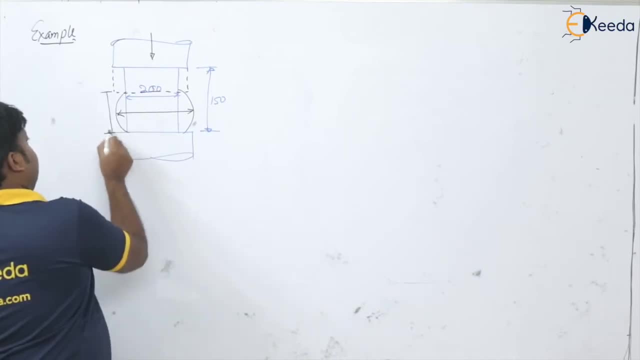 that that is not given. But height is how much now? The height now, 50% reduced, that is 75.. Okay, So this is 75 mm. This is our H final, D final. We have to calculate, Okay, And what? 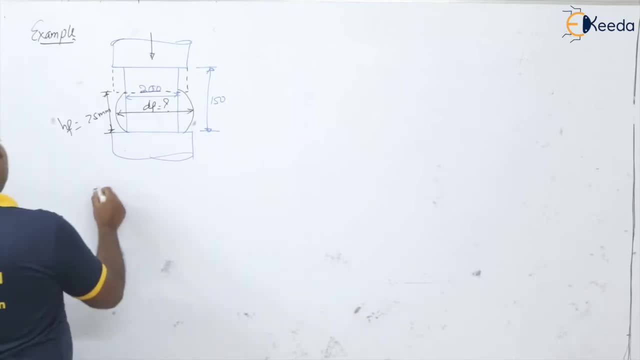 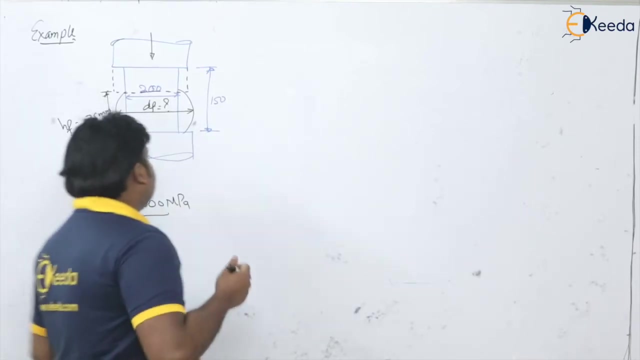 is coefficient of friction, Mu is 0.2. And the flow stresses sigma y or sigma f, it is 1000 mega Pascal. So, students, this is kind of say upsetting, isn't it? And what is given here? 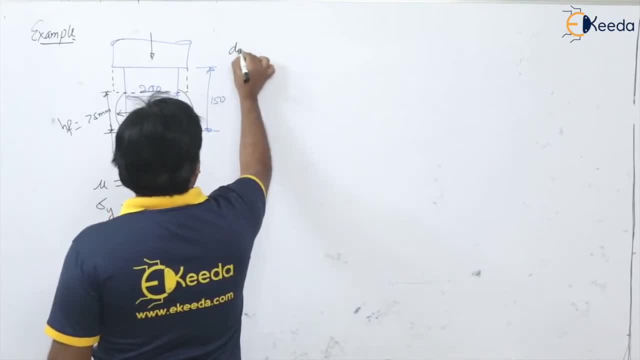 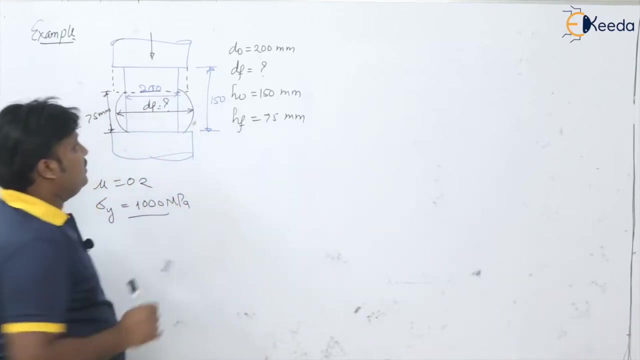 See original diameter: 200 mm. Final diameter: we have to find out Original height: 150 mm And 50% reduction mean it becomes 75 at the end of the operation. Okay, And mu is given 0.2.. Flow stress is given 1000 megapascal. So first of all let us find out the final. 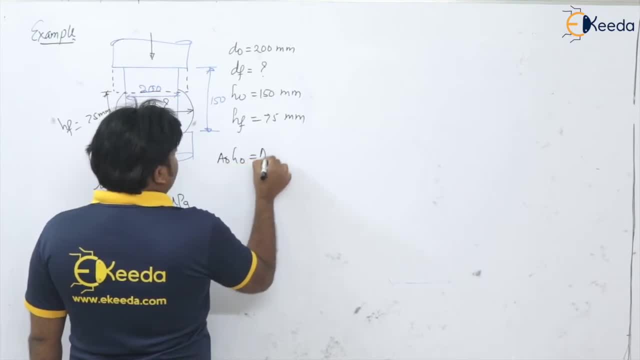 of Df. df, that is a naught, h naught is equal to a final, h final volume. constancy, that is do square. ho is equal to df, square into h final. so what is d final? that is, do under root of ho by hf. what is? 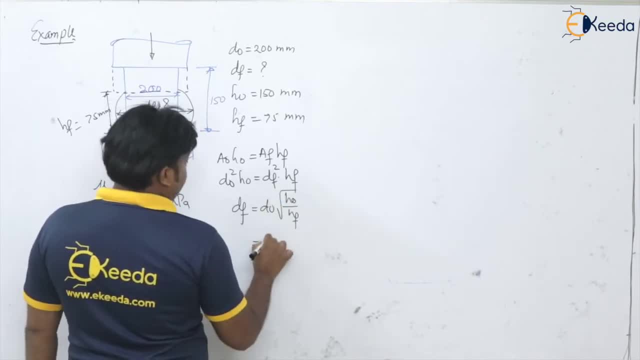 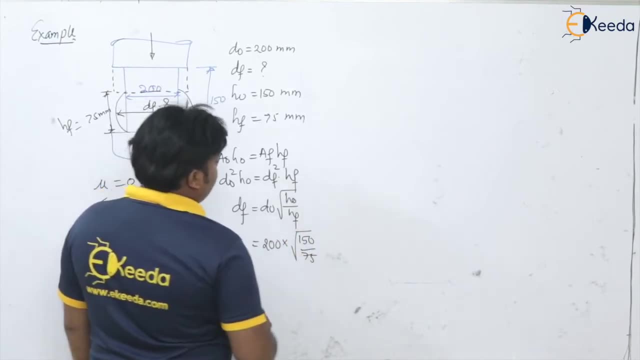 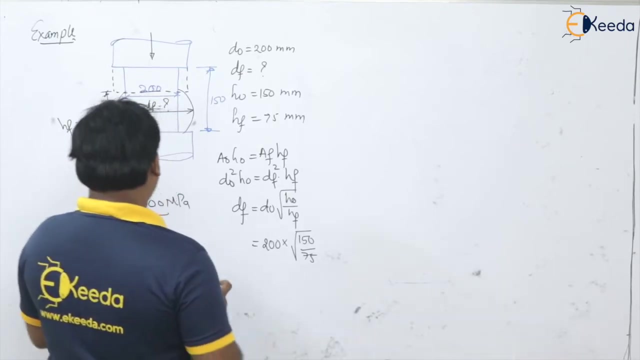 d original. d original is 200 into root of h, original, 150 divided by 75, so 200 into root 2, 200 into root 2, it is 282.84, 282.84 millimeter. this is the final diameter, isn't it? 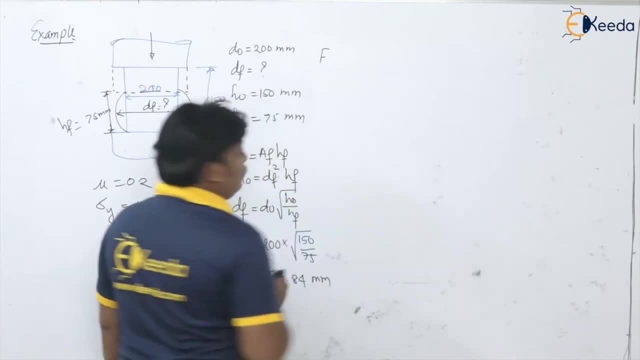 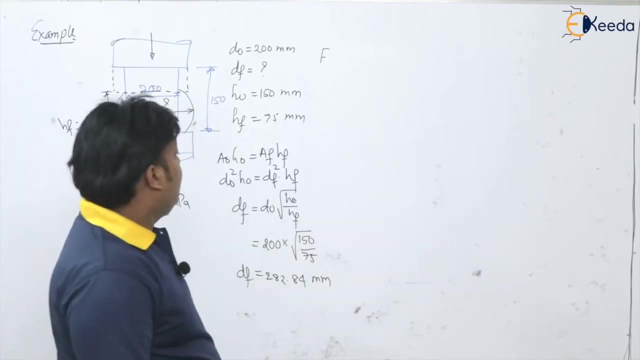 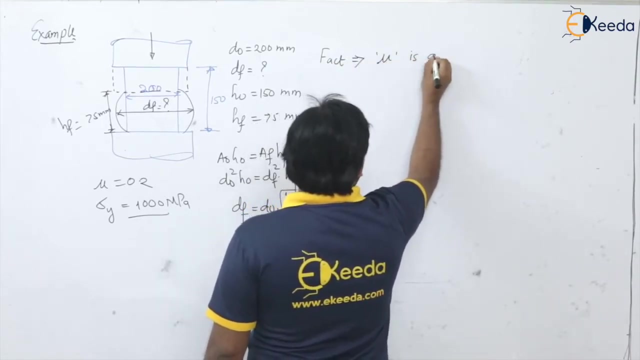 so what is the fourth force at the end of the stroke? always, see, this is the assumption. we already learned that the maximum force is at the end of the operation in the forging process. so f actual. we know that whenever the mu value is given, mu coefficient of friction is given, what is this f actual? 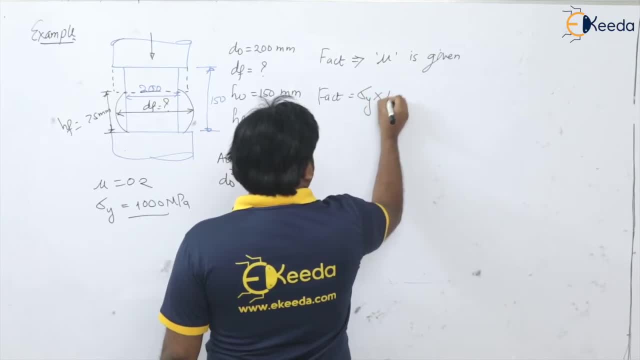 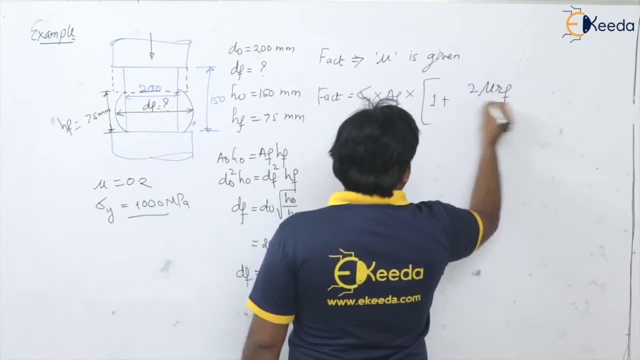 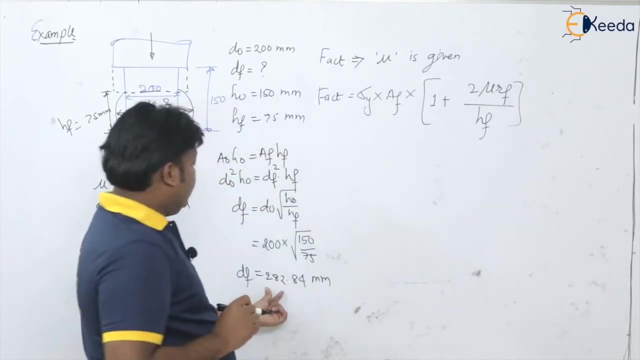 this is nothing but this sigma y into final cross sectional area, into bracket one, plus 2 mu r final, divided by 0. h final. we know this now r final. how much this 282.8 word divided by 2, you will get the r final. 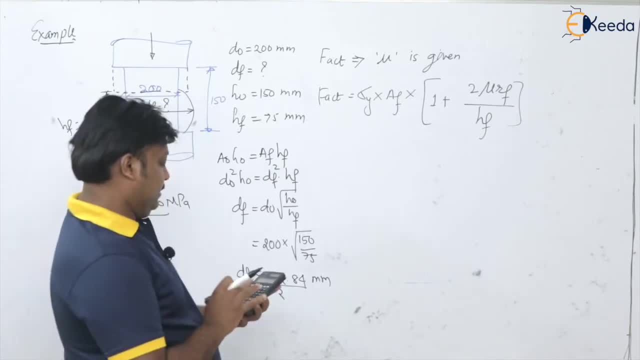 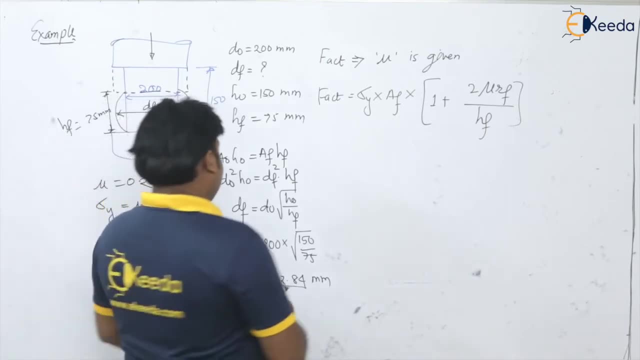 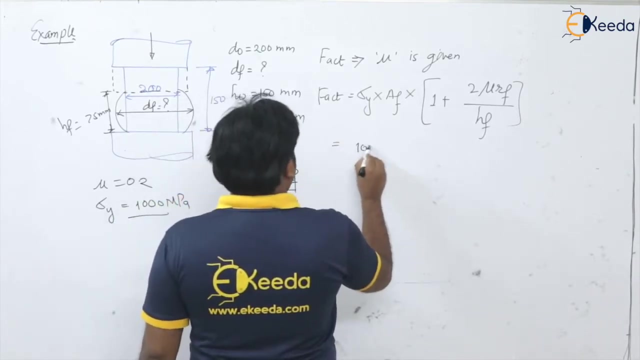 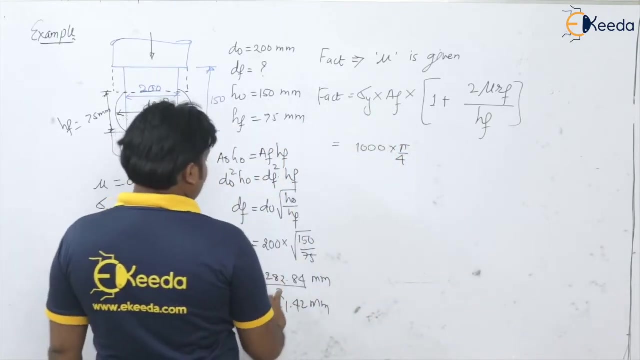 how much 282.84 divided by 2, it is 141.42, it is 141.42 millimeter. okay, so sigma y is 1000 into pi by 4, the original or the final diameter, that is 282 282.84. 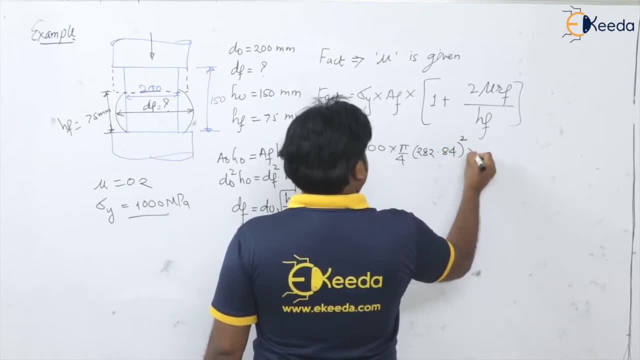 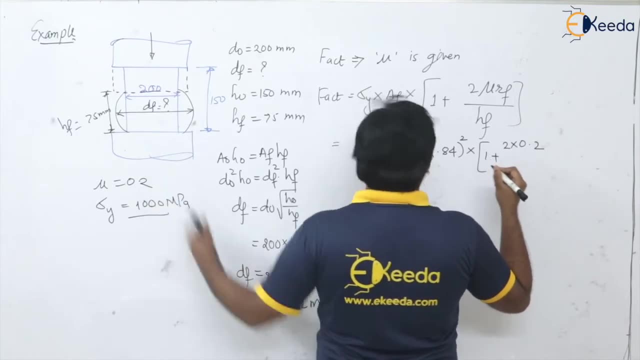 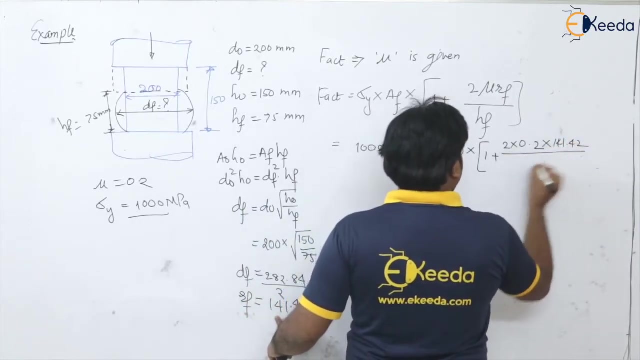 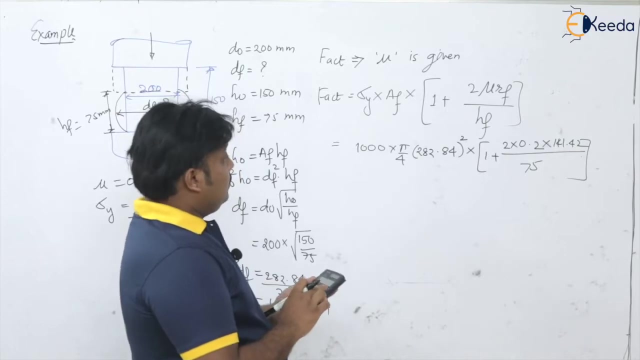 square into bracket 1 plus 2 into mu. is how much? 0.2? okay, and two RF 141 for to .42 divided by final height, 75 to calculate this, and we'll get the answer, sorry, in total into 0.2 divided by 751, plus answer into: 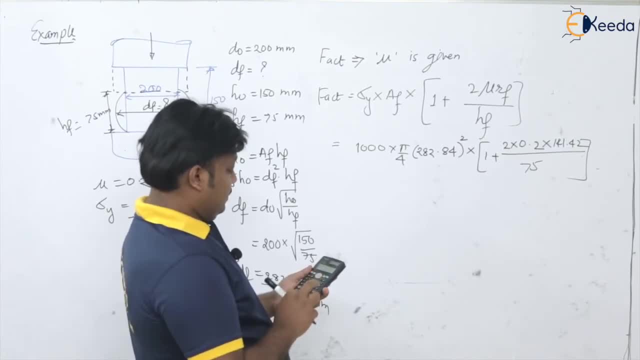 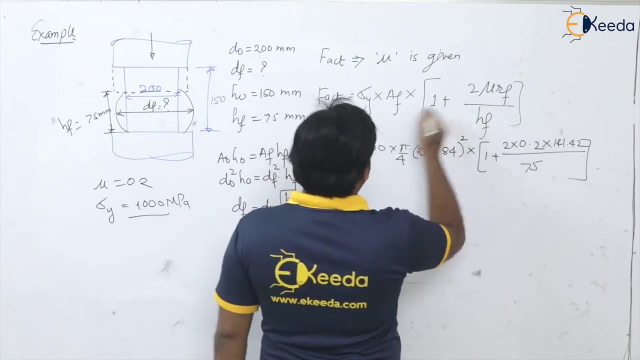 282.4 squared into 250 times pi. so it is how much 141.42 to 0.2 into 2, divided by 75 plus 1 into ok. so the formula is: 1 sigma y into a final, into 1 plus 2 mu rf divided by 3 hf, this is: 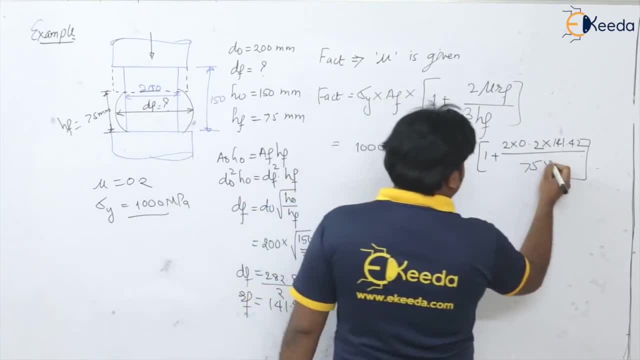 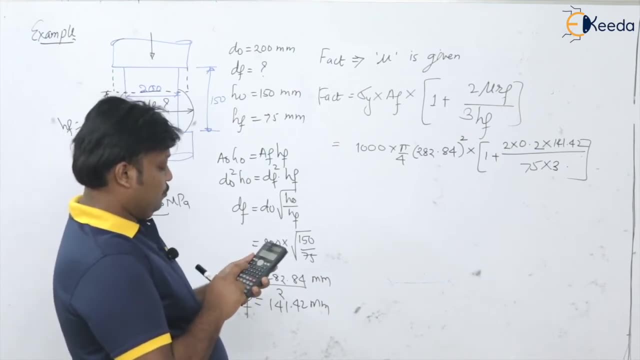 a formula, have you know? so it is here, multiplied by 3, so you will get 141.42 to 0.2 into 2, divided by pi, divided by 3 plus 1 into 2, at 2 point, at 4 square into 250. but it is equal to. you are. 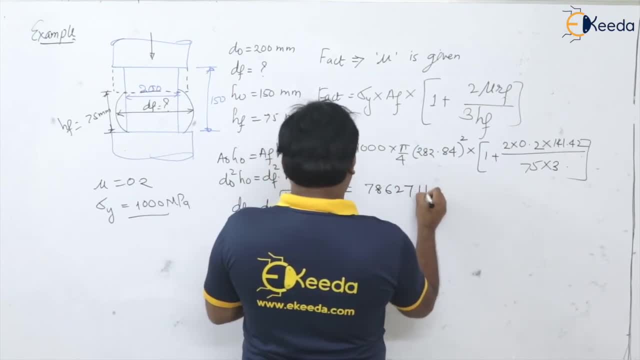 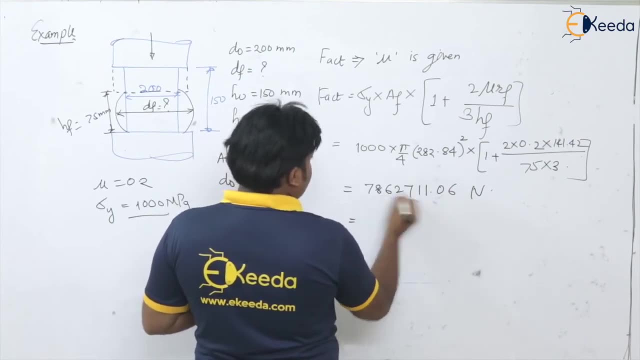 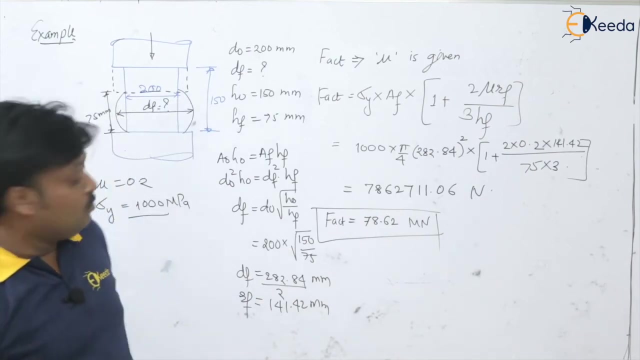 getting 7, 8, 6, 2, 7, 1, 1, 0, 6 Newton, so it will be 1, 2, 3, 4, 5, 6, 78 point 6, 2 mega Newton. it will be mega Newton. ok, so the option should be in mega Newton. see, yes, the option should be in. 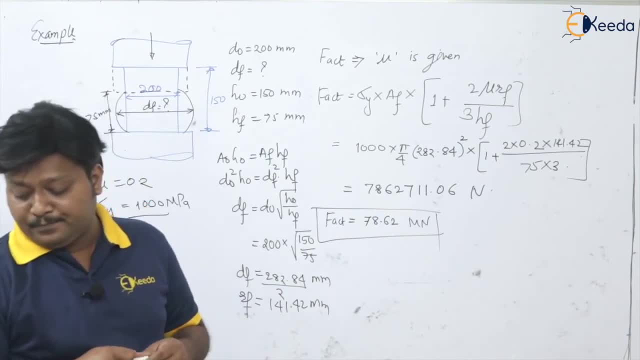 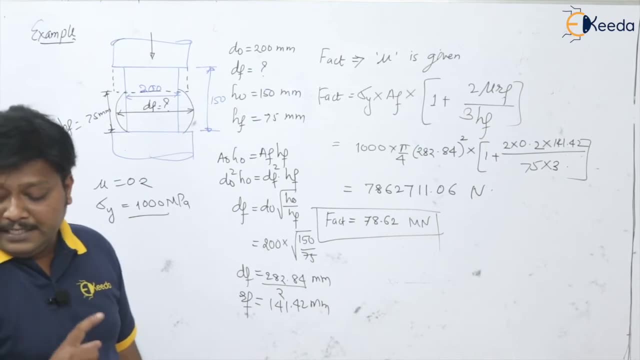 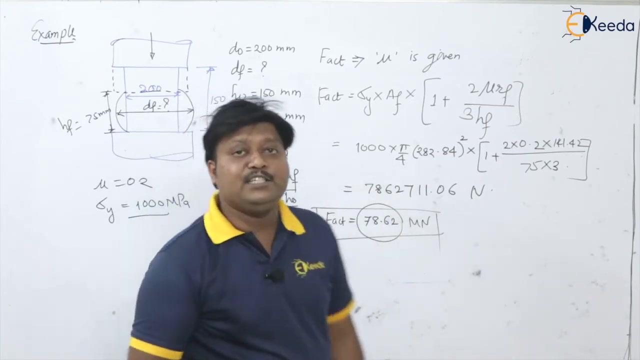 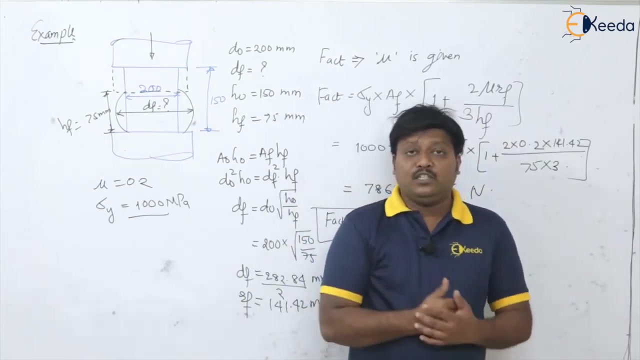 mega Newton's options are 28 point, 20.8 mega Newton, 31 mega Newton, 78.6 yes and 88.6 mega Newton. so yes answer will be what this? 78.62 mega Newton. so yeah, these studies are the kinds of four Times 5000. the questions on the force calculation. 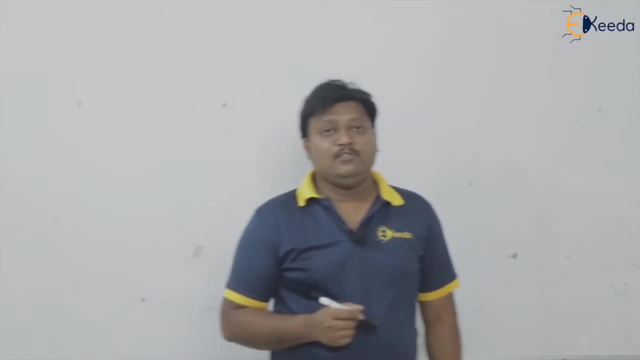 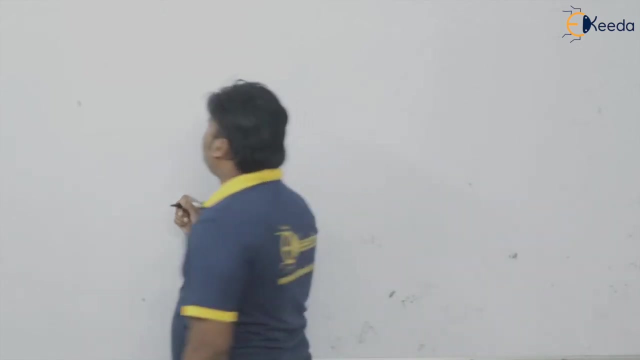 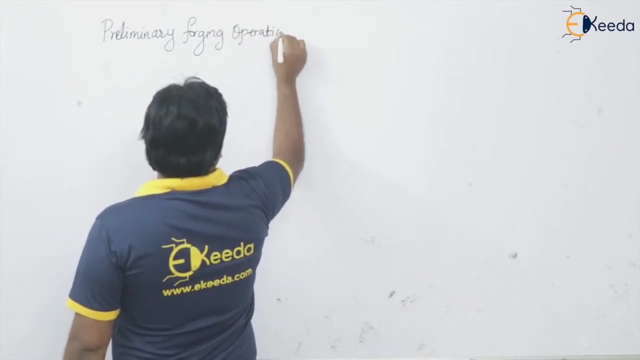 in the forcing operation. go treat it in times 5000.3 mega Newton, 4lean time in real-time- Impossible. I MS VED 13 würstel very fast. so we really want Jang operations. so even see it one by one. number one is the fuller. 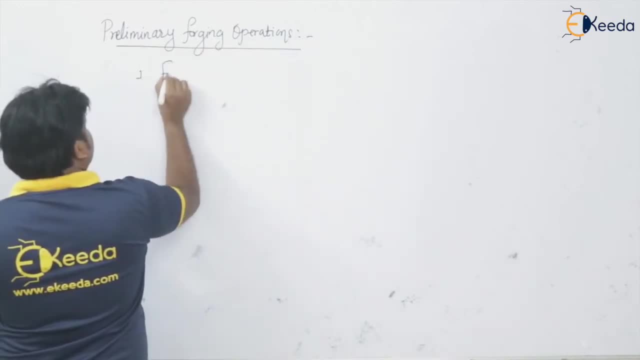 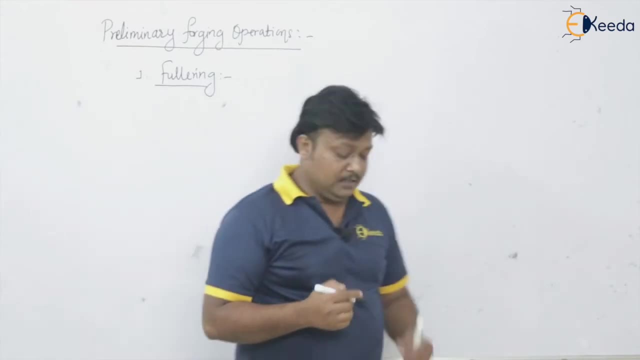 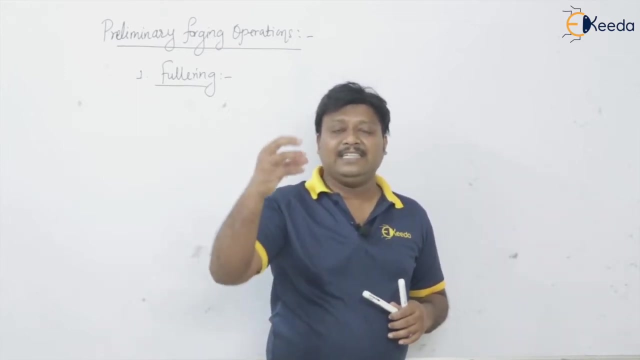 starts by과ît 00URH, 00URH, 00URH, Fao, 00URH operation. so the fully in the full ring operation. what we are doing, we are relocating the material along the lengthwise direction, so definitely increasing the cross-section area, increasing the length, but it is. 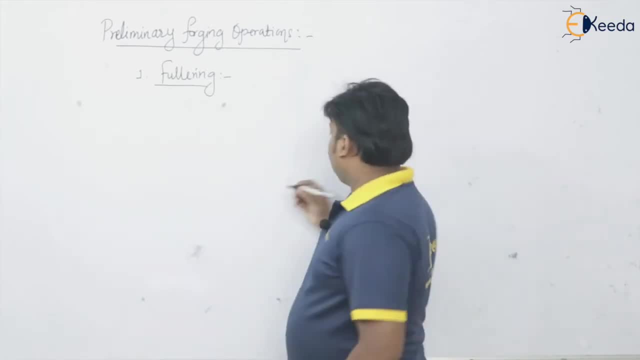 uniformly. if you see the full ring, so suppose on the anvil, so this is the, and we will. so here is say the lower fuller is there, or bottom fuller is there, and here is we are having the top fuller, okay. so here we are going to get the. 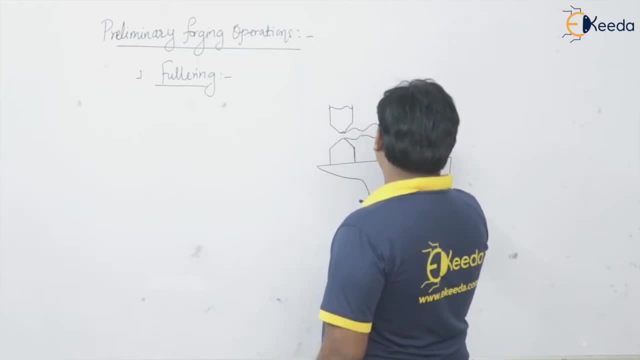 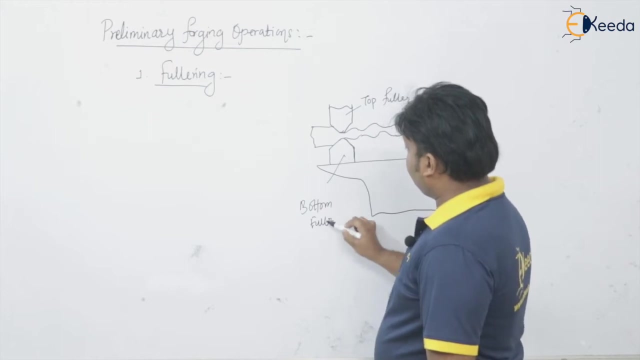 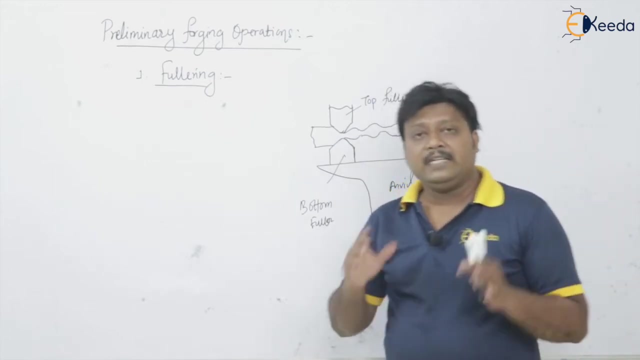 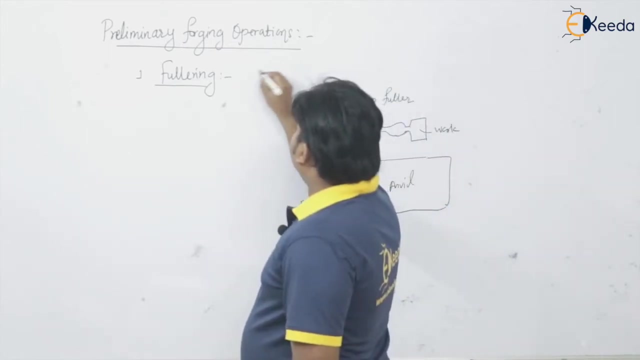 marks of this fuller on to this work surface. okay, are getting some marks here say this is the work, this is the top fuller, this is the bottom fuller and this is the anvil. so in this fullering operation, we are distributing the material from center to the outward, but non-uniformly, isn't it? 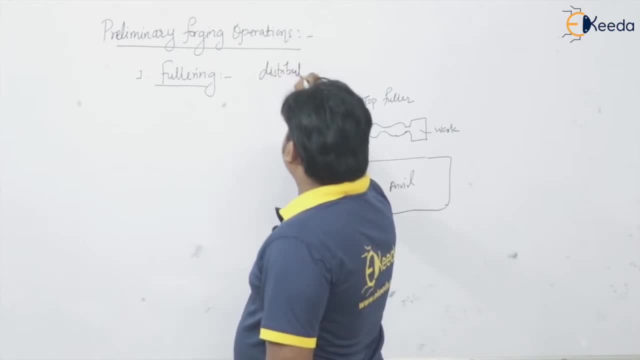 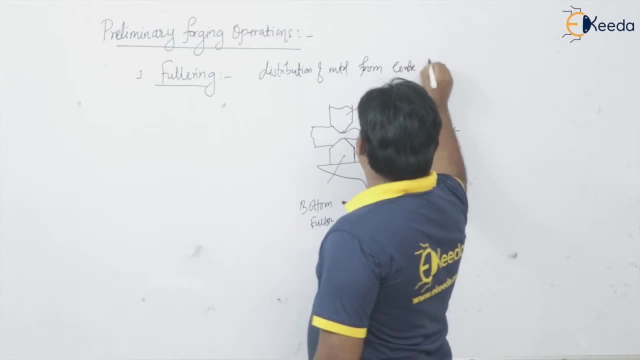 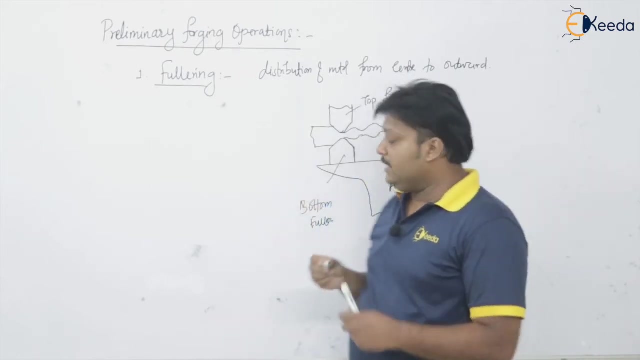 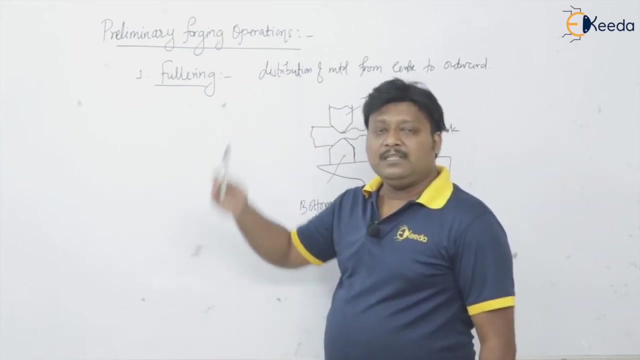 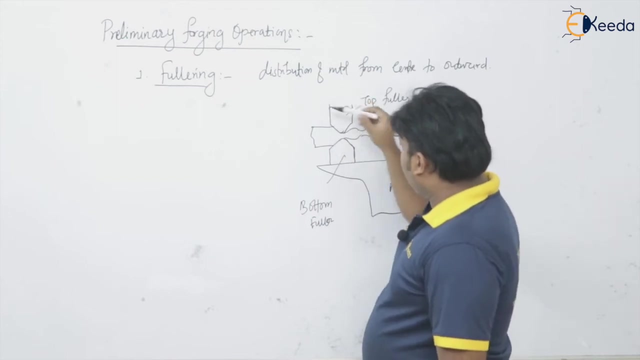 distribution of of material from center to outward. so because of that, what is going to happen? the see, the length of this work piece is going to increase, but the section, for example the diameter, is going to reduce. so here the force is applied, see, perpendicular to the axis of the work piece, isn't it? the force is 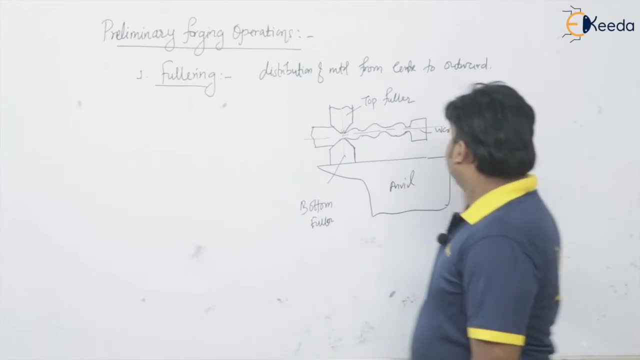 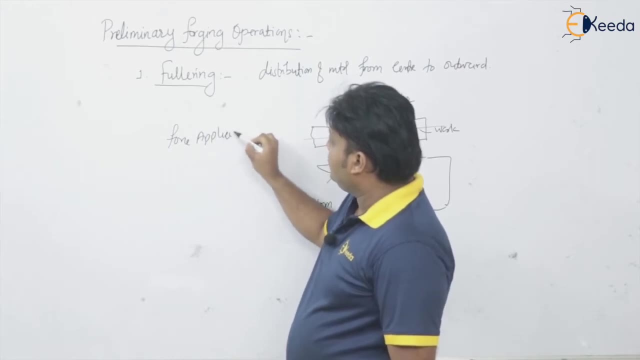 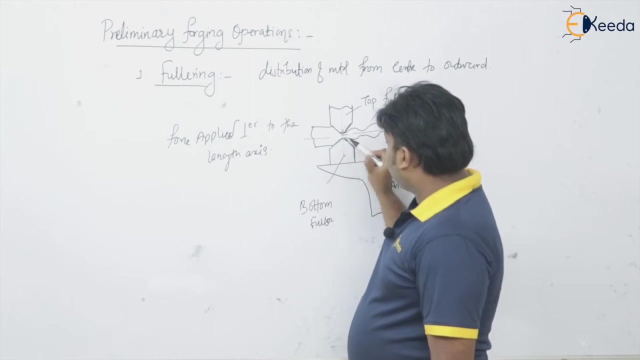 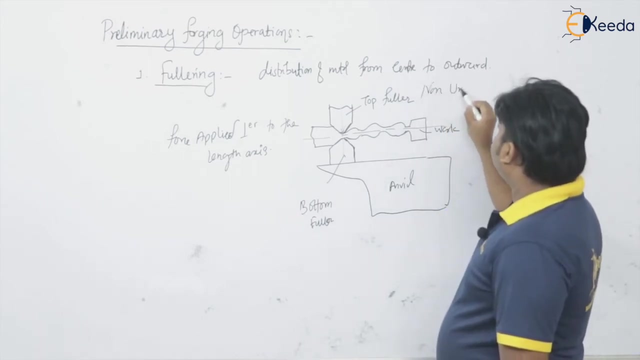 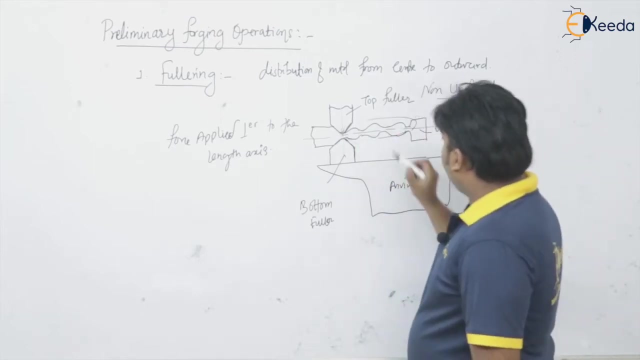 applied in the direction perpendicular to the length axis, force applied perpendicular to the length axis, length axis and, of course, because of this marks of the fuller- see the marks of the fuller- we can have this non uniform. the process is non uniformly to remove these marks of this fullers. what we have to do, we have to use the. 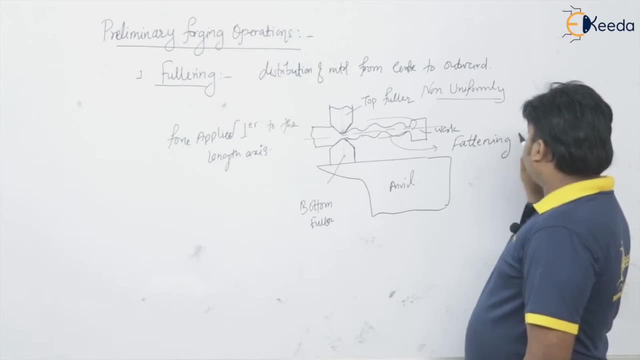 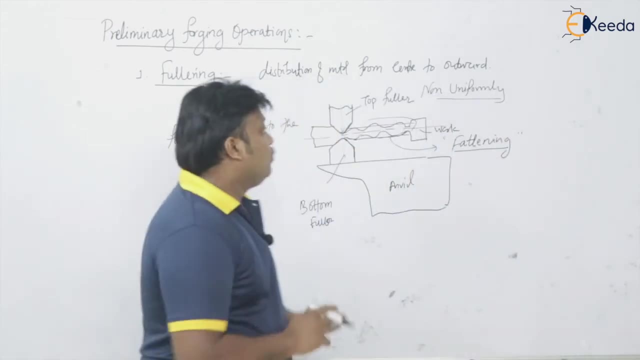 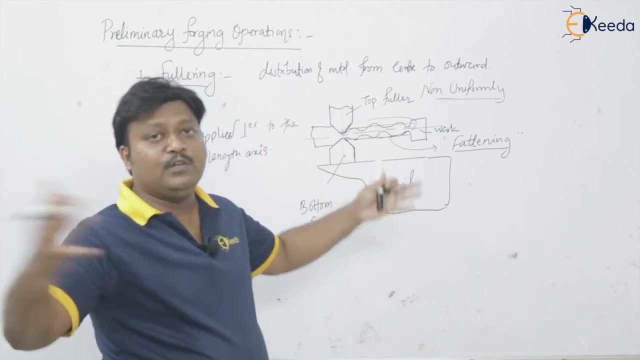 flattening. the flattening process is done so that we can remove the mark and we can make the part more uniform. so basically, basically, the idea is this: in the full ring operation, the material is distributed from the center to the outward direction. length is going to increase cross-sectionally, going to 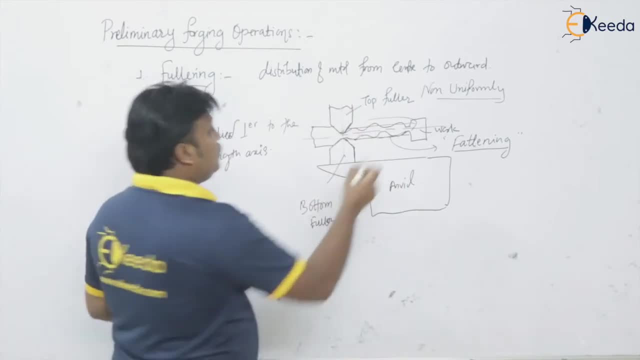 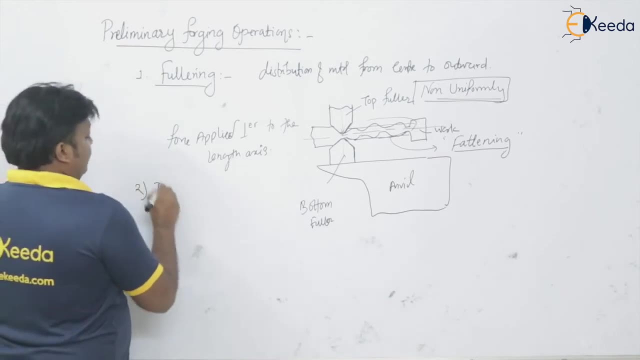 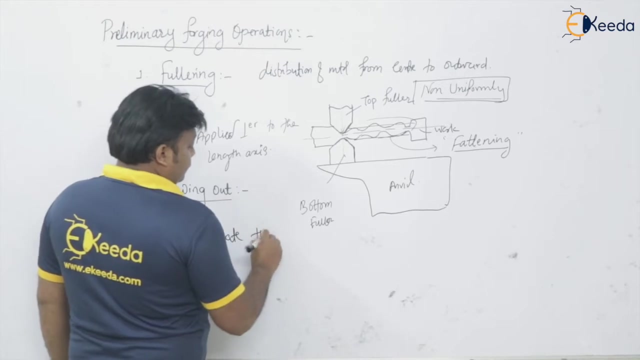 decrease non uniformly. so this word is important here. okay, now the next operation. we are having the drawing out operation, the drawing out operation. so in the drawing drawing out, the same thing we are going to do: we are going to elongate the material in the lengthwise direction and we are decreasing the 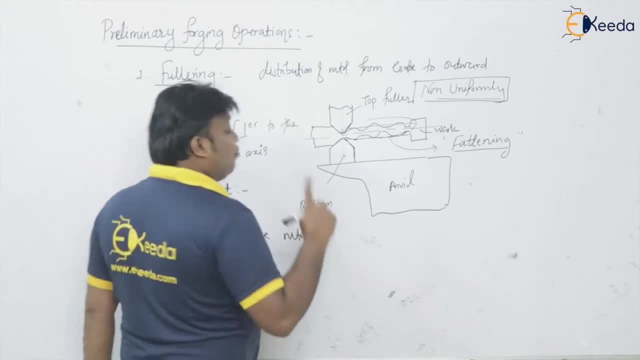 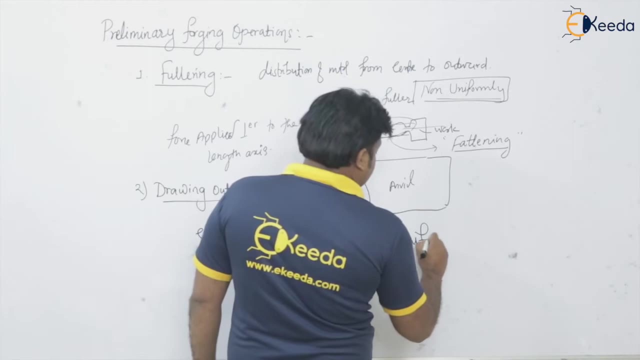 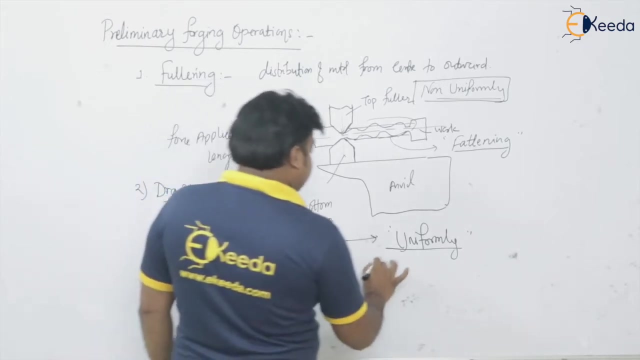 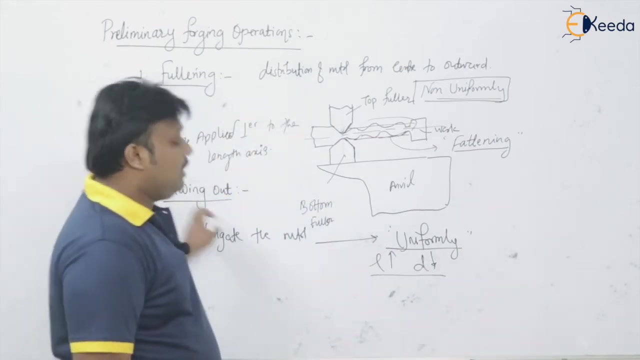 cross-section of the component, but more uniformly, please remember so. same process as like this, but it is uniformly. it is uniform, please remember so, the distribution of the material from center to outward, increasing the length and decreasing the cross-section, that is, diameter, of the component or workpiece. this is known as the drawing of or. 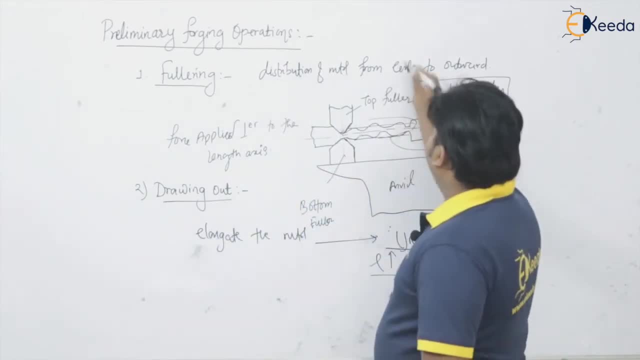 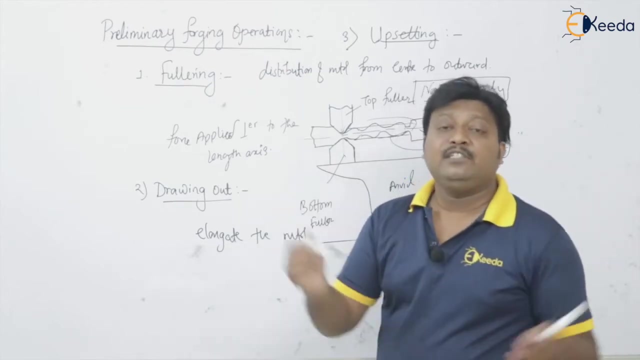 drawing out operation, then the next operation we are having the third operation I will take. that is upsetting. this is simply we have seen in the open die forging operation. so here the material is going to compress between the two flat dies. we have seen this operation. see, this is top die, this is the workpiece material, or 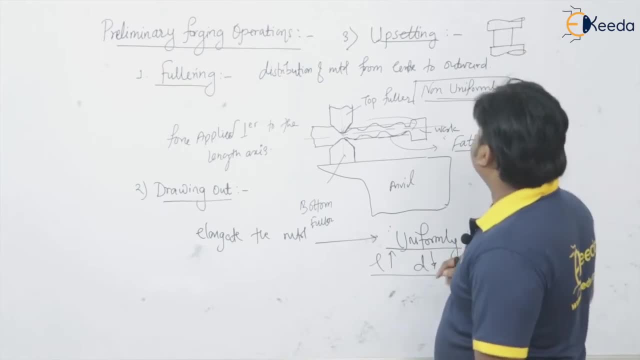 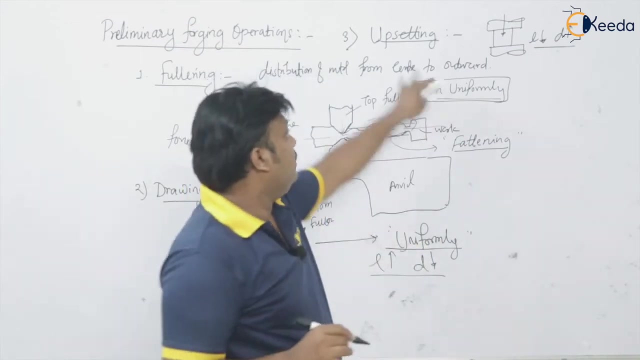 billet material. this is the stationary die, this is moving die, and we are applying the force, compressive force, isn't it so that what is going to happen? the length is going to decrease, but cross-section is going to increase, isn't it so? this is the upsetting. the third preliminary forging operation. 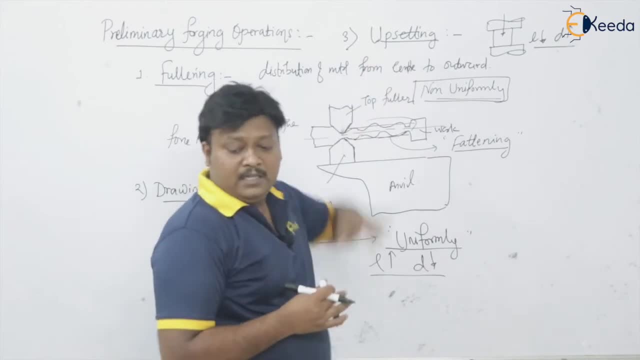 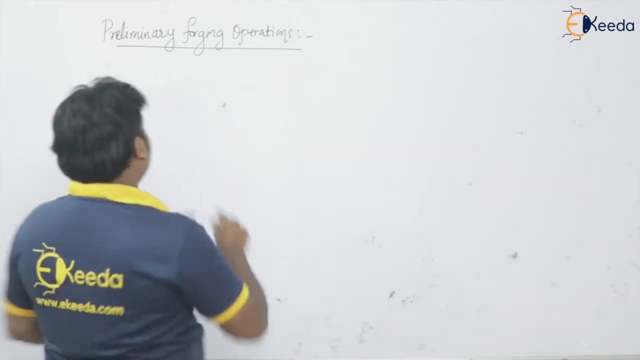 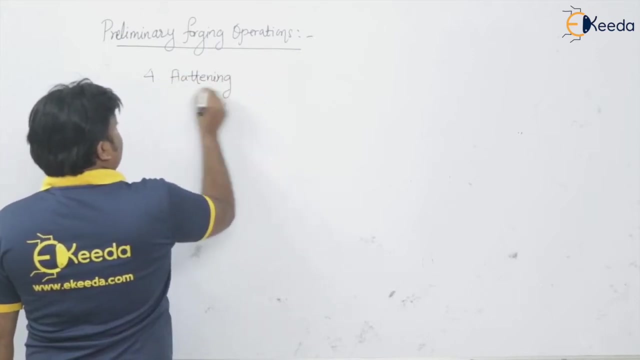 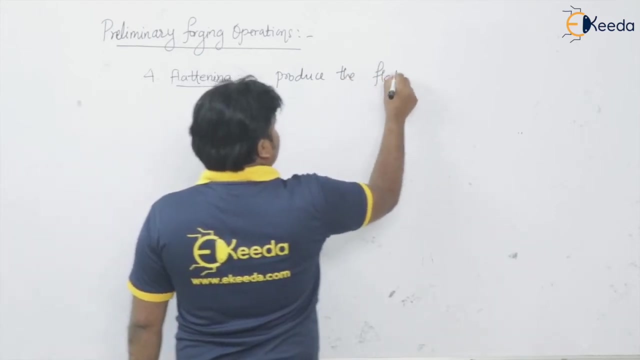 is the upsetting, then we are having flattening, the fourth process that we have, that is the flattening. so flattening is what produce? the flat surface. produce the flat surface or to put more uniformity in the workpiece, or to put more uniformity in the workpiece or knitting. 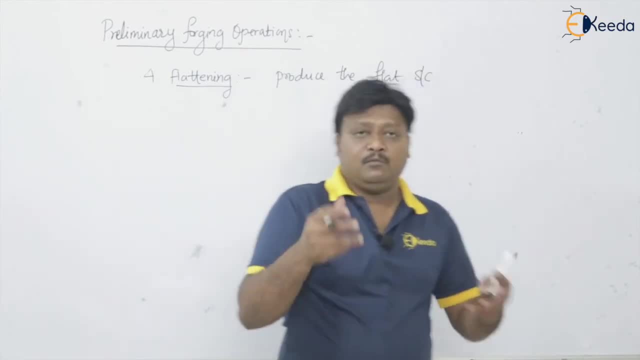 or ordered production in wouldn't be a good shape. shape, shape. through the modelト pour the flat surfaceид І لفب, worlds are coming up, if you want. this was never country. this is right, not easy Workpiece. as we seen in the fullering, the part is no more uniform. 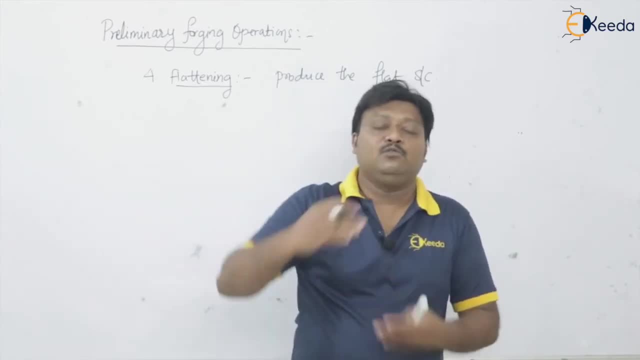 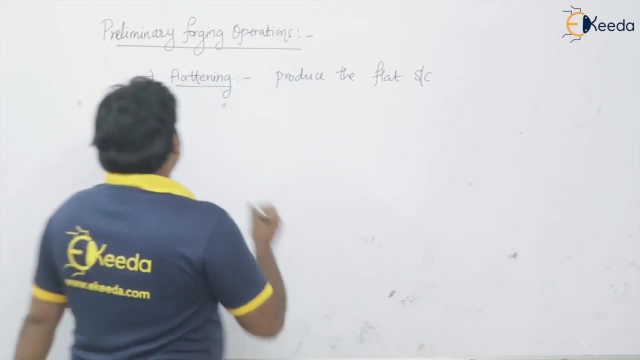 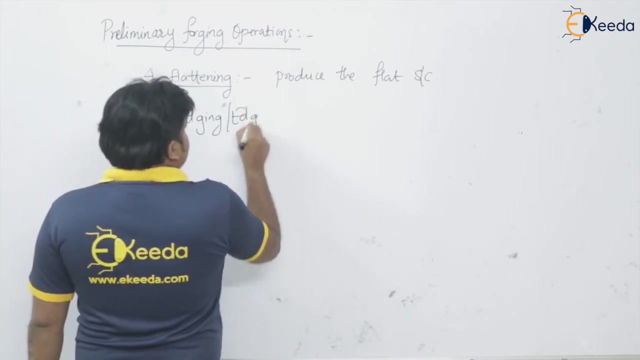 So, to remove that non uniformity, we used to have flattening after the fullering operation, isn't it So that is producing the flat surface. That is a flattening. then, fifth, We are having Edging, or edging, edging, or this is also known as edging. So what is mean by this? 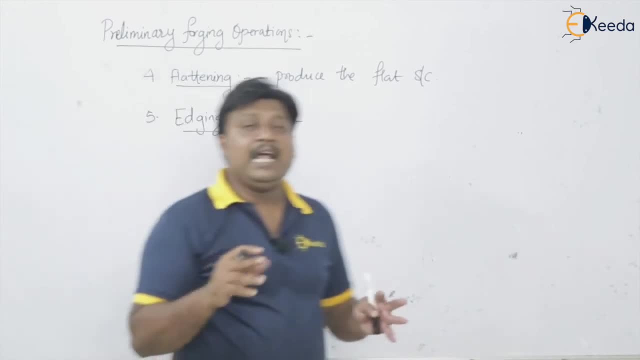 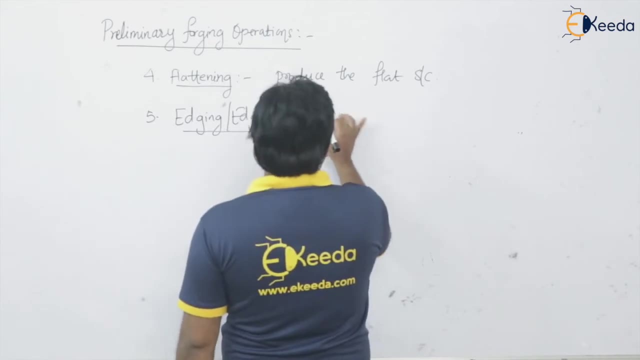 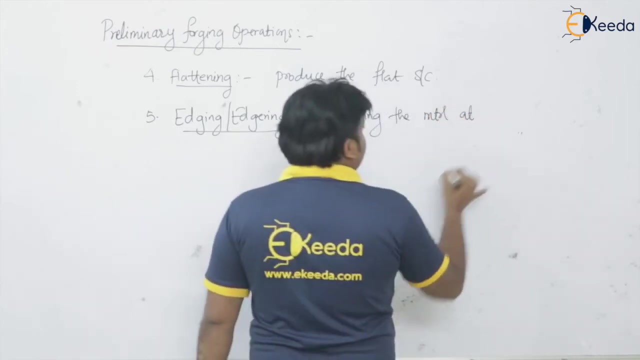 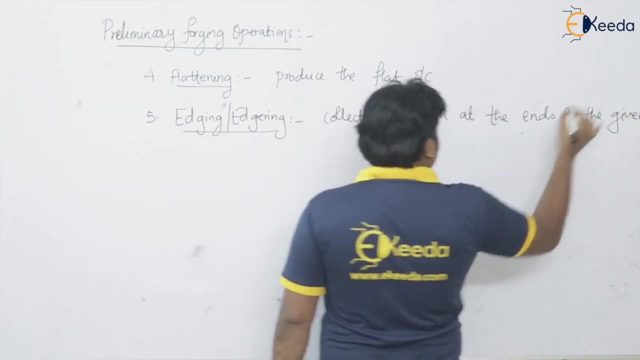 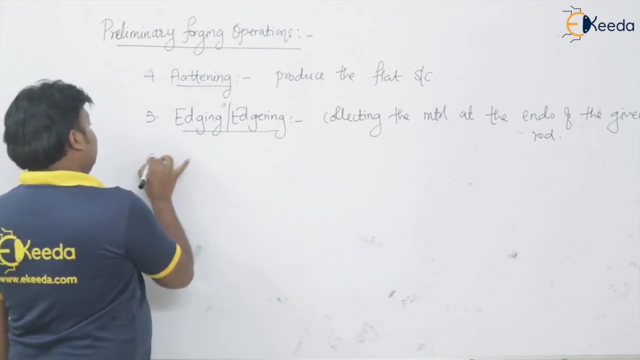 so this is nothing but collecting the material at the ends of the Given workpiece or given bar. So distribution are the collecting the material, collecting the material at the end, at the ends of the given bar or whatever For the operation, isn't it? So this is the edging, or edging operation. sixth one We are having that is chamfering. 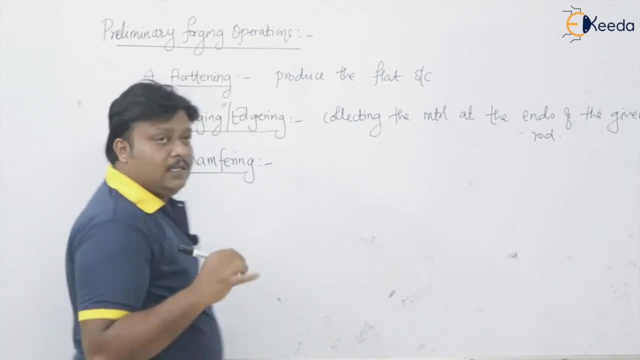 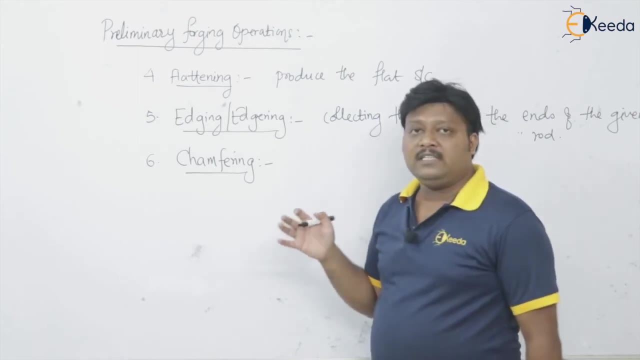 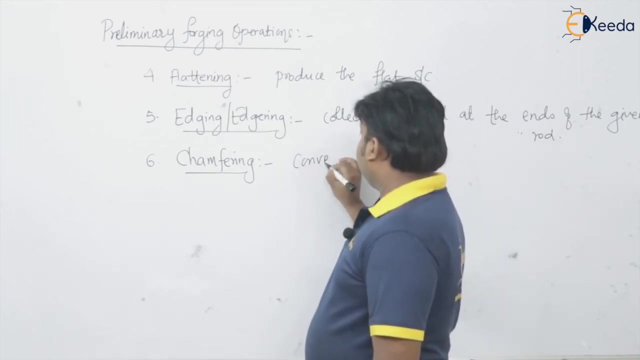 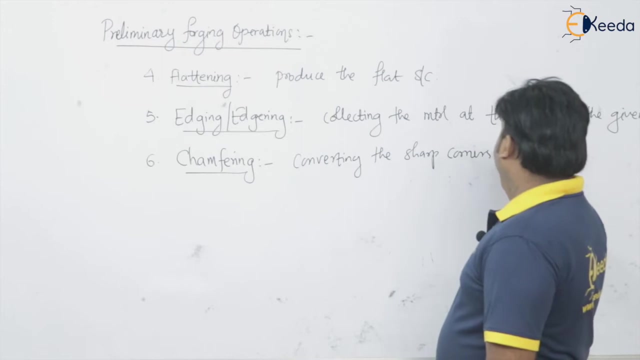 Chamfering. chamfering is what? Making the sharp corner into the some Soft corners that it with some radius, that is nothing but the chamfering that is. chamfering is nothing but converting The sharp corners into Smooth corners by giving the corner radius. Yes or no? 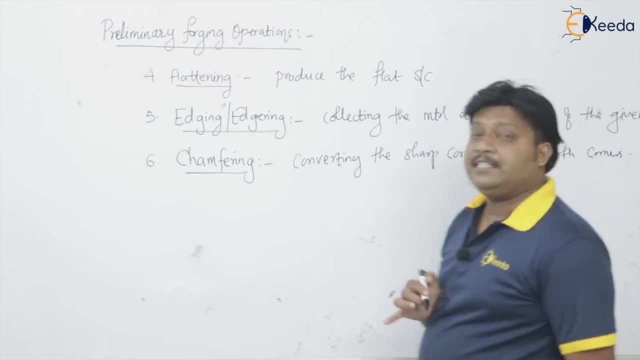 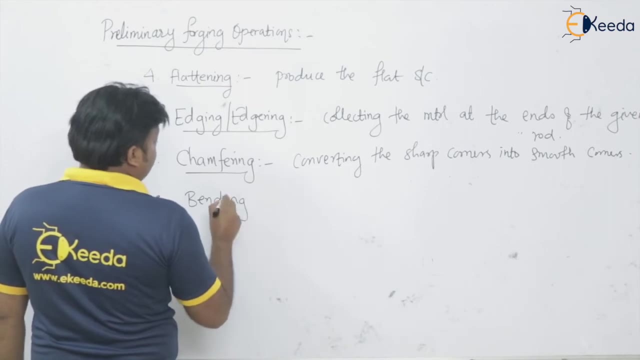 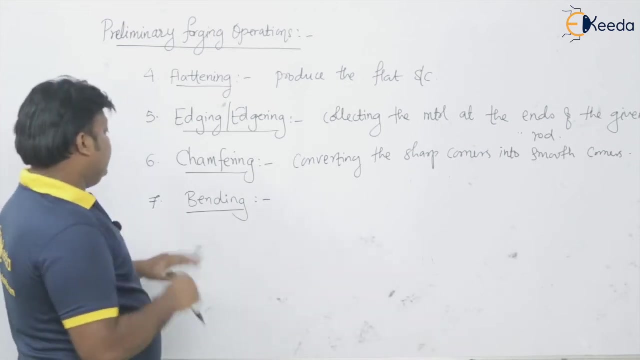 Smooth corners. so this is the Chamfering seventh one. we are having the bending, We have learned this operation, bending, Or we are going to learn this operation in the sheet metal operations. so bending is the operation, is what? where the material is deformed along the straight axis, which is lies in the 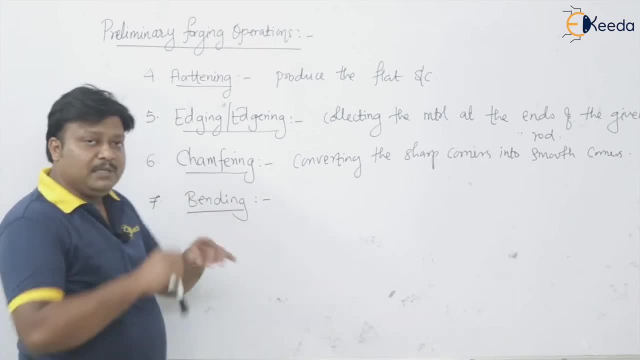 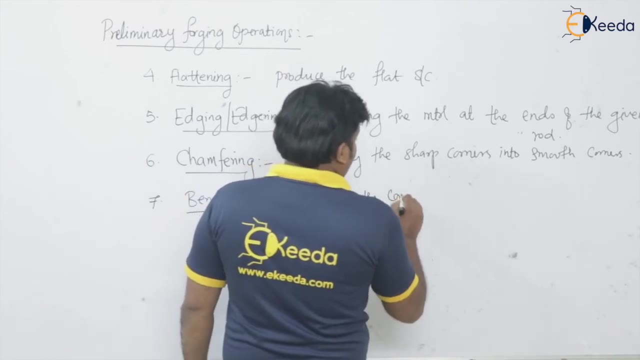 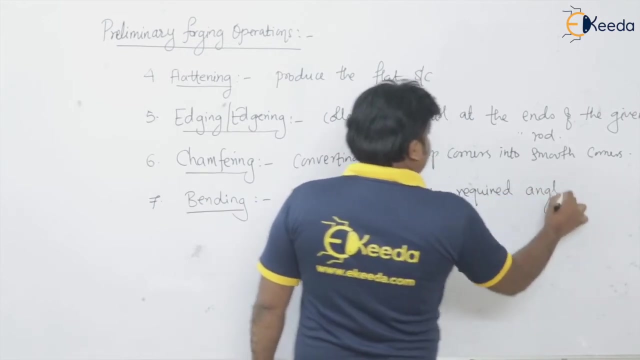 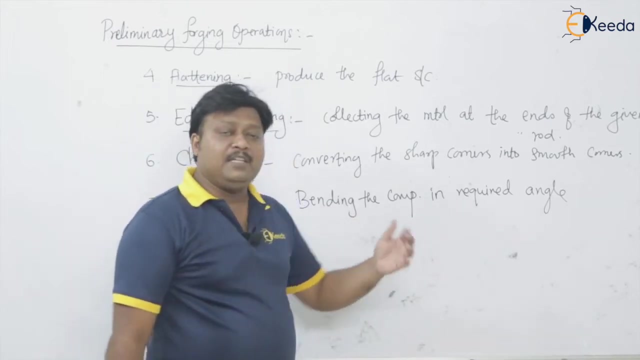 neutral plane. okay, so bending is nothing but simply bending the component, bending the component or workpiece in a required angle, in a required angle. for that we are having the various dies. we are having wiping die. single edge die are same, only wiping die and single edge die are same. then we are having v bending, die u bending. 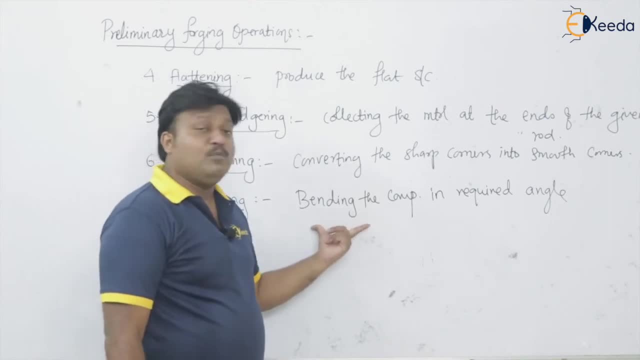 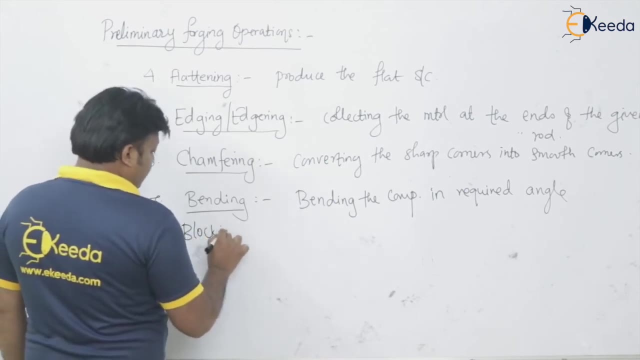 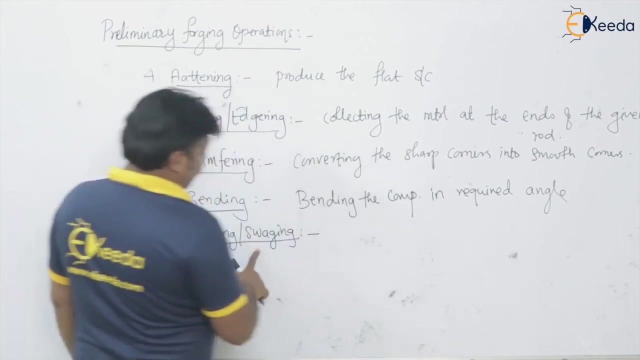 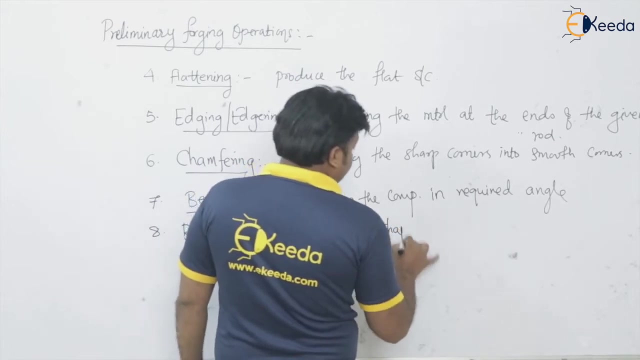 die like. these are the various kinds of bending operation we are having. okay, eighth, we are having the blocking or swagging operation. blocking or swagging, so what is this operation actually? in this operation, generally, the rough shape of the component is produced, the rough shape of the part. 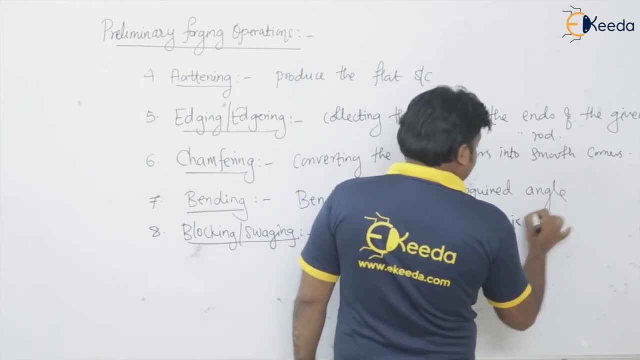 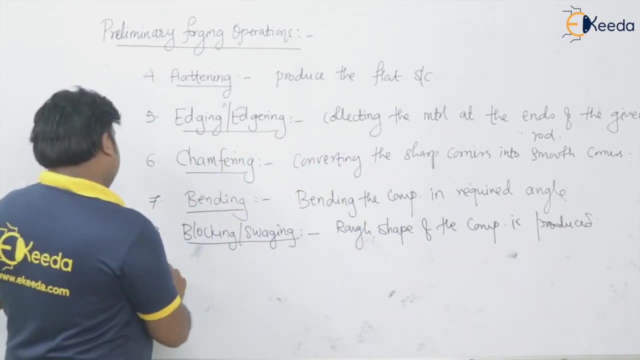 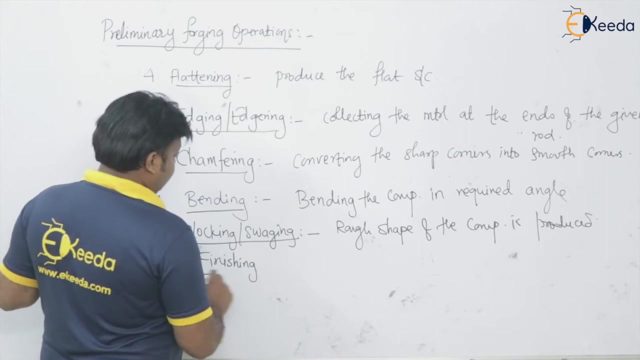 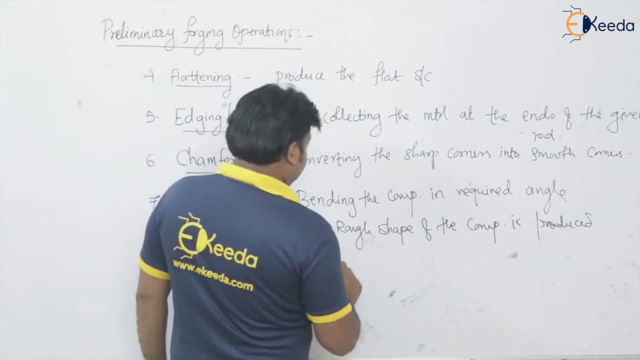 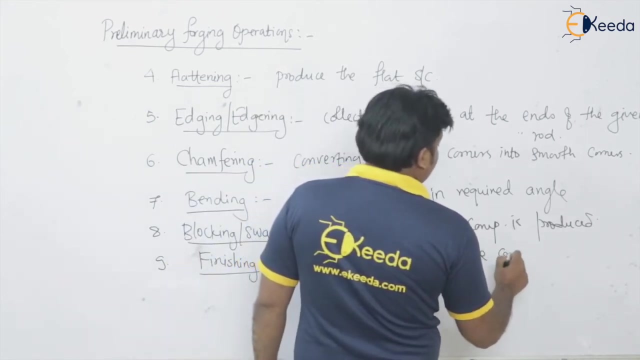 or component is produced. this is the blocking or swagging operation. ninth operation is our finishing operation. it is the finishing operation that is. finishing means what? so? exact size and shape of the component is obtained, exact shape and size of the component is going to obtain, and. 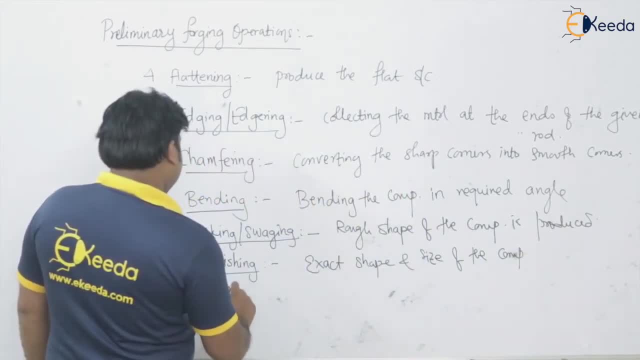 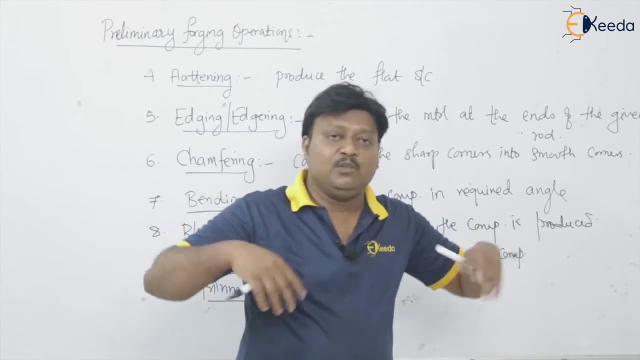 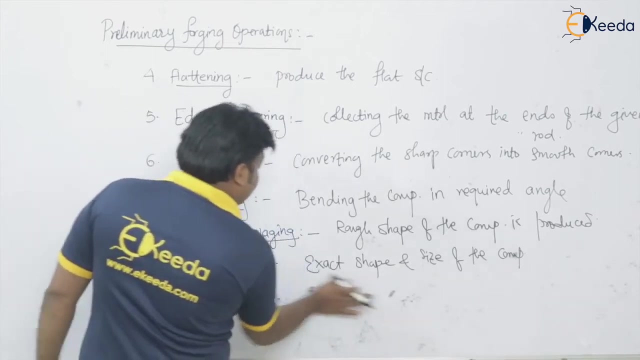 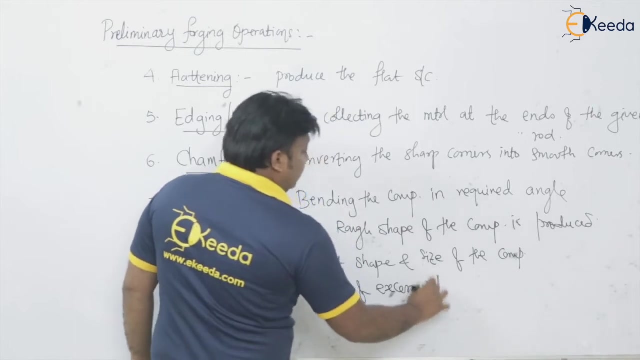 the last one I will write here: the trimming operation. so, whatever the excessive material which have shown the circumferentially, in case of the closed eyes, as a flash, that can be removed by their trimming operation, that is, removal of excess material, removal of excess material from the components for the 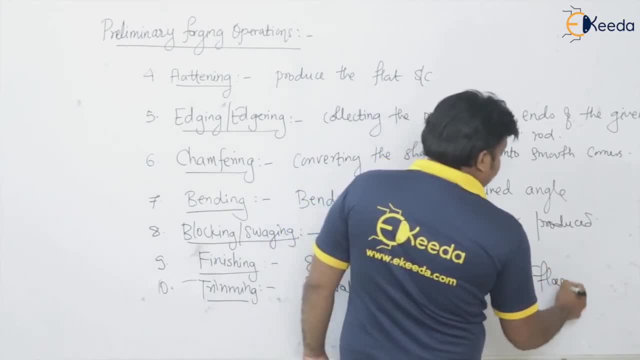 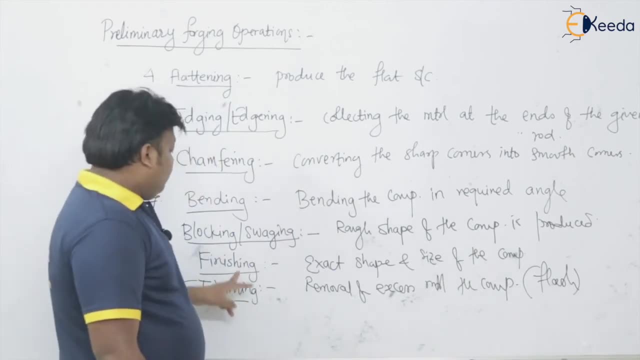 components for an inch. in bracket I will write: flash is going to remove by the trimming operation and please remember that trimming is always done after the finishing, or I can say the finishing is always followed by trimming and this blocking is always followed by finishing. now see, this is four, five, six, seven, eight. 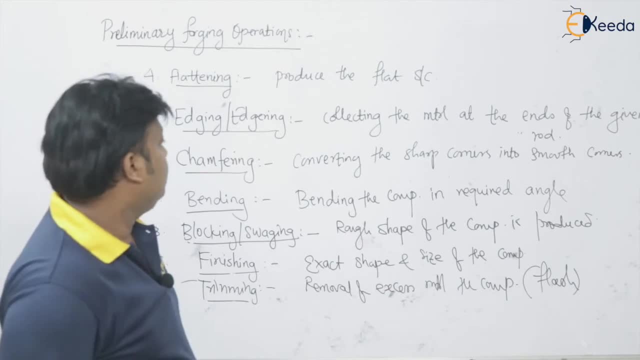 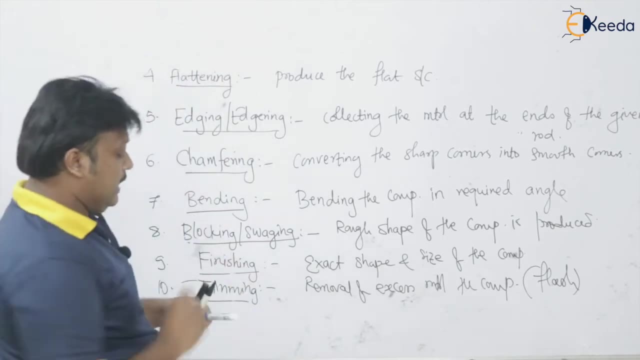 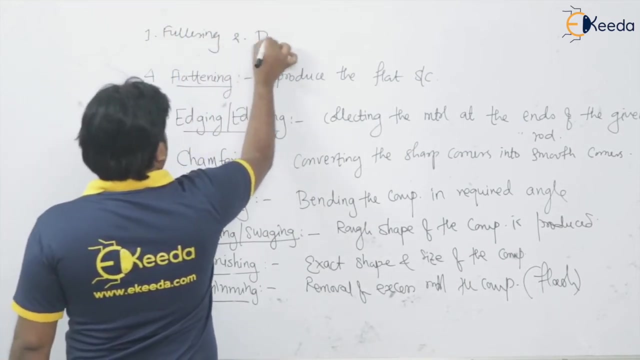 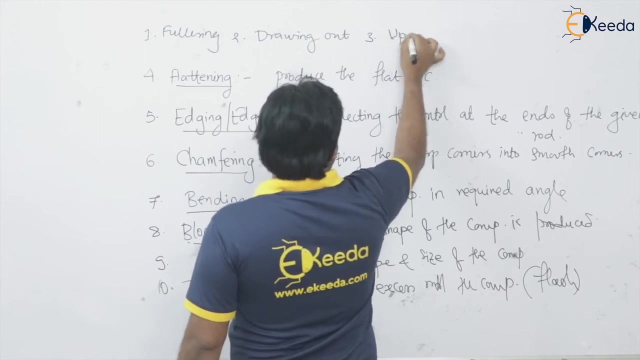 nine ten. so I will write once again, whatever the processes we or operations are used for the trimming operation. so I will write once again, whatever the processes, we or operation, preliminary operations which have we discussed. so number one, catheter. number one, fuller ring. then second was drawing out, third was upsetting, isn't it? so one 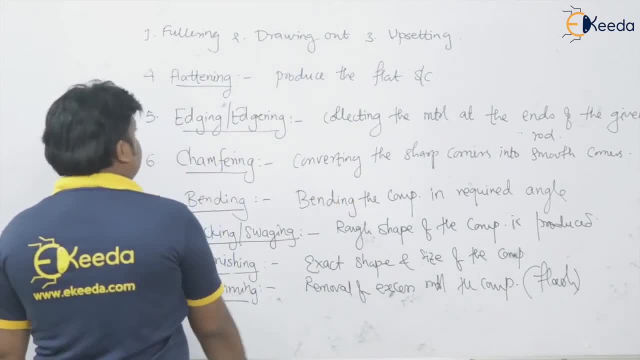 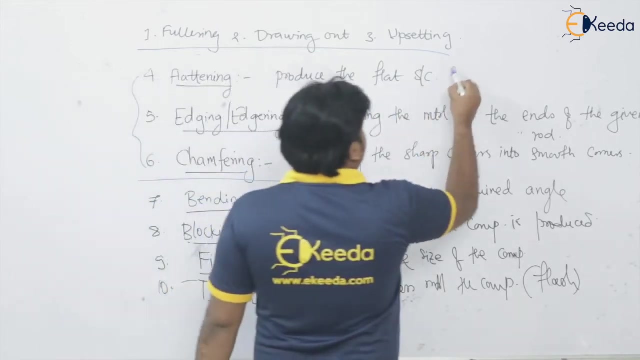 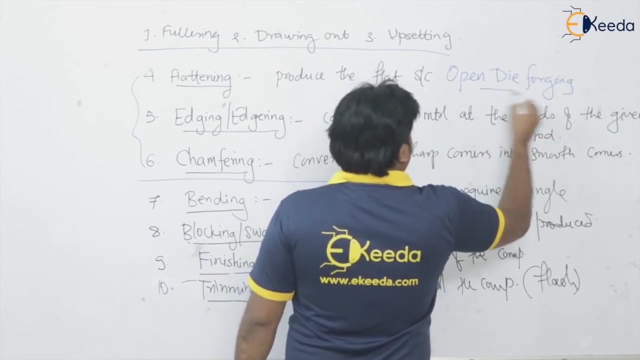 two, three, four, five, six, seven, eight, nine, ten. so see, if you look at this, first six operations, so these three operations and these three operation up to championing. so please remember, these three plus three or six operations are the open die forging operations, the open die forging operations. please remember this, okay, the 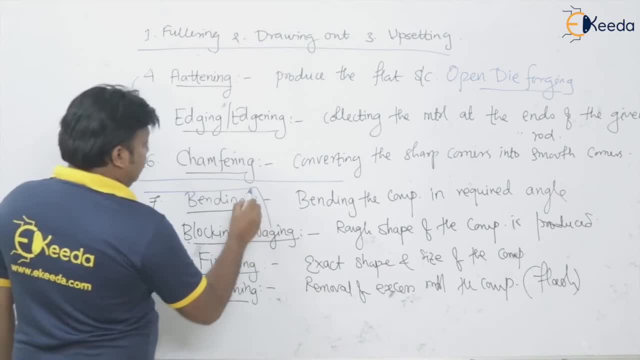 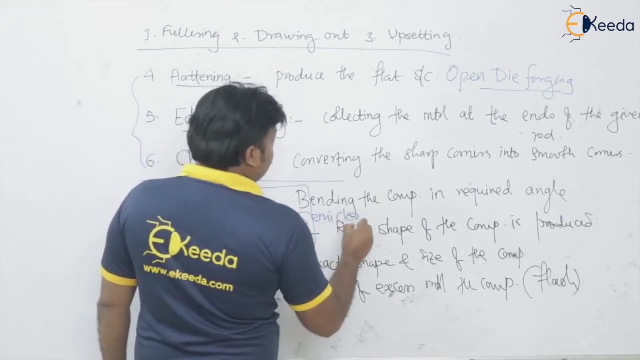 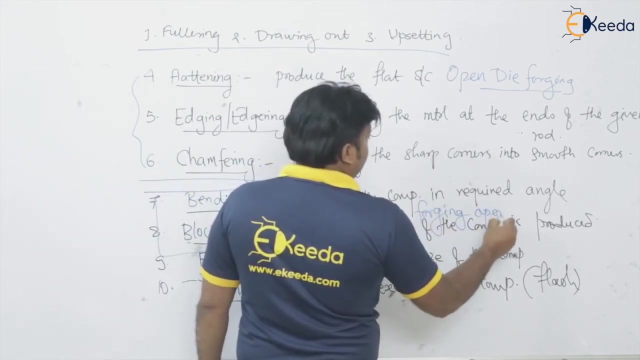 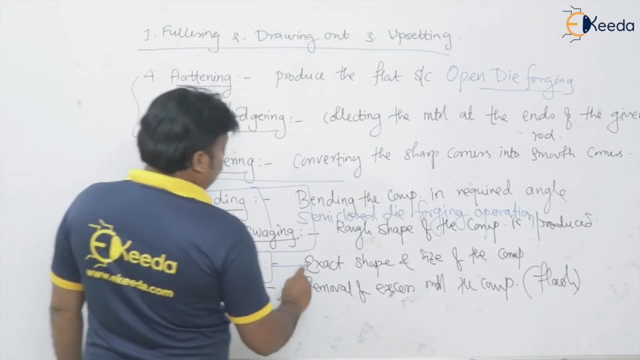 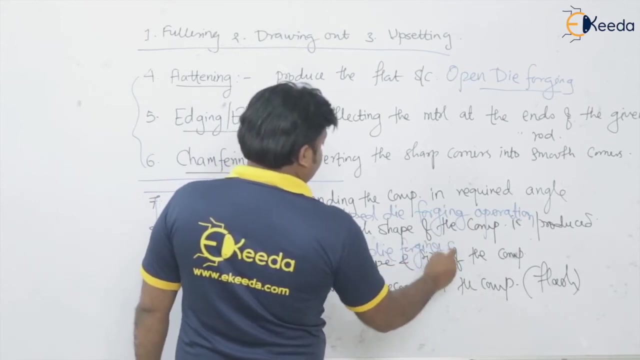 operation number seven and eight, that is, bending, a bending and blocking operation. these are semi closed. semi closed. die forging operation. die forging operation. please remember this. and finishing is pure closed. die forging operation closed. die forging operation. please remember very important and the trimming is what it is, nothing but the. 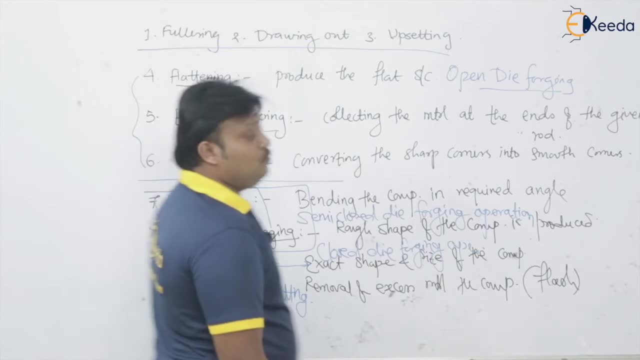 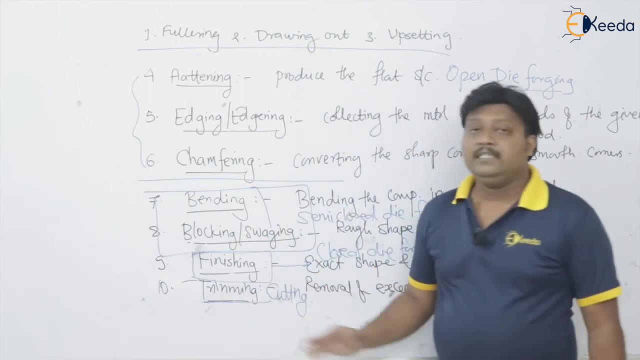 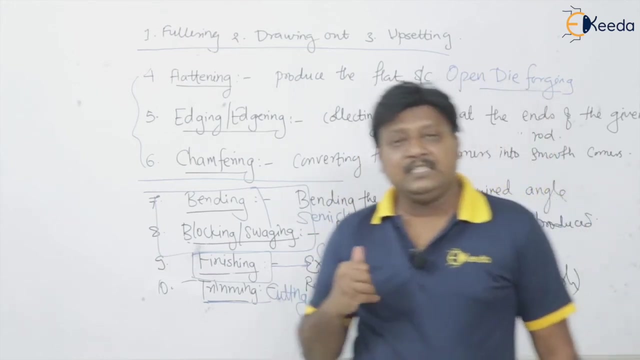 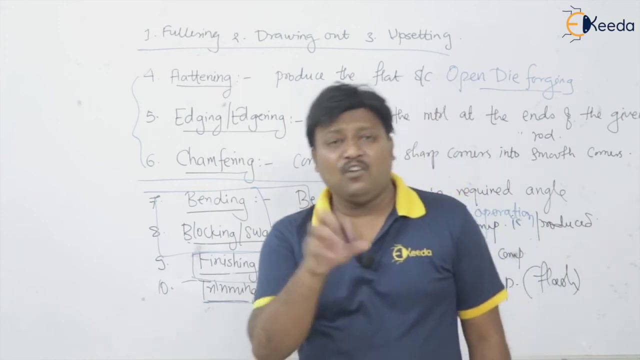 cutting operation. okay, so you should know the which are the open die forging operation, which are the semi closed die forging operation and which is the closed forging die operation. you should able to tell. okay, now see, by using this forging preliminary operations, if I ask you to made the connecting rod which is 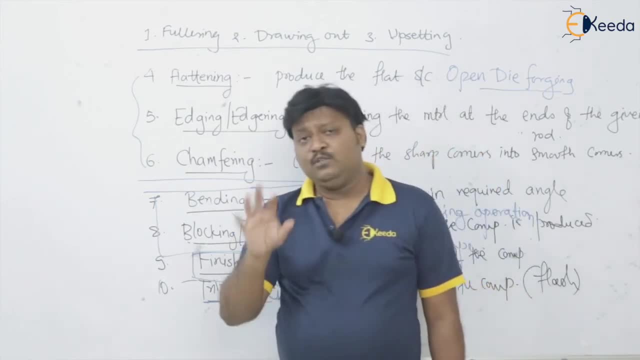 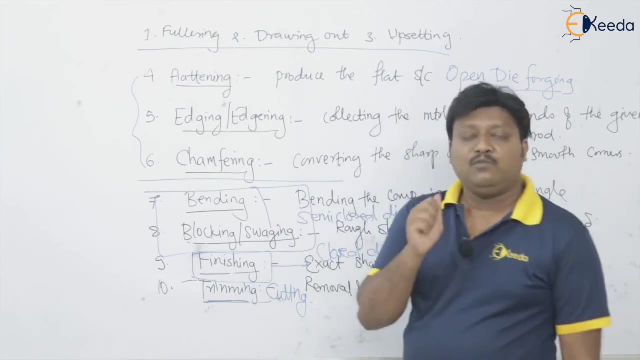 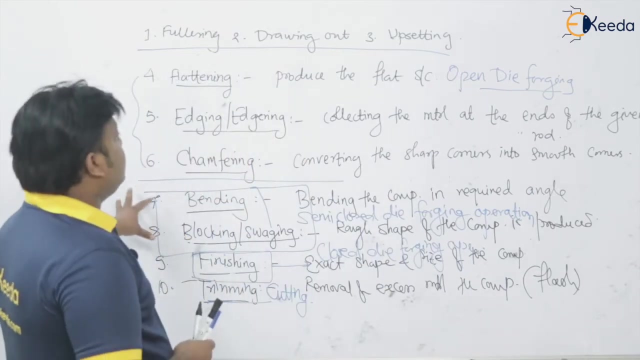 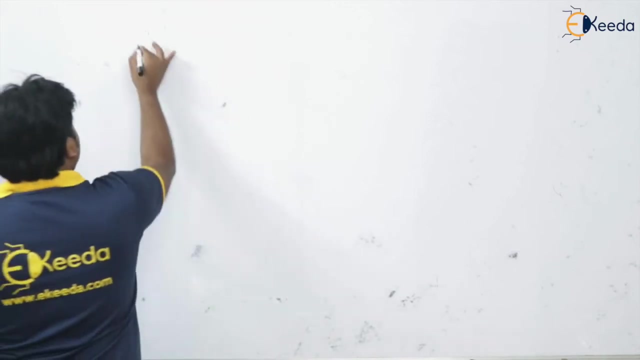 used in the rice engine. so connecting rod is basically used by or manufactured by. not used by, it is manufactured by the forging operations only, by forging technique only. so let us, by using some of the operations in that suppose, if I give you the question, like this, suppose, if I take the example of- to manufacture. 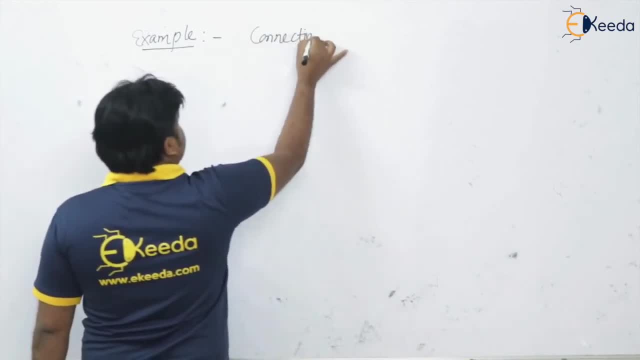 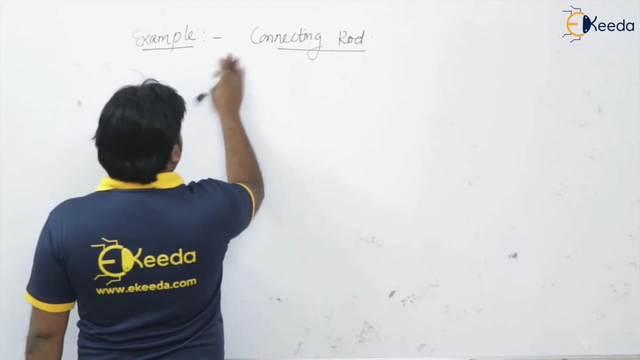 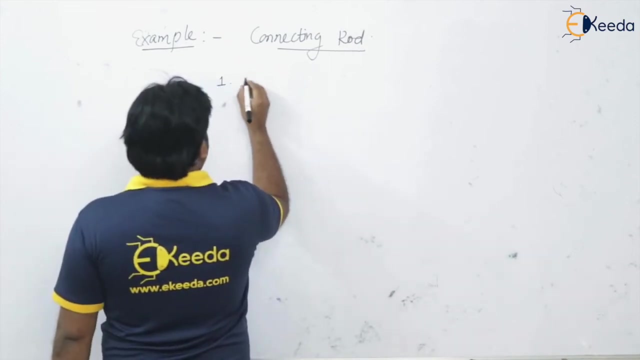 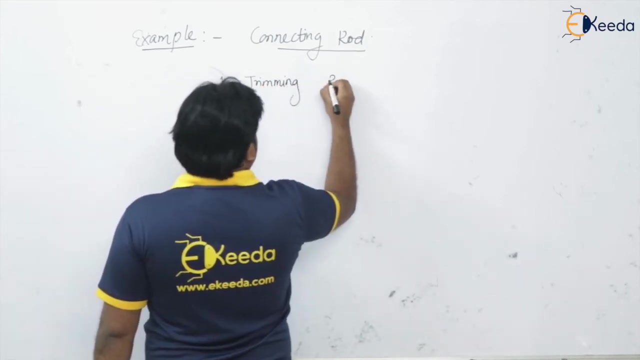 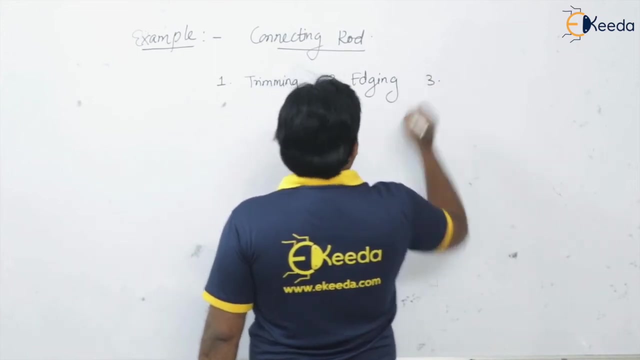 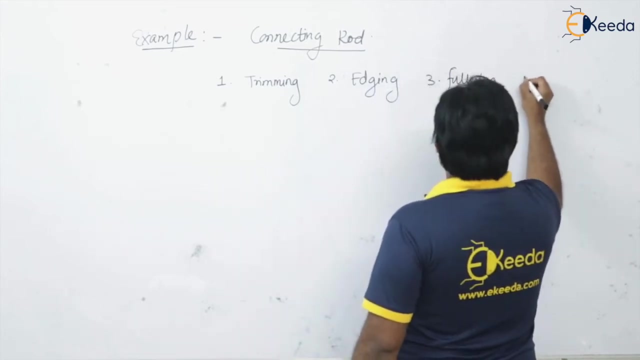 the connecting rod, okay, the connecting. so in the question suppose I, if I give you the various preliminary forging operations, like say one number, if I give you the trimming, the second number, if I give you the edging third number operation, if I give you fuller in fifth of fourth operation, if I give you the 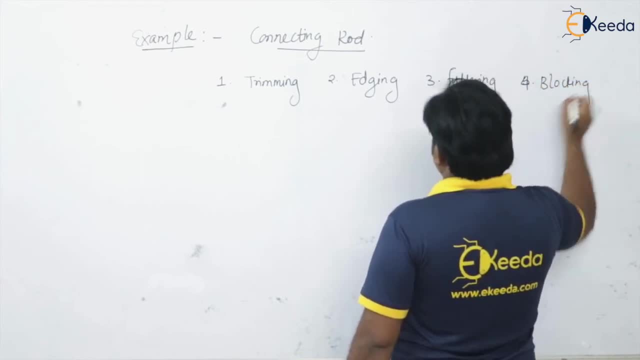 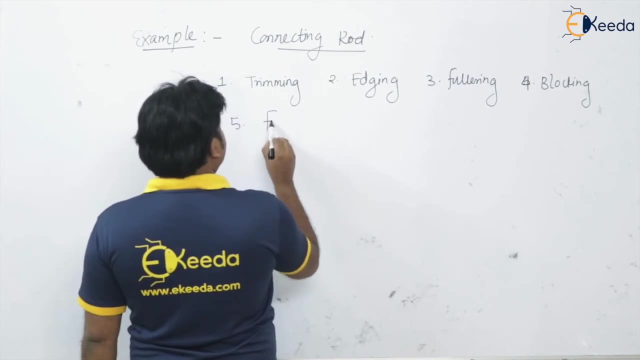 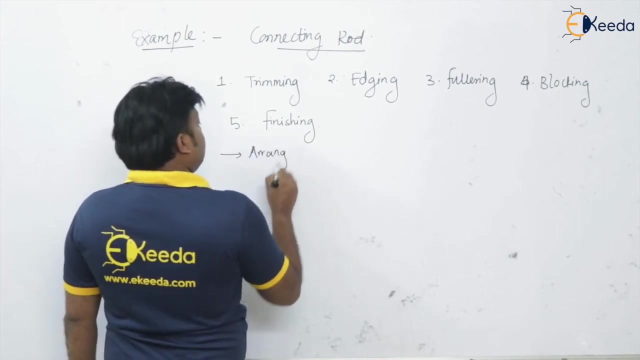 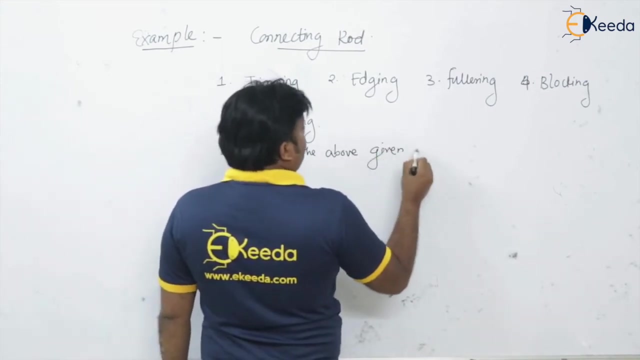 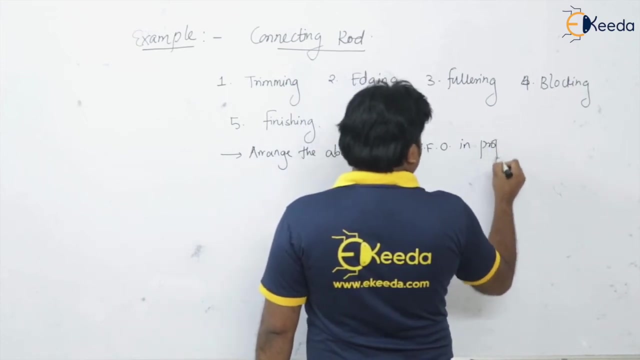 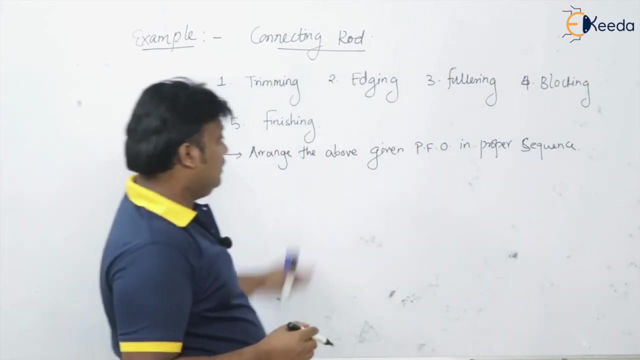 blocking. fifth operation, if I give you the finishing, so these are the operations. if I give you and ask you arrange the above given preliminary forging operations in proper or correct sequence- proper or correct sequence. and in the options, if I give you the various kind of sequence. so option ABCD, if I. 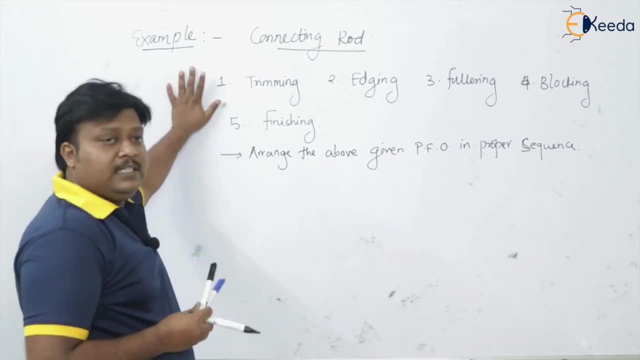 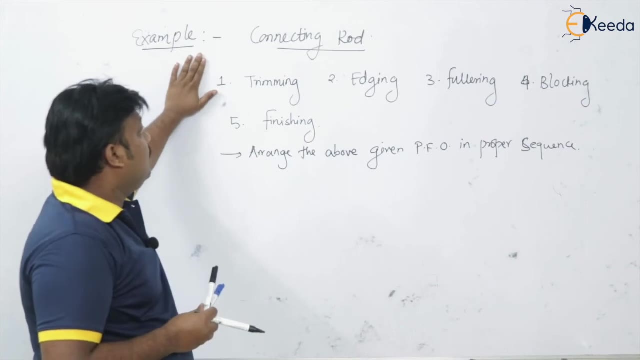 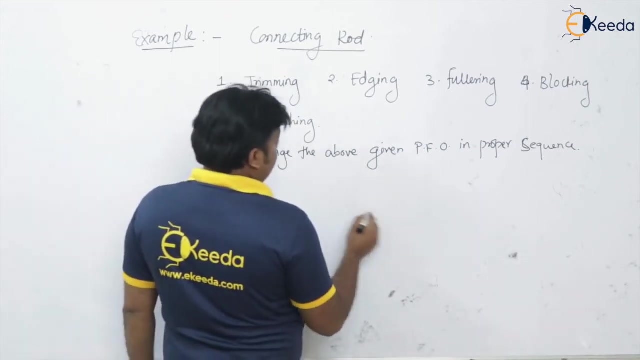 make, then this is a correct sequence. two more question, isn't it? so try to manufacture the connecting rod by using this preliminary forging operation that has been given to you. so, first of all, how the connecting rod look like. so it will be like this, isn't it? 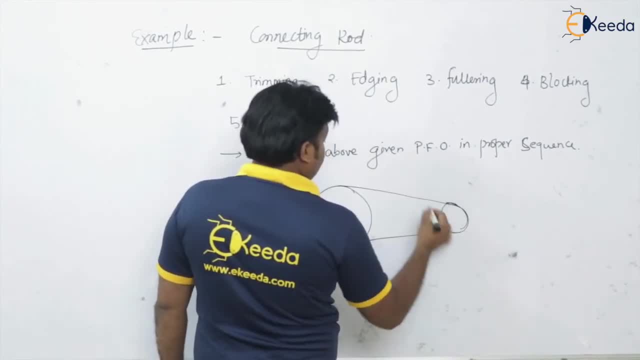 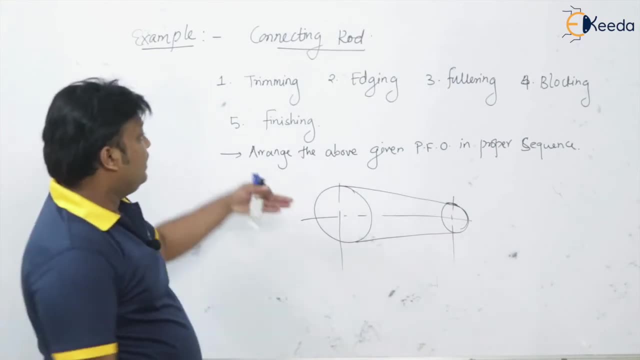 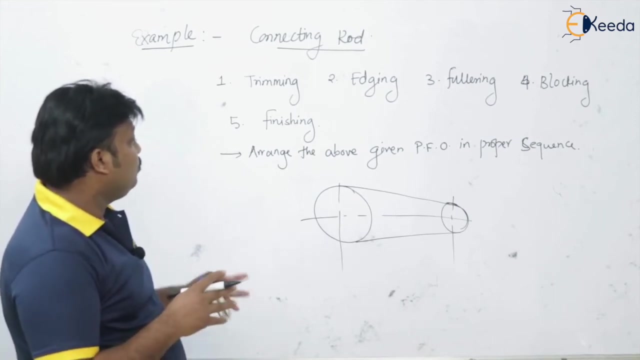 okay, so this is the connecting rod. okay, now, this one we are going to produce from a given rod. so which is the first operation that we have to use here? so i hope the first operation that we have to use that is the fullering operation. so for given rod, we have to distribute the material. 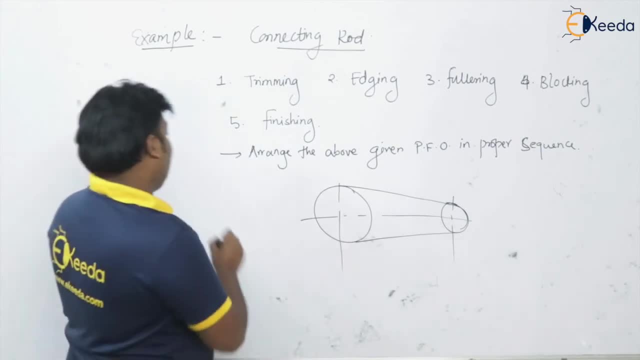 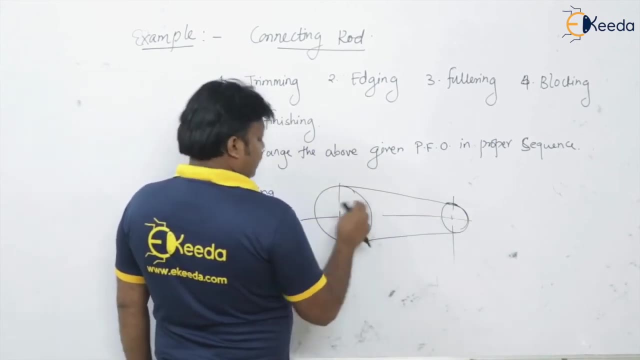 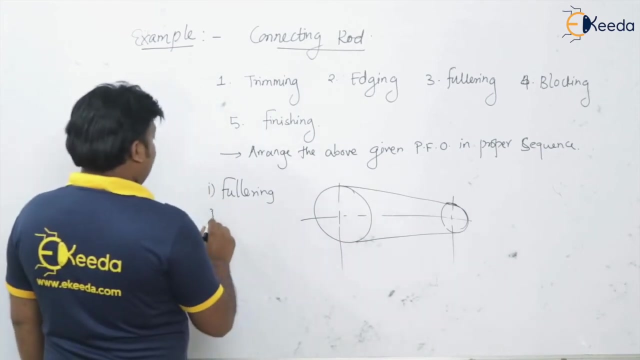 from center to the outward direction. so i will go for first the fullering, then here see the ends of these two, of these rod. two ends are not same. we have to provide the necessary material at the ends. so after fullering i will go for the edgering operation or edging operation, once i got. 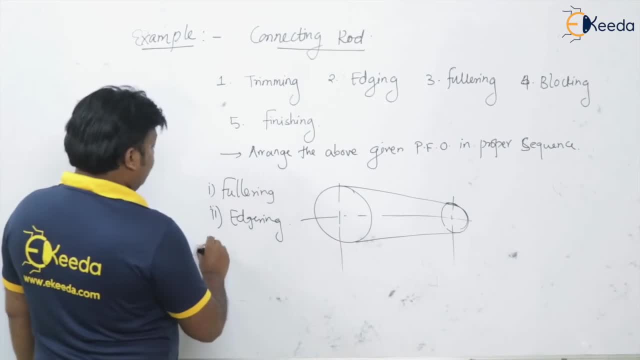 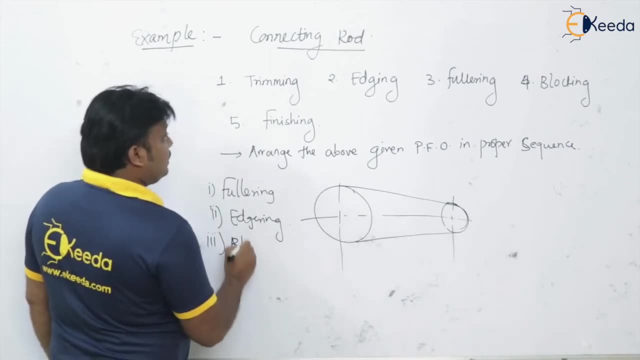 the sufficient material at the ends, i can go for the approximate shape, that is, rough shape. for producing rough shape, i will move on. that is the blocking operation. given it's yes, and of course you know blocking is okay. okay, so we are going to make the connecting rod, and the connecting rod is always followed by. 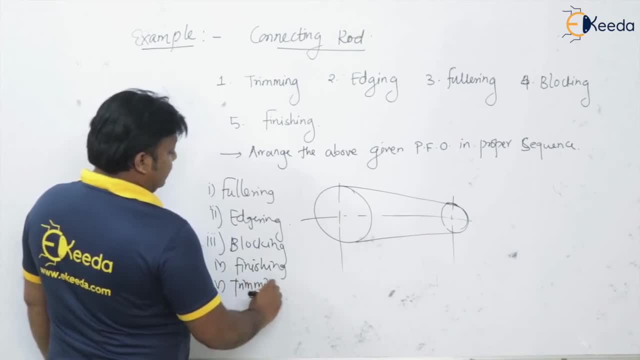 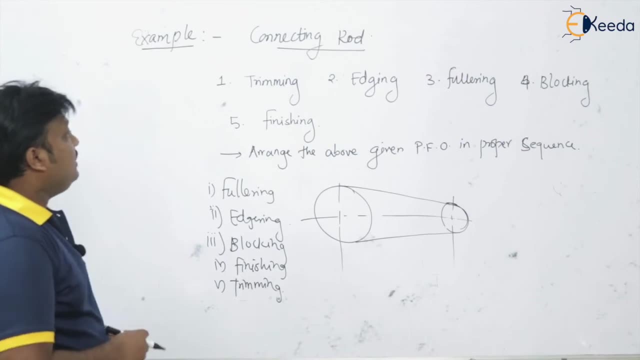 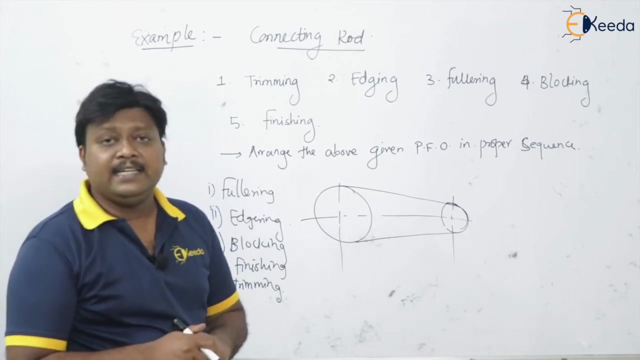 the finishing, and finishing is followed by trimming. so in that way, i can able to make the connecting rod from a given cylindrical rod, isn't it? so now, if i ask you to manufacture the head of the hexagonal bolt, okay, the head of the hexagonal bolt. if i ask you to, 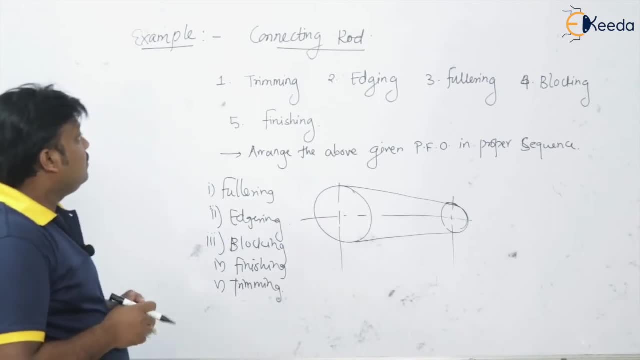 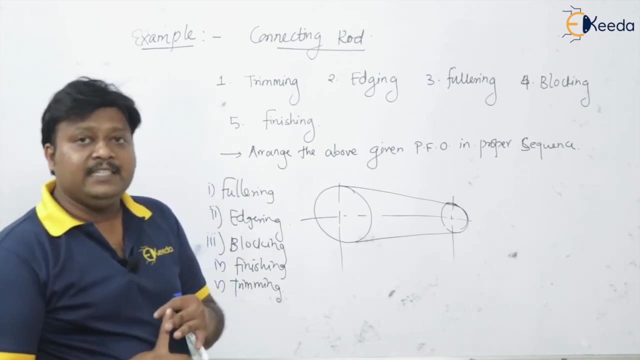 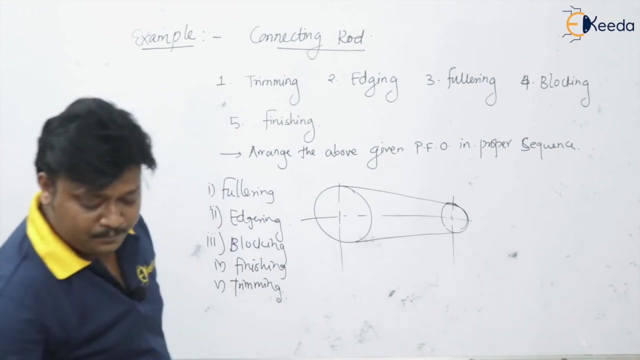 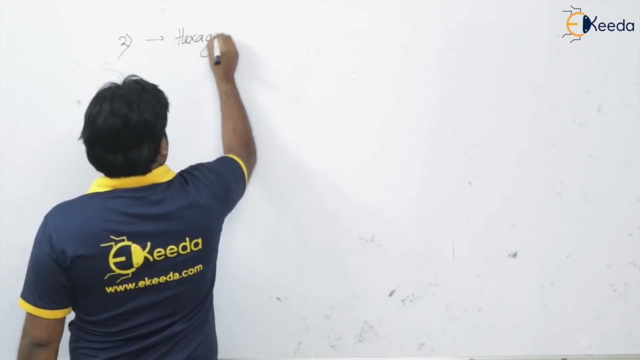 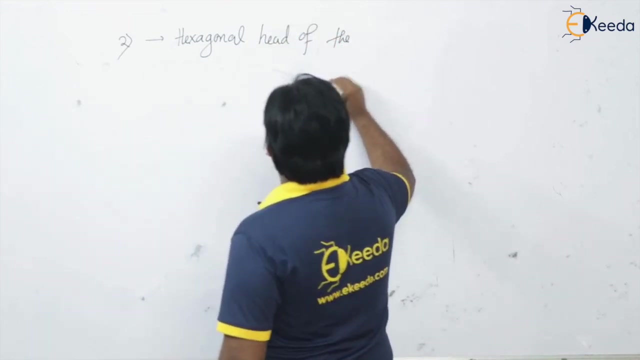 make by these forging operations, giving you the operations like blocking, say, chamfering, upsetting and trimming. okay, so which are the operations I am giving you? say, for next example, that you are going to make the hexagonal head of the head of hexagonal bolt head of the 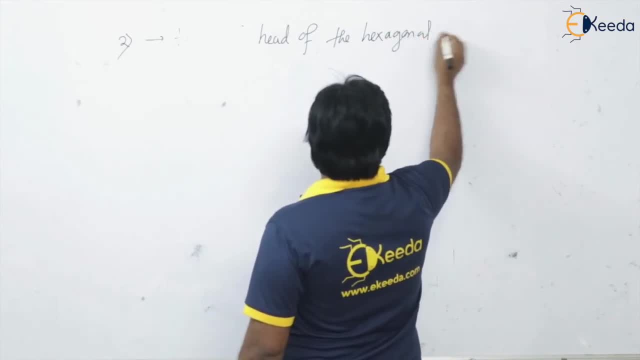 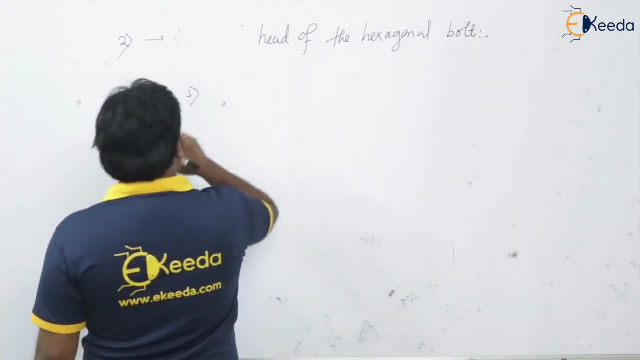 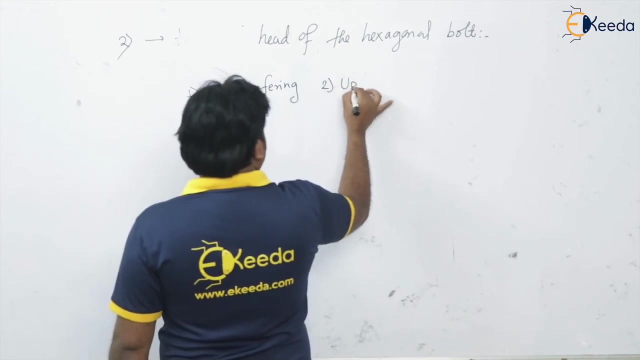 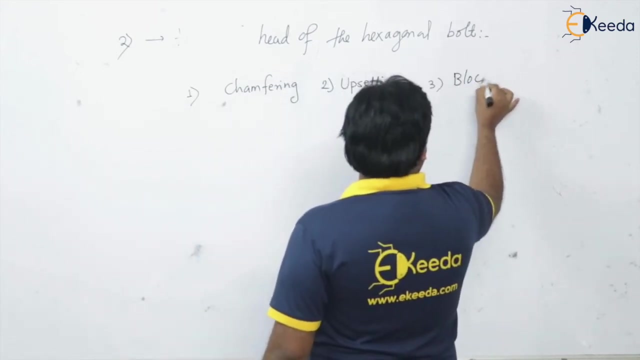 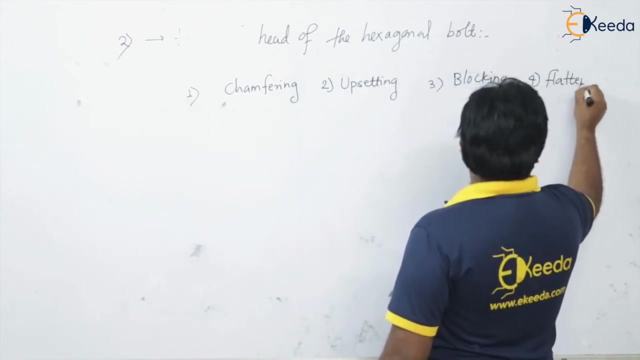 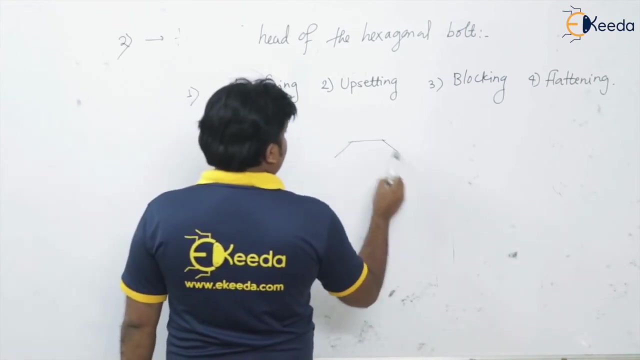 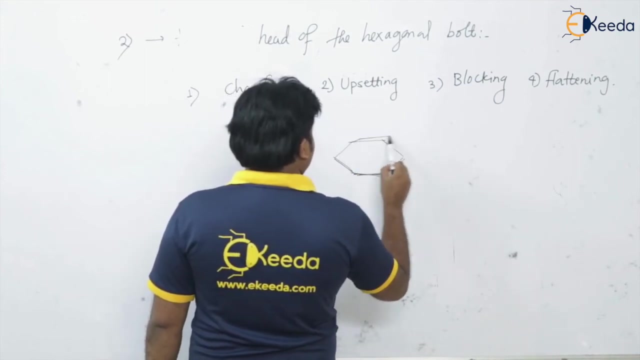 hexagonal bolt. okay, now the process I have been giving to you, that is, chamfering, upsetting, then blocking and say flattening. so we have to make the head of hexagonal bolt. definitely, that will look like this, isn't it? you have to made it, Master. 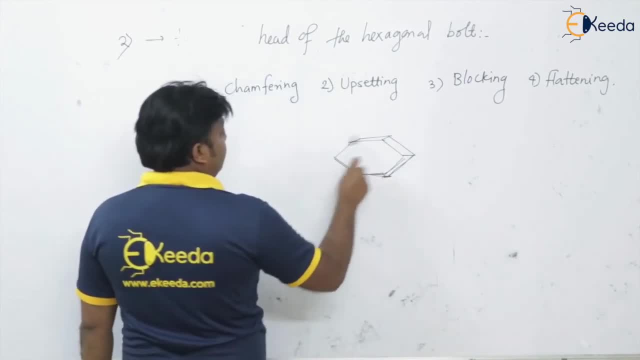 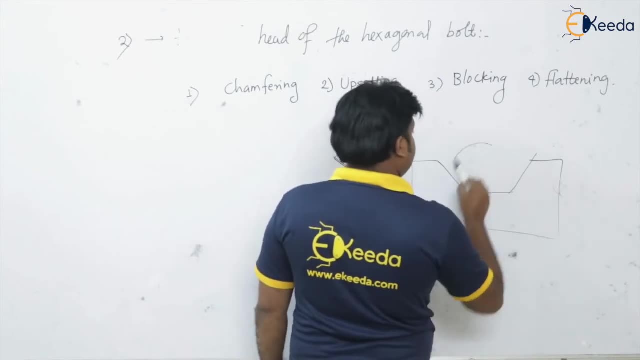 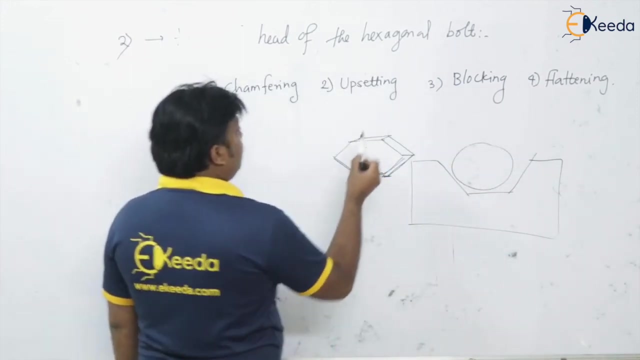 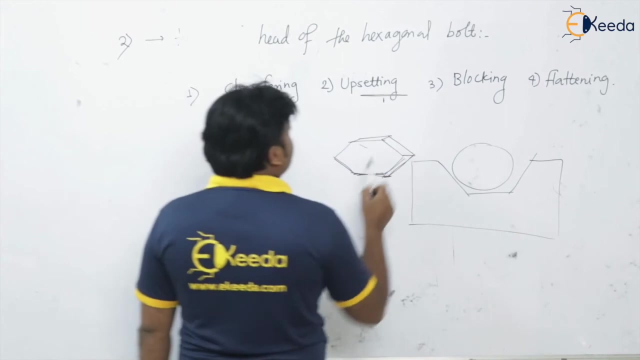 okay, hey, this is a head, actually hexagonal head. so definitely, if you are having this material, you put in the die. okay, so you upset it first of all. what we'll do. you are going for the upsetting, isn't it? then you are going for, after upsetting, will go for flattening, isn't it? first of all, we will. 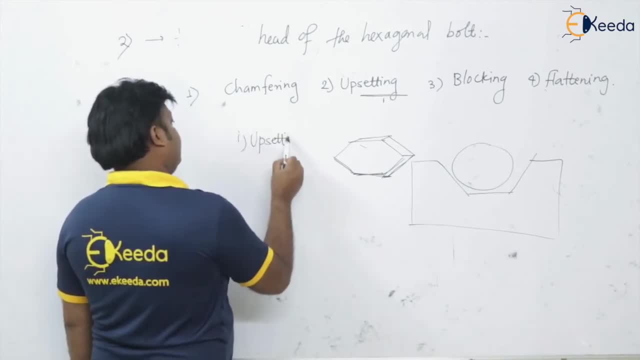 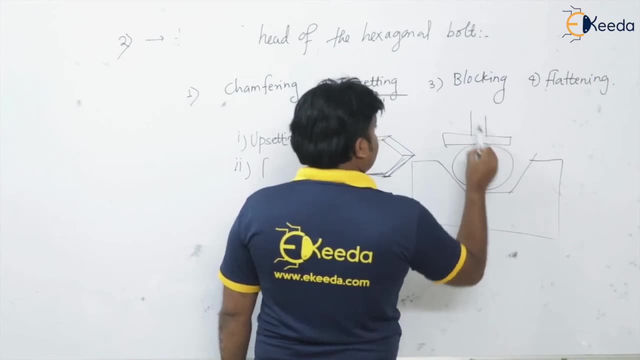 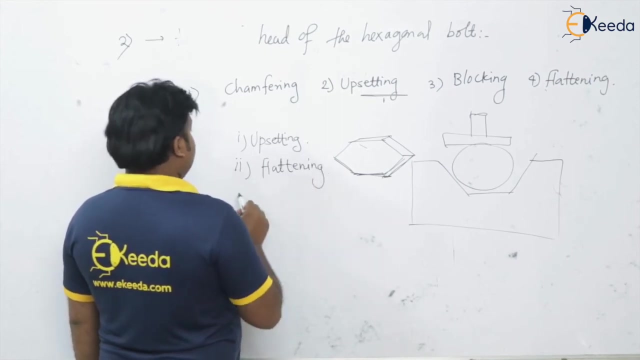 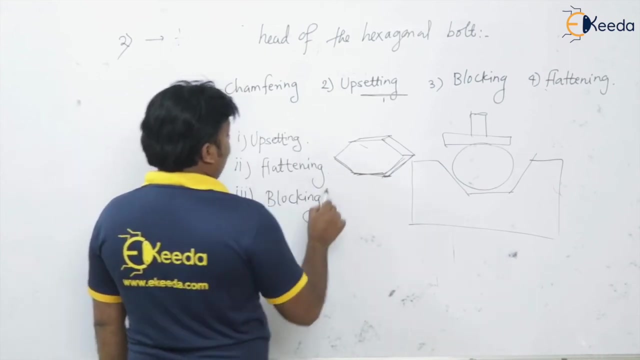 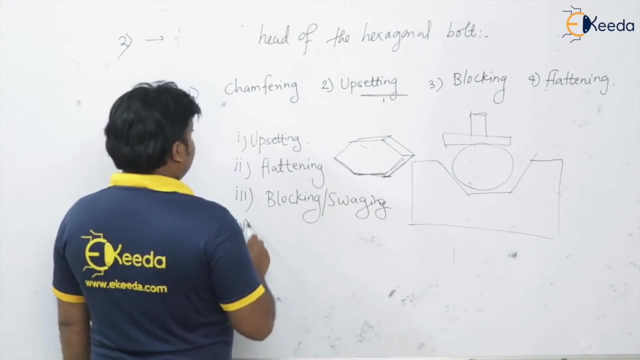 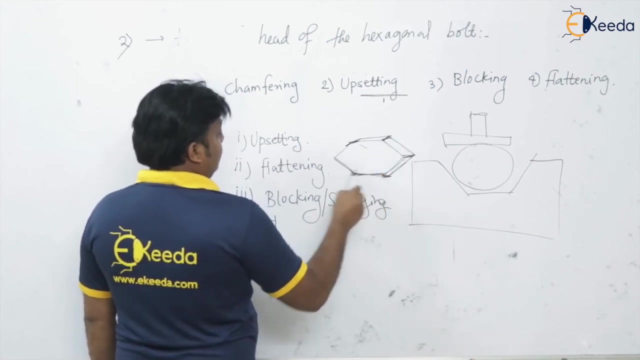 go for upsetting, then we'll go for flattening, isn't it? by the flat dies flattening. then we will go for the approximate shape or swagging operation. here we generally go for: block your swagging, okay. and last one will go for the chamfering of the edges here. okay, this edges are going to get chamfer. 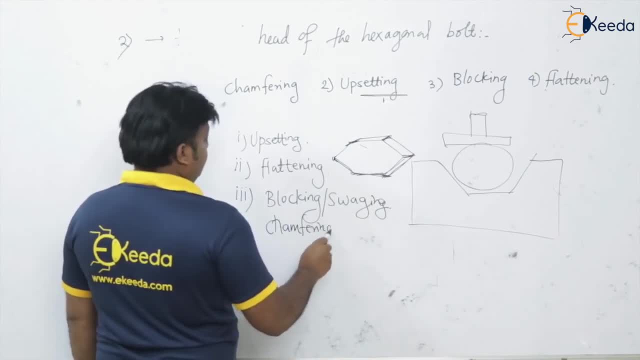 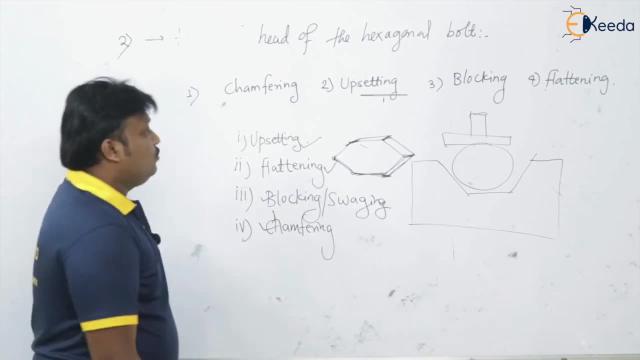 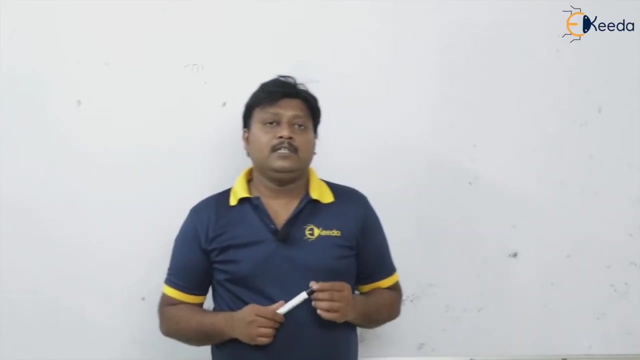 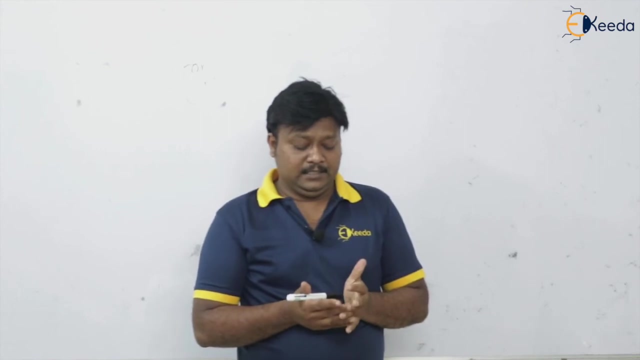 chamfering. so correct sequence will be first upsetting, then flattening, blocking and chamfering. so this is how we can able to made the given component by using this preliminary forging operations. now here we are going to see the next topic, that is, the forge ability. so forge ability means what actually the 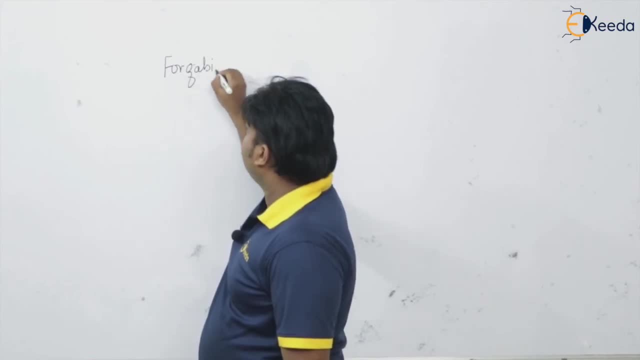 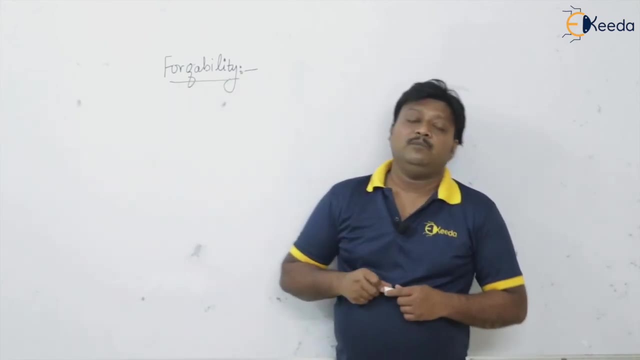 for shabby it understand. so what is mean by forge ability? the definition of forge ability says it is the ability of the given component for the forging or the ability of the component to get forged with a little amount of force. what is forge ability? the ability of the given component to forced to get forged. 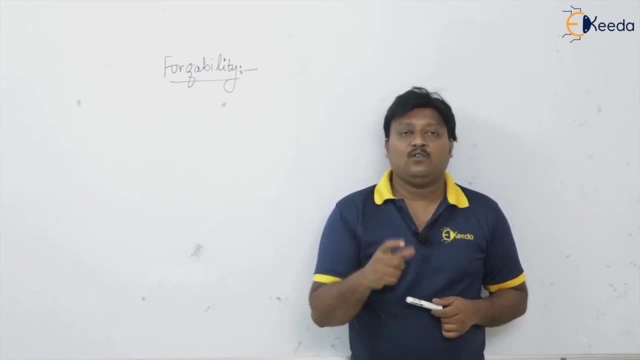 with the small or giving amount of force. so we use the only oneаемig cathode to get to theude with the small or little amount of force. if it is念, amount of force is called as the forge ability or the ease with which the 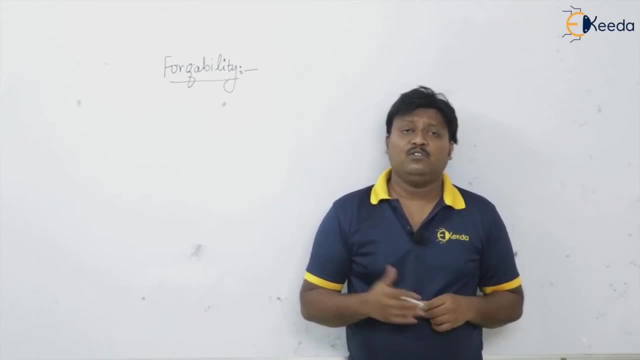 forging can be done on the component, that is, with, of course, the little amount of force. it is the forge ability. now, what is the forge ability of various materials that we are using in day-to-day life for the forging operation, or the materials which are subjected for the forging operation? 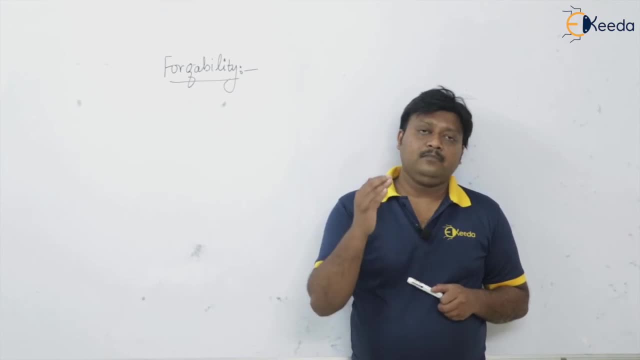 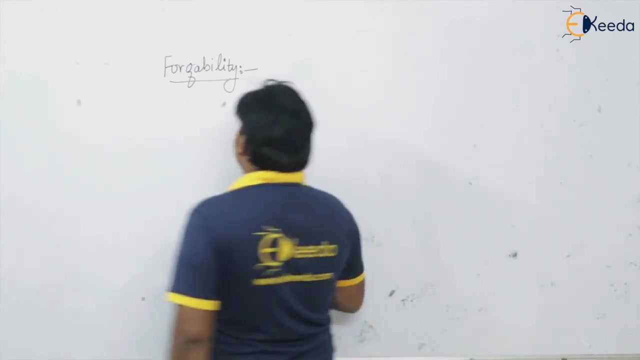 we are going to see the ability of these materials. which material can we get easily force or which material is very poor for forging operation. that thing we are going to see. so I am going to write here the various materials with decreasing order of their forge ability. okay, so subsepa LA. the material is 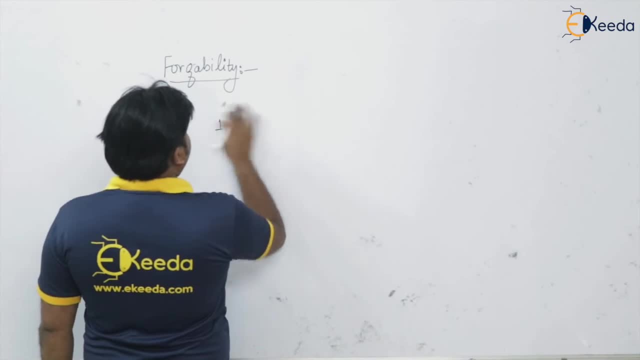 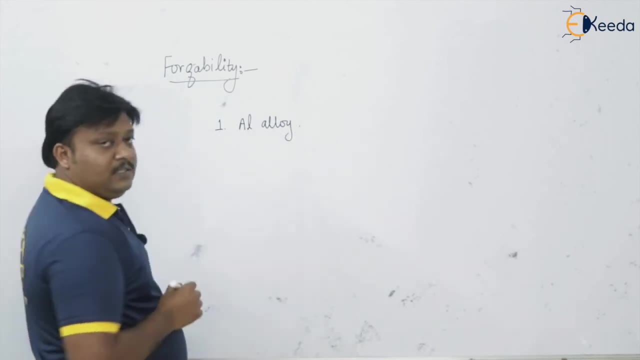 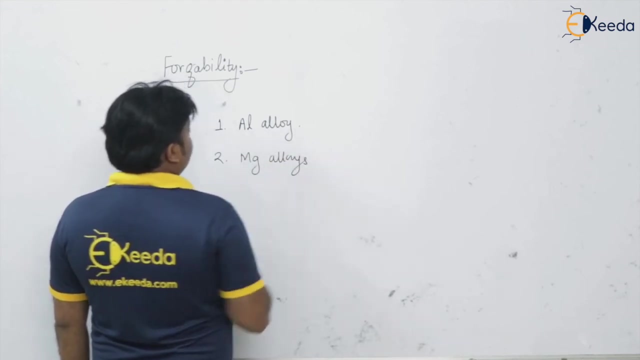 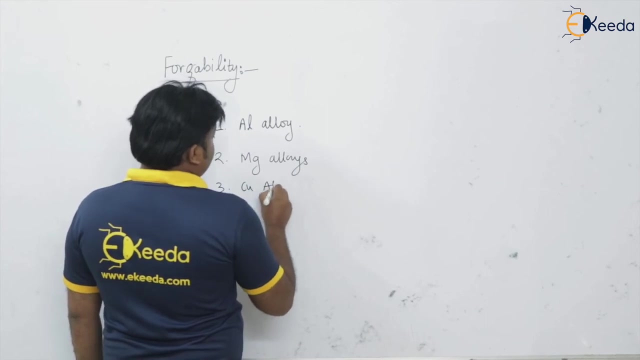 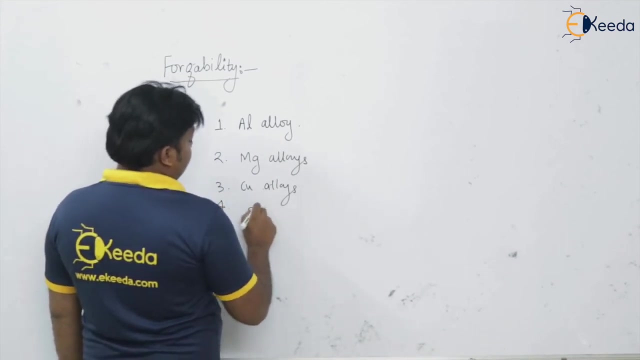 having very good for job. it is the aluminum alloy, which the aluminum alloys. then we are having magnesium alloys. after aluminum, the magnesium is very good for the forging operation. third, we are having copper alloys. third, we are having the copper alloys. fourth, we are having the steel as a good forging ability. 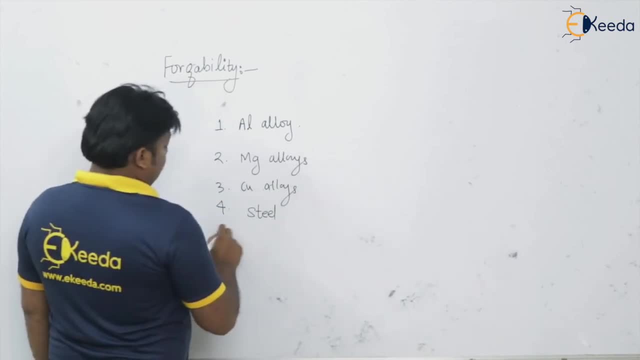 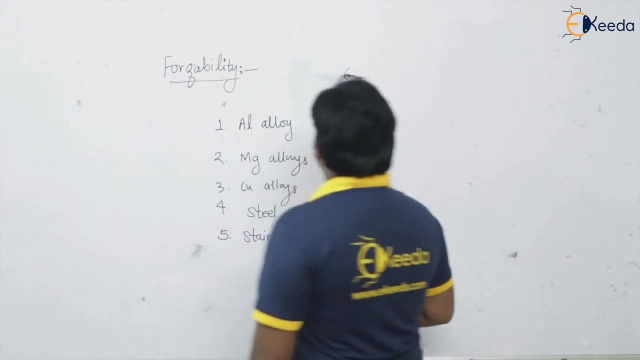 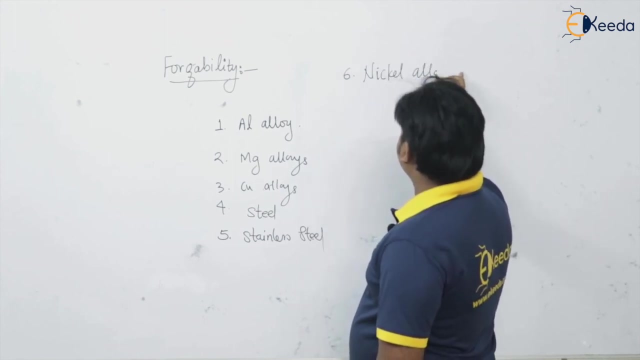 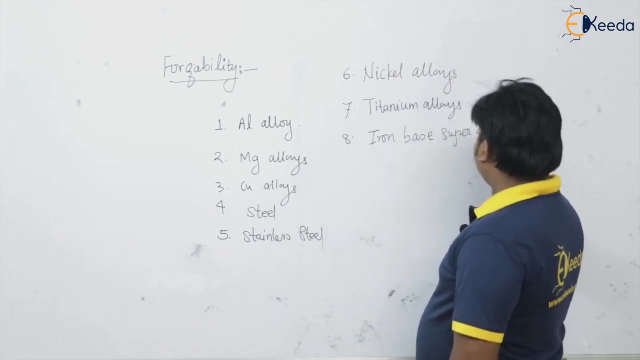 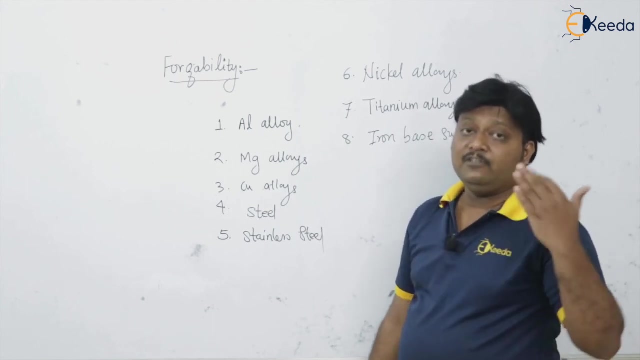 I believe it is steel. after still, we are having the stainless steel. okay, then we are high having the nickel alloys. after nickel alloys, we are having titanium alloys, then we are having iron based super alloys. super allow means these are the newly developed material having its very good properties at higher or elevated temperature. they are not. 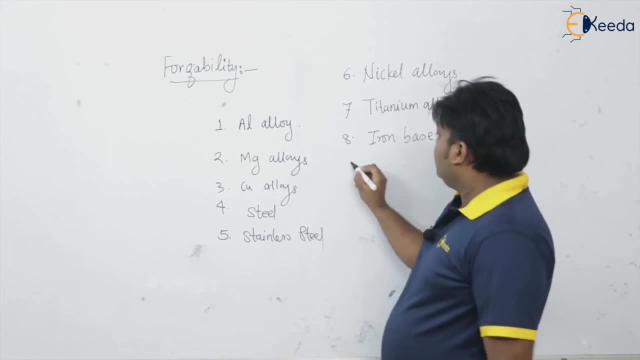 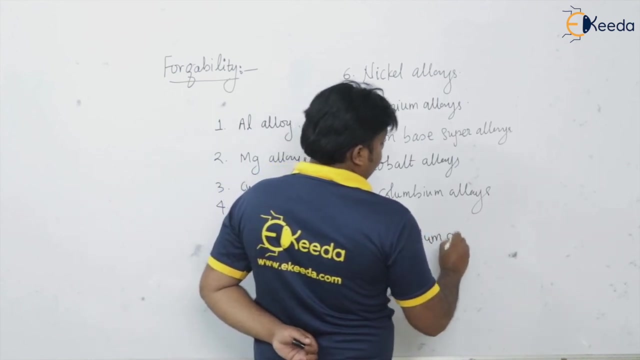 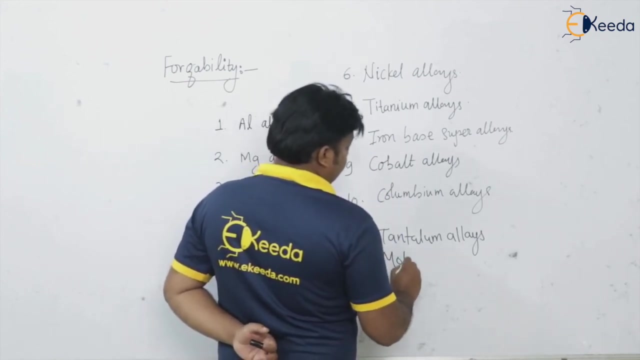 going to lose the properties. these are the super alloys. then we are having the cobalt alloys. then we are having the columbium at 11 number. we are having tantalum alloys, tantalum alloys- 12 number. we are having molybdenum, molybdenum alloys. 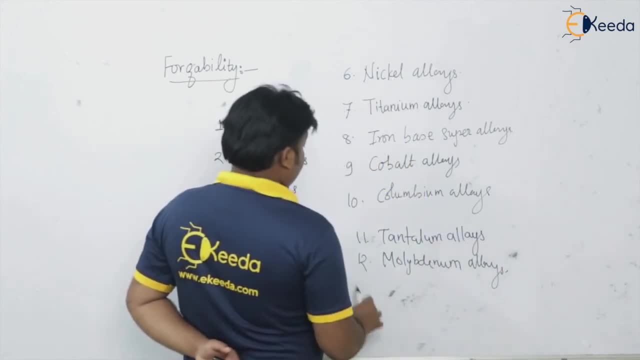 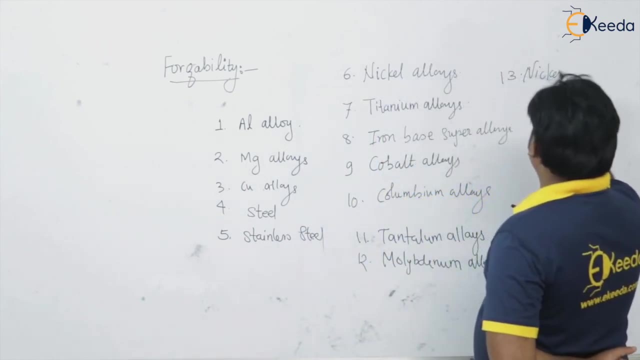 13. then we are having nickel-base super alloys. nickel-base super Aloys- number 14. we Dee Sway- very poor, That's sounding pretty amazing. Gods alloys who are having the�� best alloys alloys. one last thing: we are having nickel base super. it is a nice banco muscle. 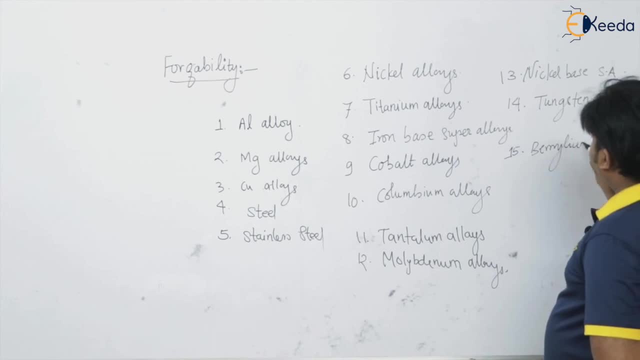 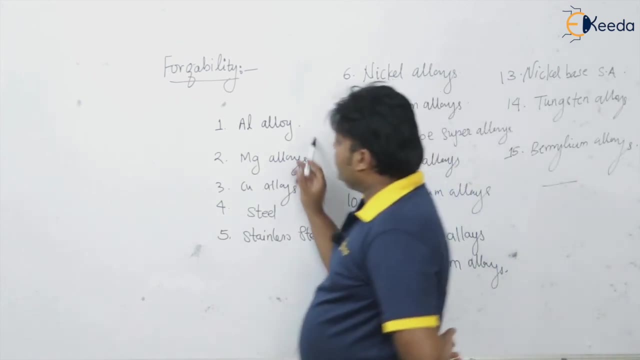 alloys, nickel base, super alloys, nickel base liquid alloys. second is we are having the breve oyster withży. no single aluminum alloy and decline Aloys, heavily virtue alloys, and that's beryllium alloy, beryllium alloys, so you can see here the aluminum, magnesium and copper. 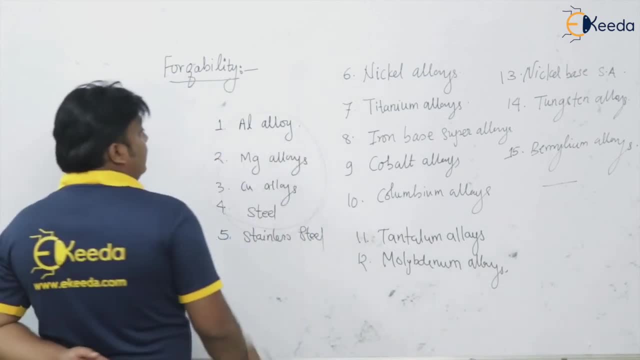 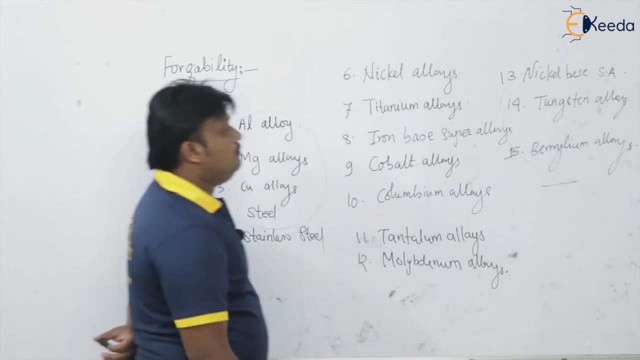 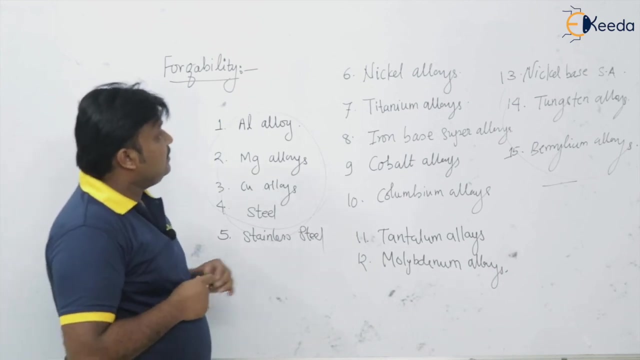 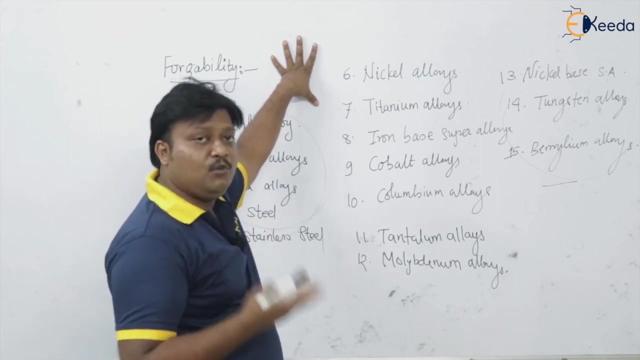 these are very having very good forgeability and if you talk about the very worst or poor forgeability, we are having the tungsten and beryllium alloys. okay so aluminum, magnesium, copper steel, stainless steel, nickel alloys, titanium alloys, iron base alloys, cobalt alloys, columbium alloys, tantalum alloys, moly. we are having nickel base alloys. we can be super alloys.